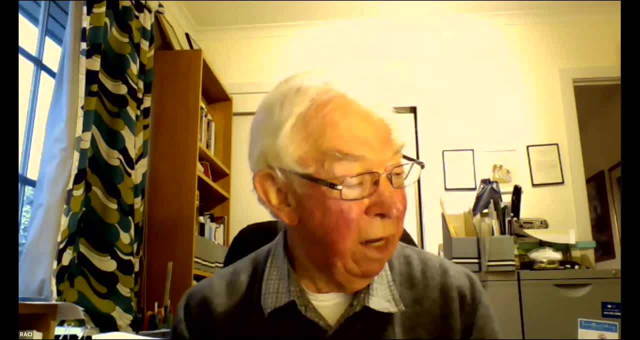 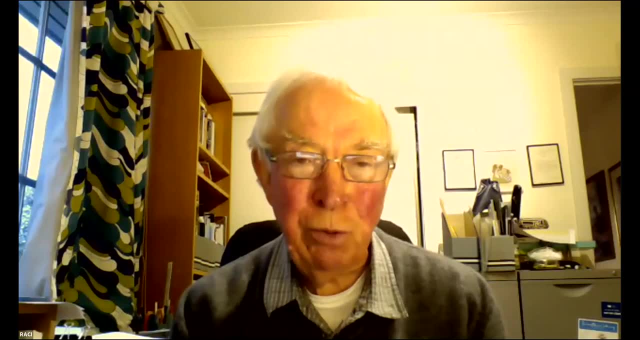 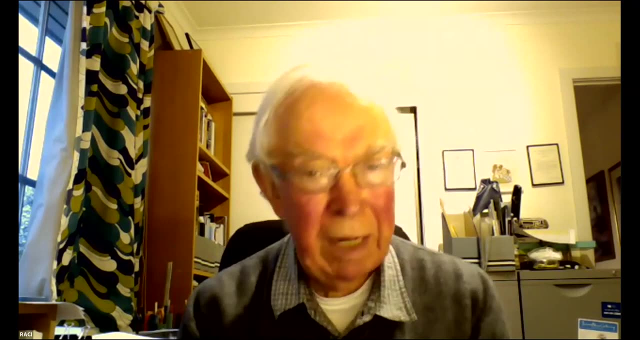 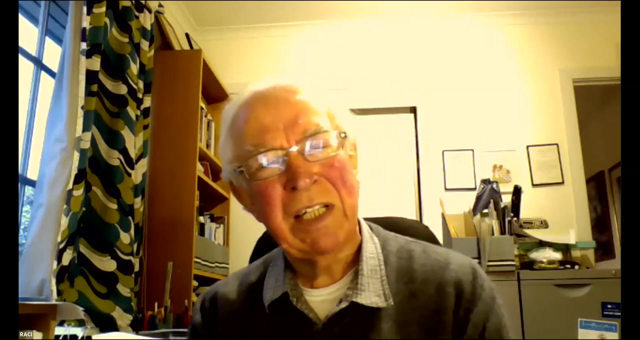 coming and for attending this historic occasion. It's the. as far as I'm aware, it's the first Zoom meeting of the Health Safety and Environment Group of the Victorian branch. So welcome everyone, particularly welcome to people from interstate. Do we have anyone from overseas, Elise? 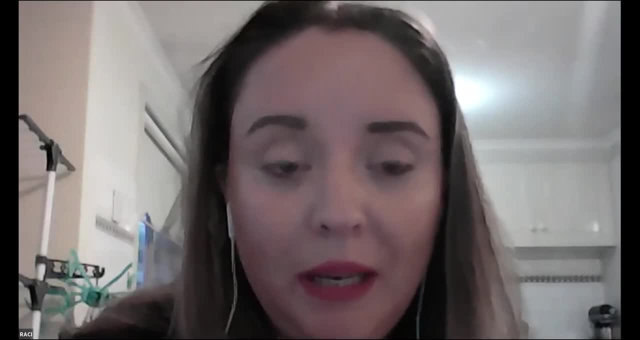 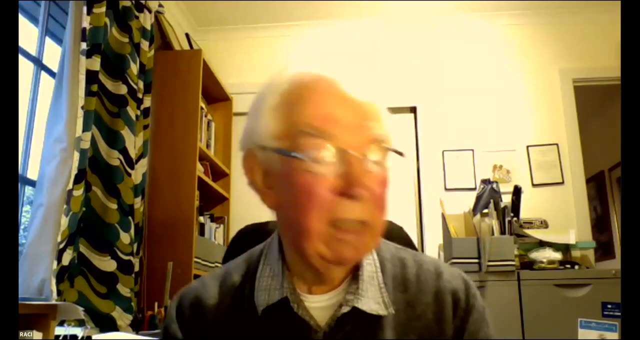 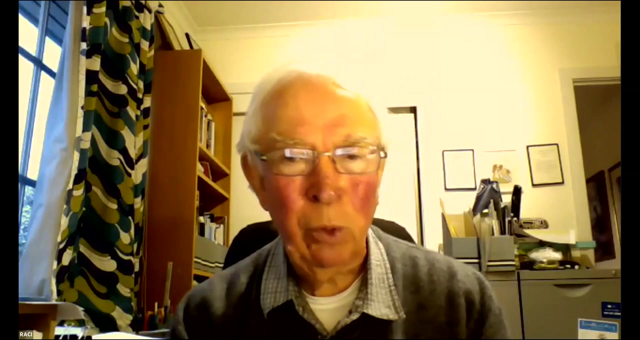 Not that I noticed on the registration list, but we definitely have interstate, Interstate people. Well, that's excellent. So thank you for coming, And I'd particularly like to say thank you to Elise for setting us up and for getting us all- well, all the technology- working Now, Elise, I think. 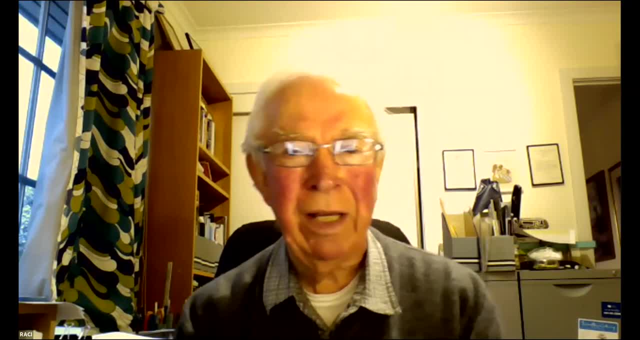 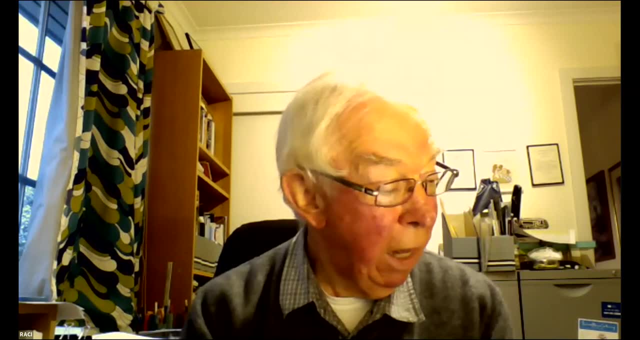 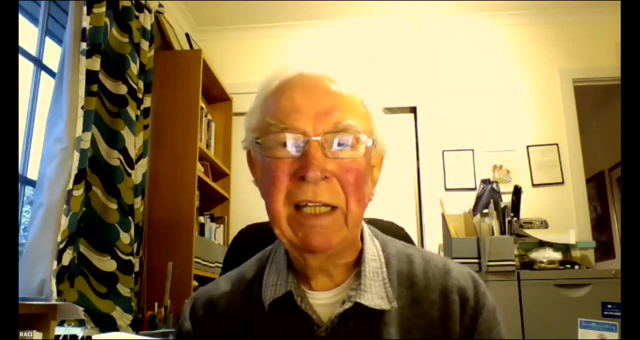 may have to leave us before the end of the meeting, but thank you, Elise, anyway, for all that you've done so far. Now, what I was going to do at this stage was to introduce Dr Ian Thomas, who is the chair of the Health, Safety and Environment Group. 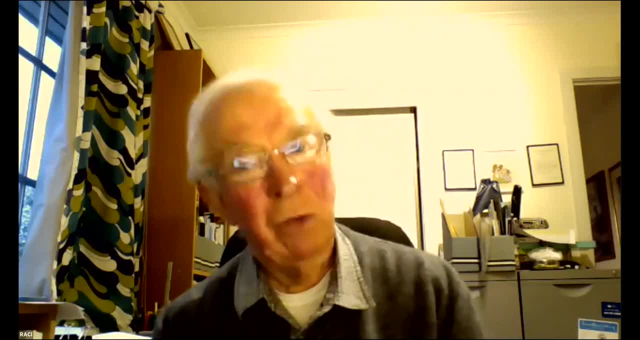 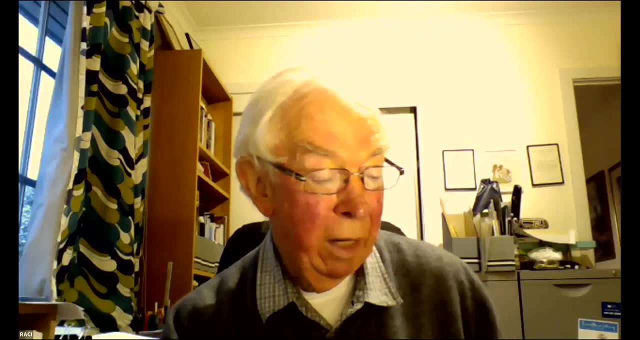 And he's the director of the Health, Safety and Environment Group of the Victorian branch. but Ian has- or Ian's wife, Joan, has just called in to say that Ian isn't well at the moment. So I will keep that He will join us later if he's able, And I think Joan may join us. 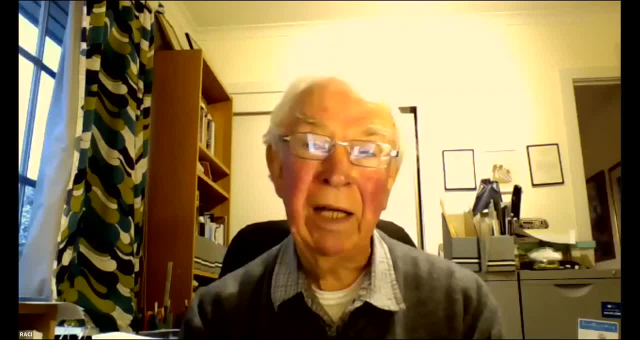 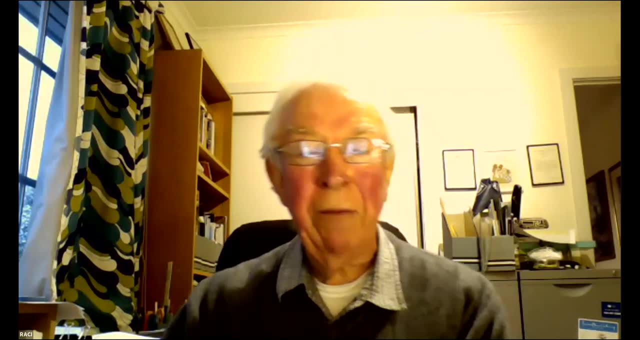 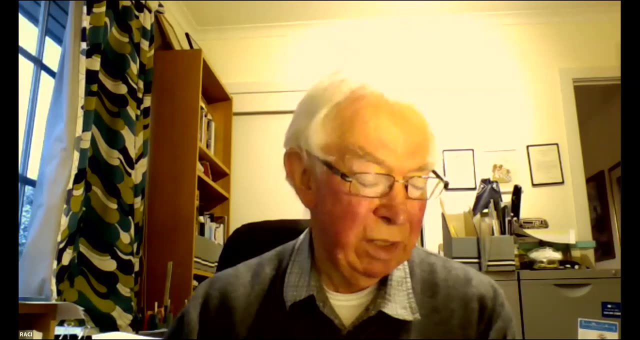 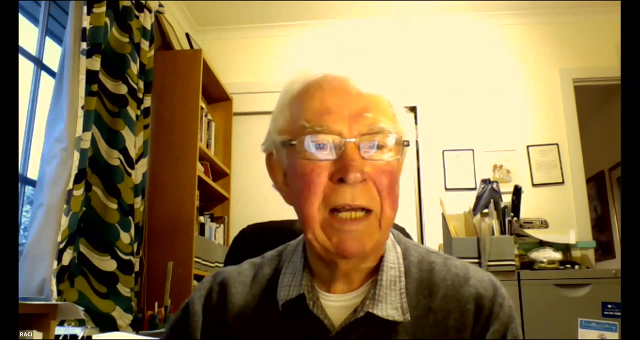 during the course of the evening, But disappointed that Ian can't make us and that Lisa has just given us an apology for Neil Jackson. Now I'd like to briefly introduce Susie and her students, who are going to make the presentations this evening. As far as housekeeping is concerned, what would be good is if you could. 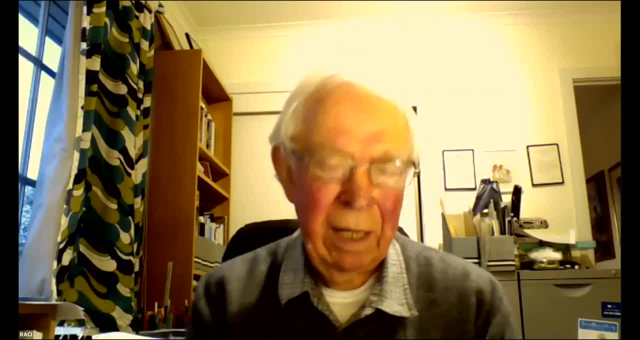 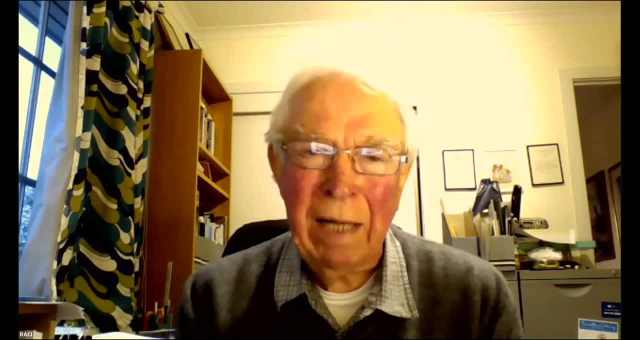 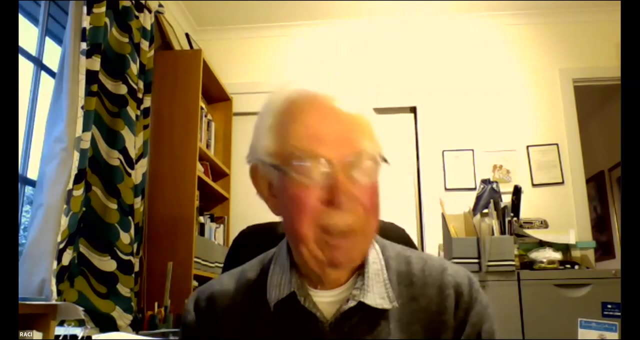 please mute your computer so that speakers have an opportunity of speaking in a sort of undisturbed manner. If you don't mute your computer, I can do that. That's kind of the thing In a sort of a position of authority here, but certainly as a 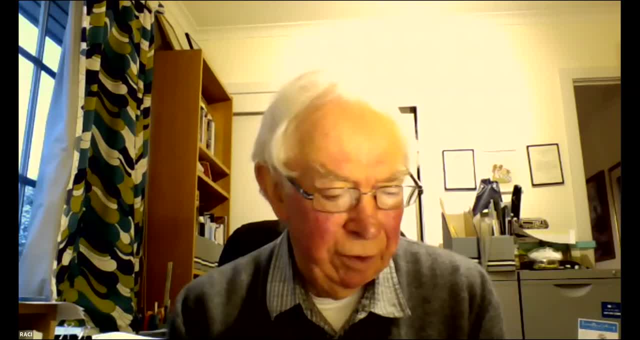 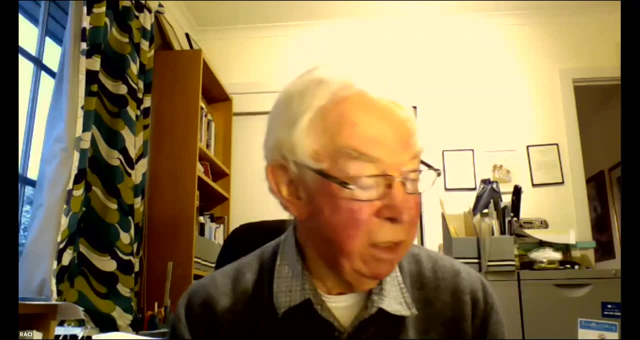 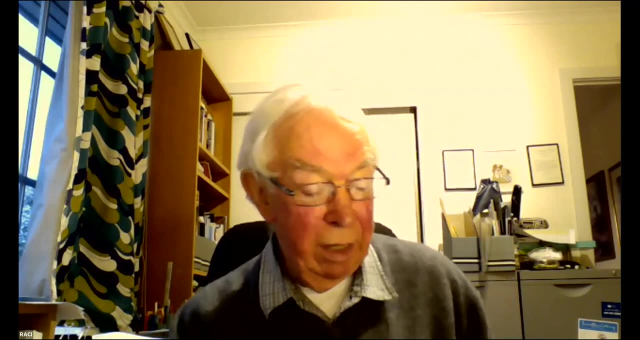 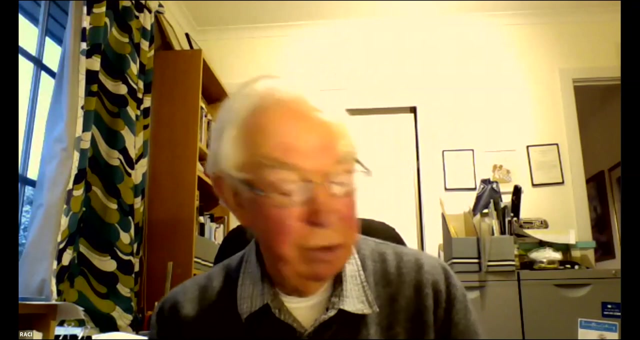 courtesy to our speakers. please turn your microphones off whilst presentations are being made. Now, what's going to happen this evening is that I'll formally introduce our three speakers, or formally introduce Associate Professor Susie Reichman, who will, in turn, introduce her two students who will be here with us, who are here with us. 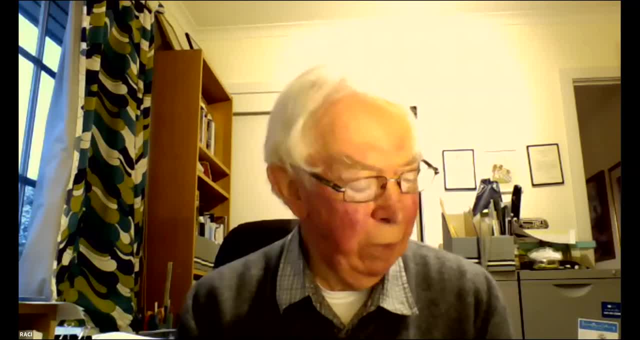 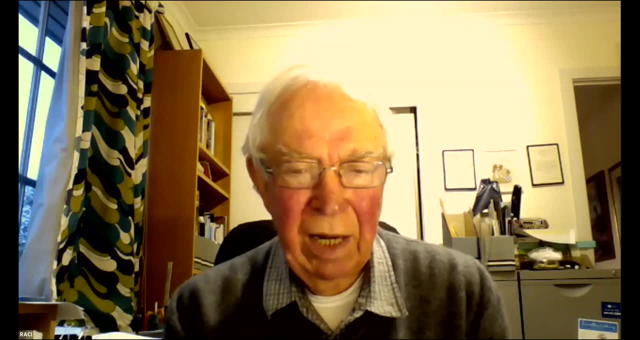 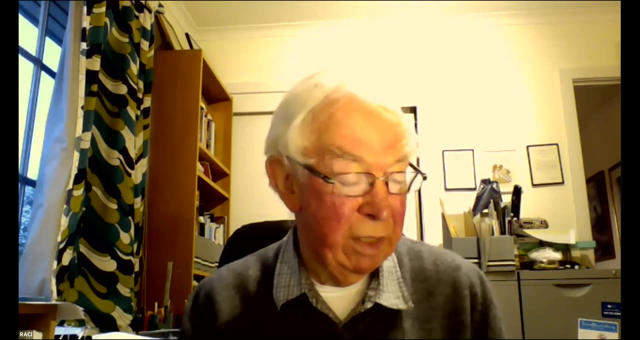 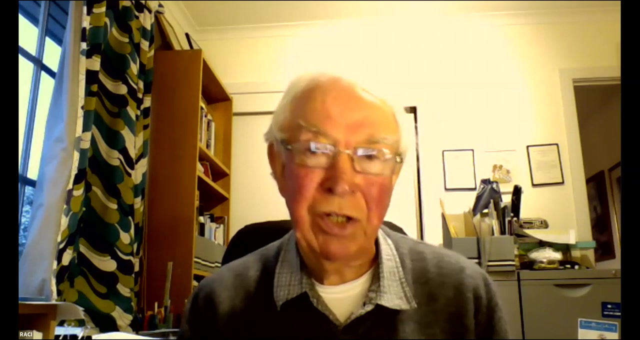 Justin Morrissey and Zhuwen Gu. Ian was going to chair the question and answer session after the presentations. I think we'll save all the questions and comments till the end of the presentations, but if Ian isn't here then I'll look after that, And the object is to keep the meeting until probably about. well, we'll see. 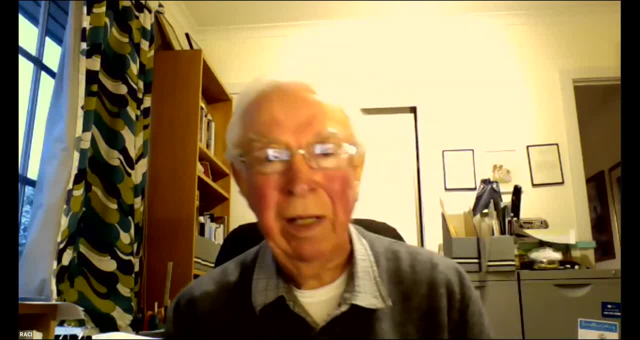 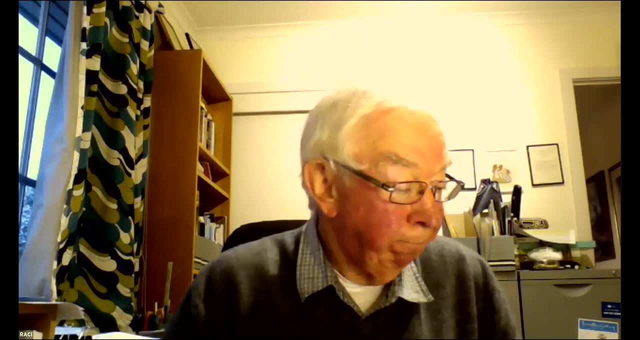 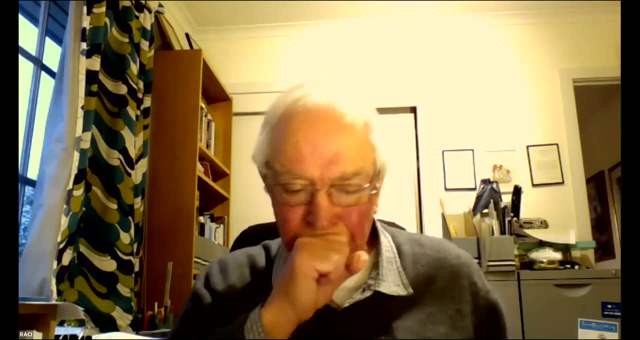 how long we go, but I'd hope to close the meeting by seven o'clock at the latest. give people a chance to well do something else this evening. So thank you again, Susie, for agreeing to Well. meet me is no picture. 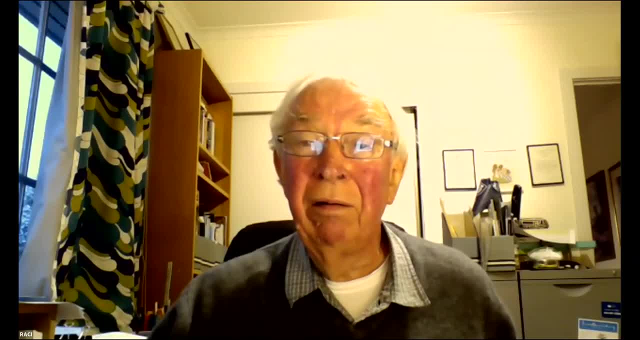 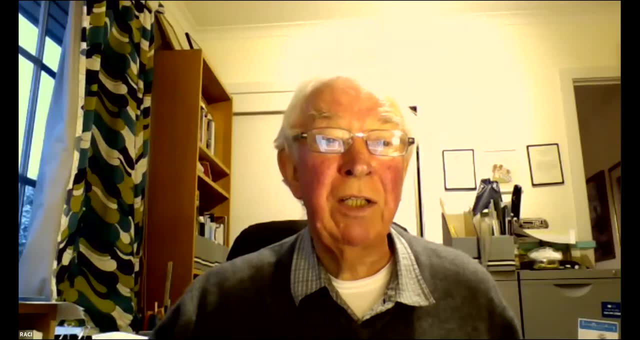 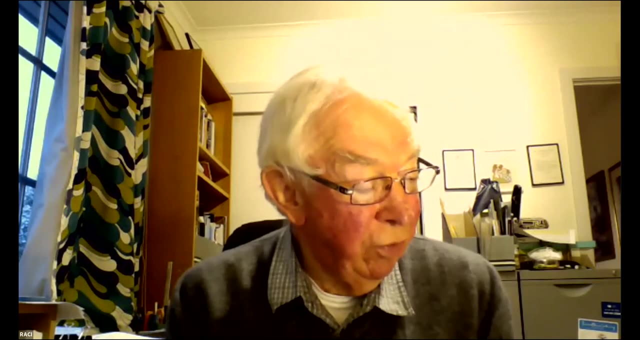 Sounds like Ian No picture. I don't know where he is. He's there somewhere. Ian Thomas, right, I've just muted him for a moment. He's there, but Joan might be there. I'll introduce Susie now to say that Susie, Associate Professor Susie Reichmann. 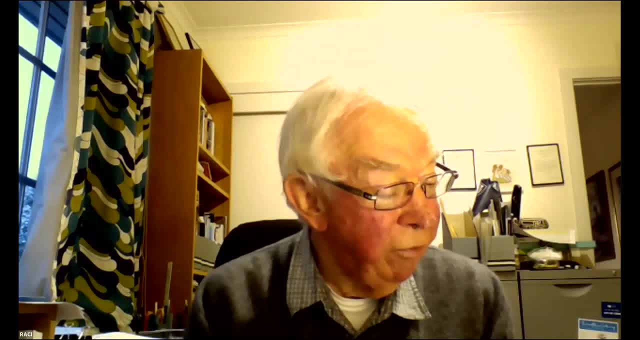 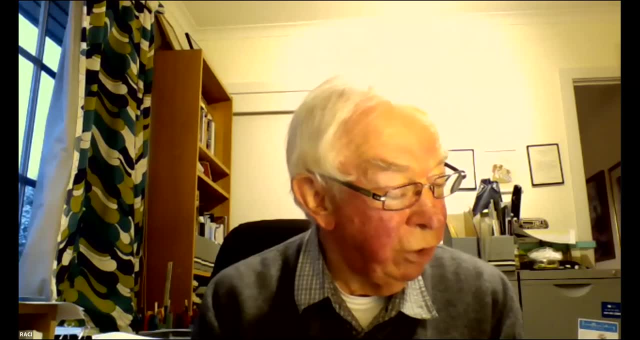 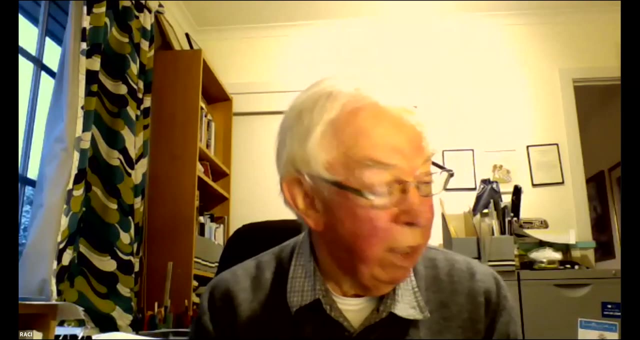 her research focuses on the fate and behaviour of contaminants in the environment, including in soil plants and the environment, Great invertebrates and risks to human health. She graduated in 2002 with a PhD in mine rehabilitation from the University of Queensland and is currently an academic. 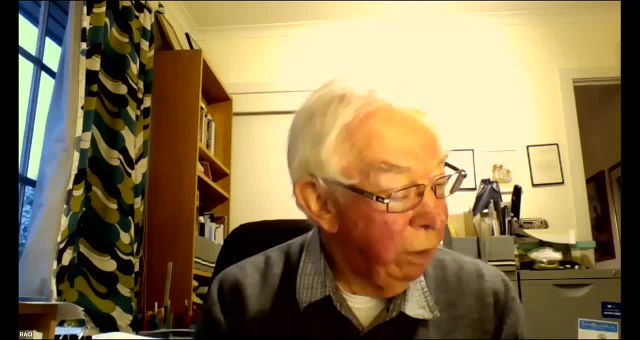 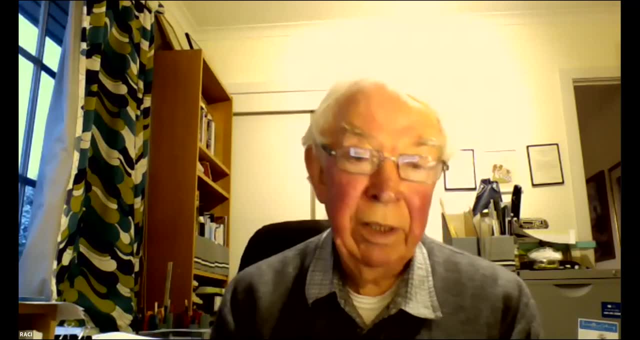 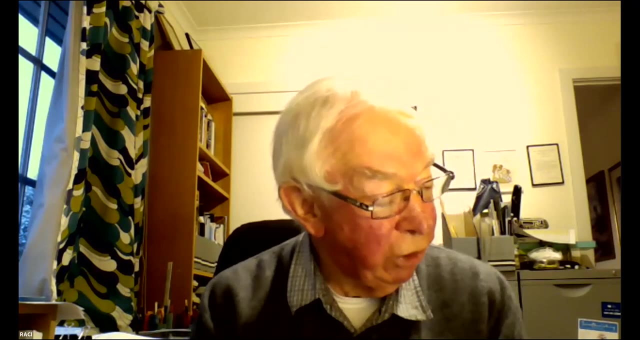 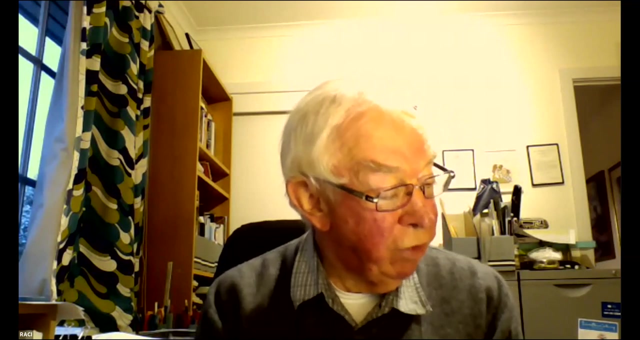 at RMIT University in Melbourne. Associate Professor Reichman has also worked for the University of California, the University of Melbourne, Lincoln University in New Zealand and the EPA in Victoria. The research currently has a focus on pollution in urban environments and in Antarctica. Susie's research has 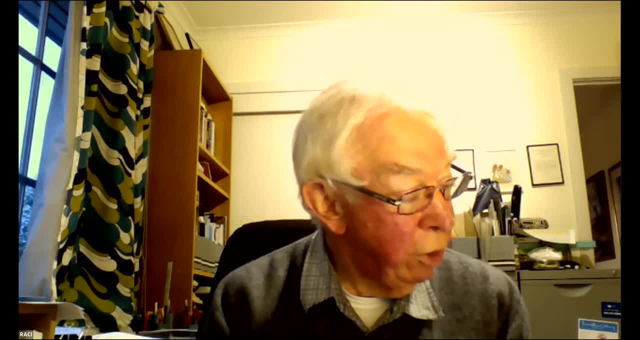 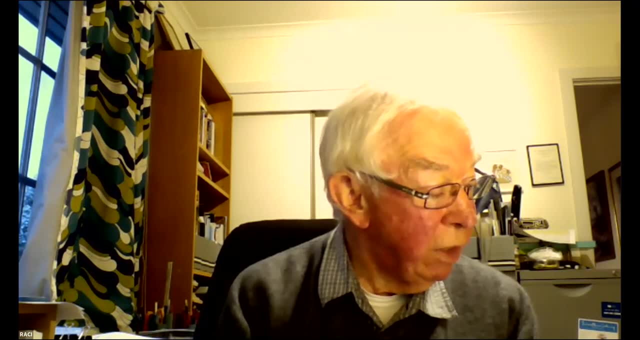 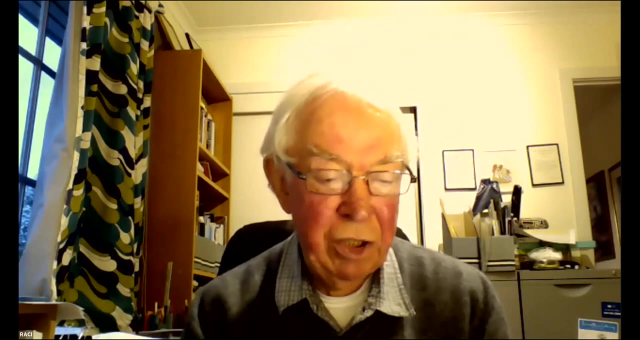 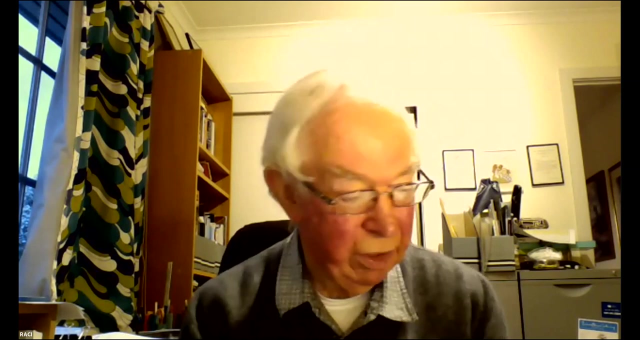 been translated into government guidance and policy used by industry to make more accurate risk assessments of contaminated environments and by the community to garden more safely. So it gives me very great pleasure to introduce Susie Reichman. Thank you again, Susie, for agreeing to speak at this first inaugural webinar and meeting of the 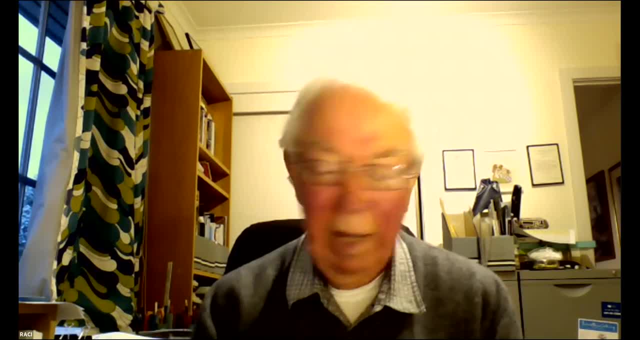 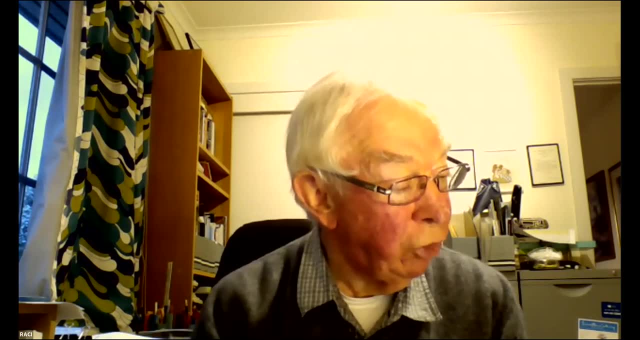 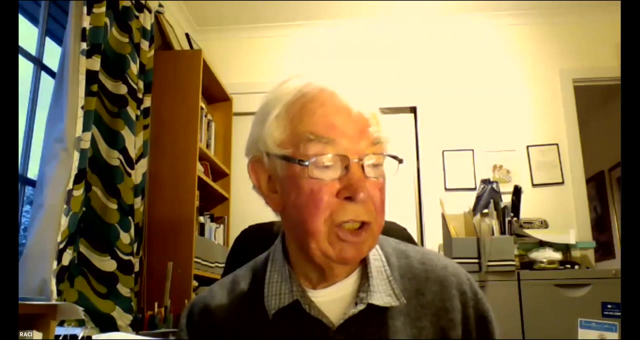 health, safety and environment group via zoom, and we're looking forward to your presentation, which I understand is reducing the risk of pollution to humans and the environment, and it's going to cover a fair amount of your recent research. Thank you, I certainly have learned the latest research What you have have Spaß. 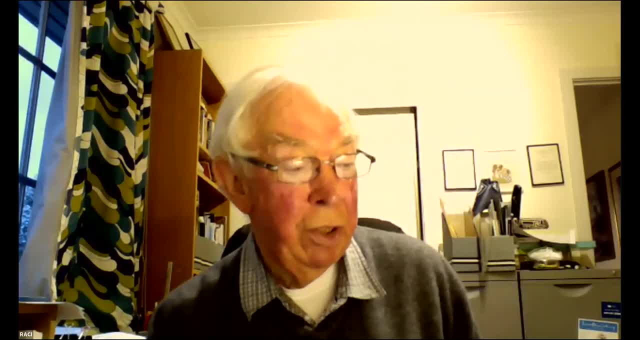 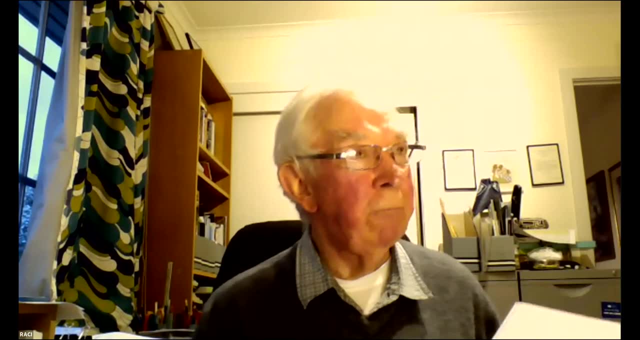 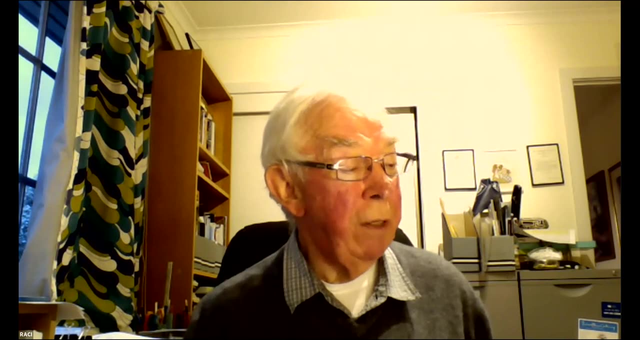 essential. you will introduce two students who will subsequently be talking to us, who, in June, move will be talking about the influence of palladium compounds and field samples on petitioning and aging in soil, And justin Morrissey will talk about the effect of environmental variables and how these will impact on people. Alfie and his family, success and頭. 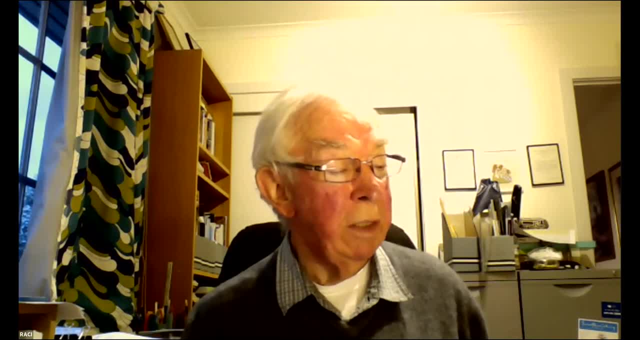 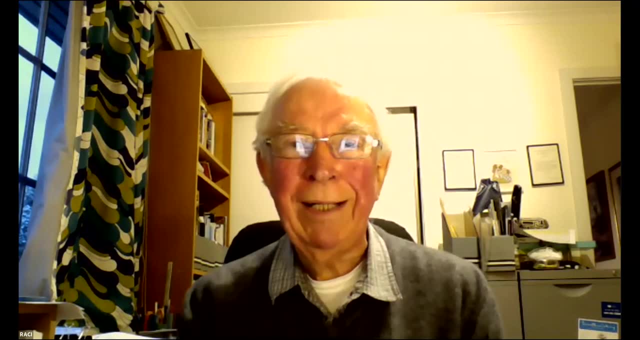 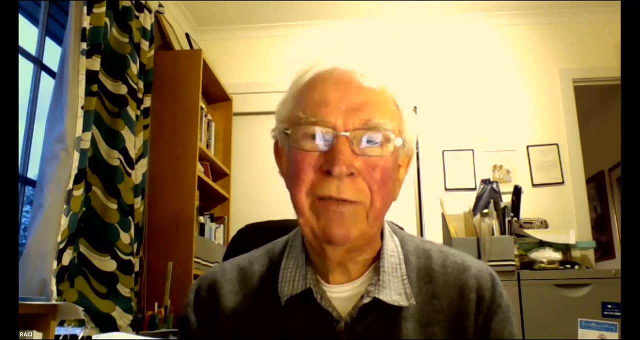 on microorganisms in a nitrogen-contaminated aquifer. So can everyone join me, probably virtually, in welcoming Susie and to say thank you for coming and we're looking forward to your presentation this evening. And before I do that, Ian, I've got a note from Ian Thomas. 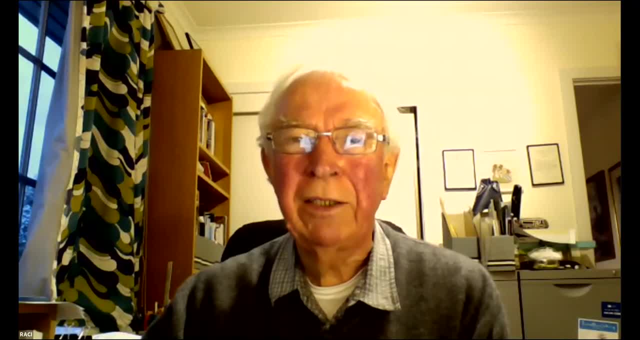 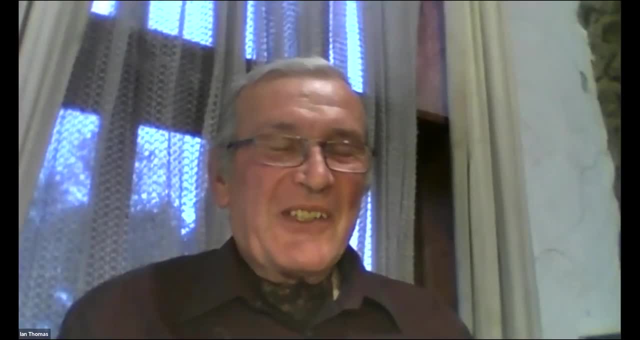 I've got a note from Joan that you weren't feeling well. Are you planning to join us? Take yourself off mute. Yeah, I'm going to try. I'm going to try. It's just a typical dose of migraine, but I think I can see you all right. 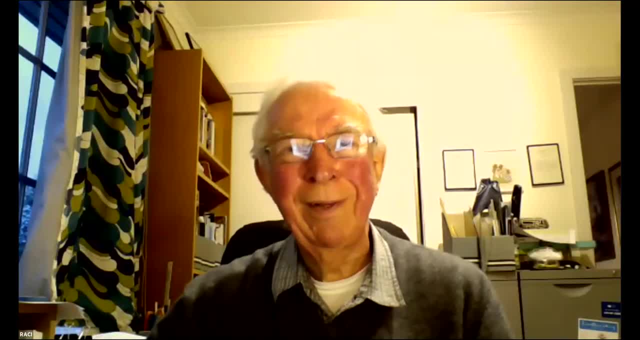 so I'll give it a go, All right. Well, thank you, Hello everybody, and hello Susie as well, of course. Good, Okay, Hi, Ian. Good, So Susie over to you. 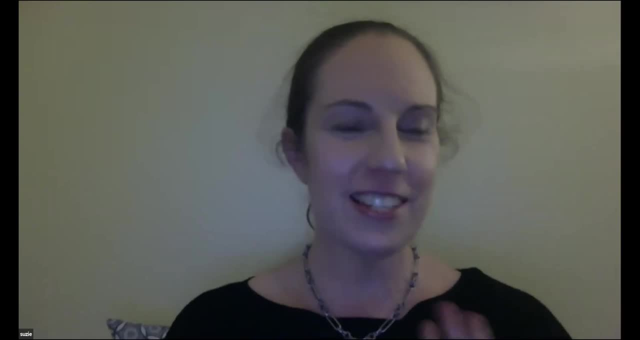 Okay, Thanks very much, Richard. Thanks everyone. A confession: This is the first time I've given a presentation over Zoom. RMIT is a big Teams and Skype organisation, so we'll just see how we go. But please bear with me if there are any issues. 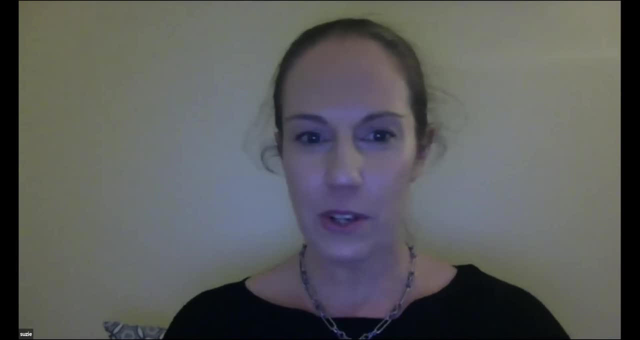 Okay, I'm just going to share. All right, We've got the first issue, because even though I have my PowerPoint open, it's not seeming to want to share it, So let's just try again. Oh no, here we go. 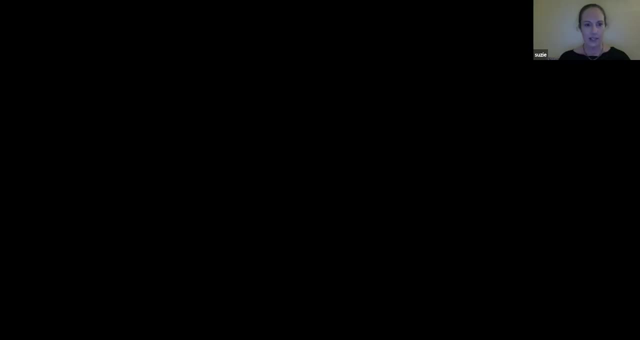 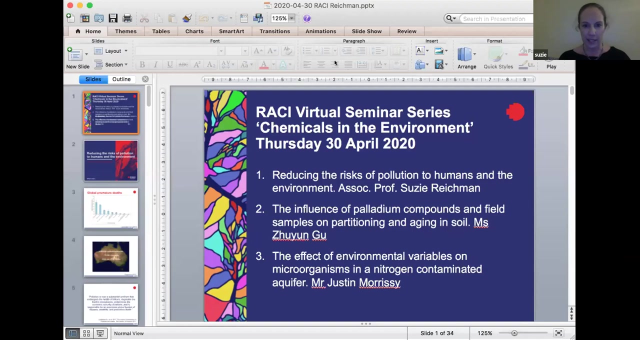 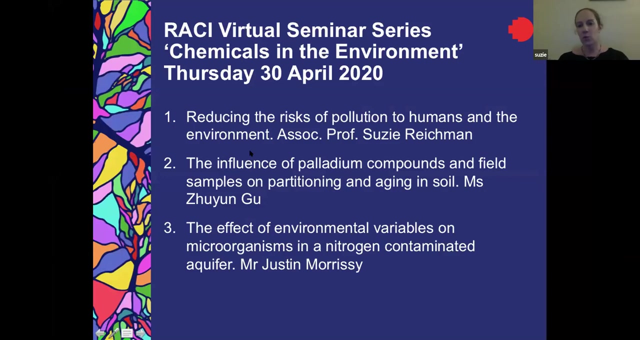 Great, It's showing it up now, Okay, So, hopefully, All right, Now let's get this. so we've got the slideshow going, Okay, Okay. So these are the three talks that we're going to be giving this evening. Richard's already introduced, so I think I'll just start with my talk. 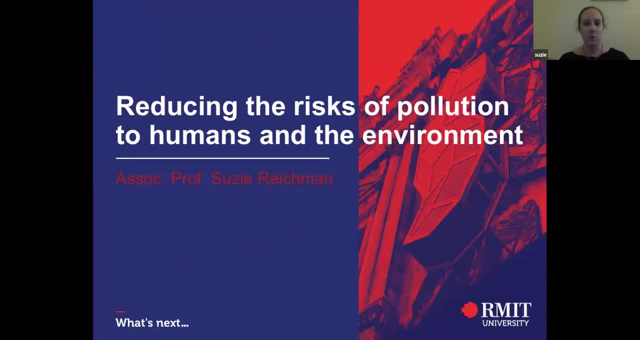 So, like Richard said, we're going to be talking about reducing the risk of pollution to humans and the environment and basically giving you a bit of a wander through the sort of research that we're doing, some of the more recent research that we've been doing in this area. 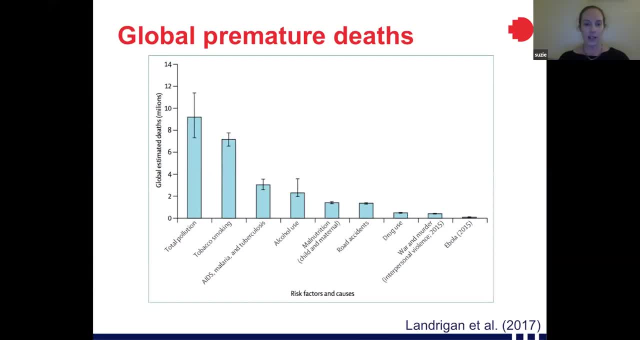 So, just to get a bit of context going, This is a sort of landmark study that came out in the Lancet in 2017, looking at premature deaths from a whole range of different things, And over here we have actually I don't know- 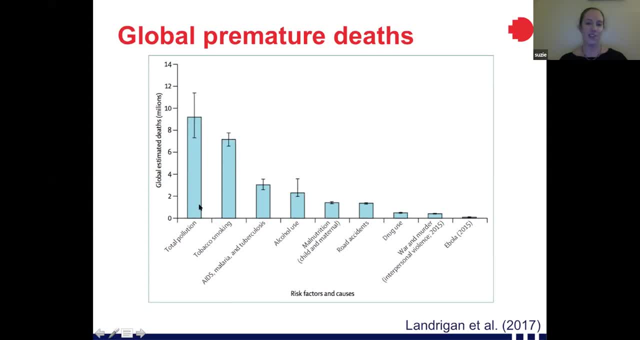 can you see my cursor? Everyone can see my cursor. Great, All right. So over here we have total pollution, and you can see that it's quite a bit higher, even than things like tobacco smoking, you know, and it dwarfs AIDS. 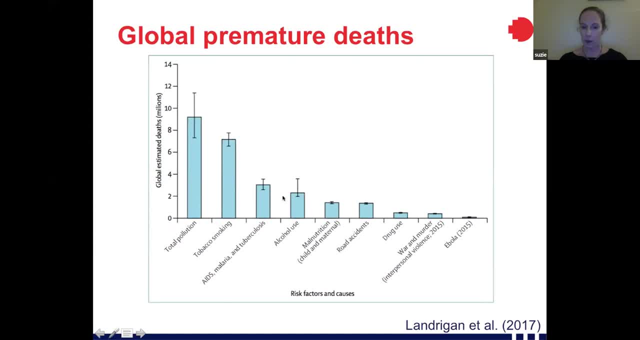 malaria and tuberculosis, dwarfs, premature deaths from alcohol use, malnutrition, road accidents, drug use- we're going down war and murder. So- and this is only the deaths from pollution, This is for human deaths. This is not. 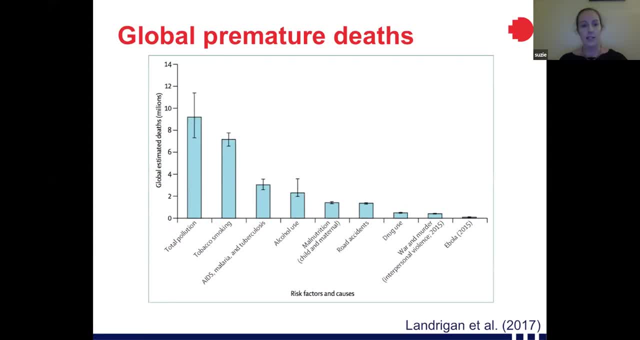 you know people who are sick and have chronic issues because of it, And so you can see that it's quite a major issue. pollution around the world It's also- it's only the deaths that they were they could catalogue with quite a degree of confidence. 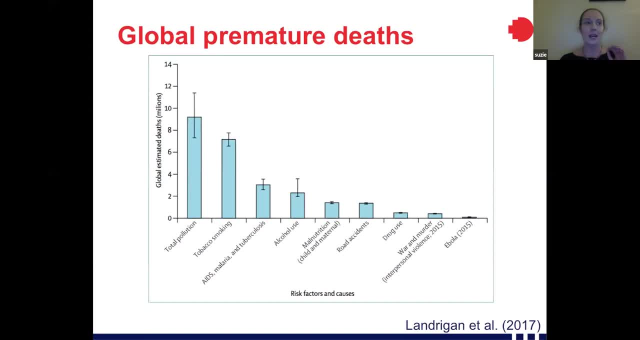 And they admitted in the report that there were quite a few that it you know it wasn't a hundred percent clear the link to pollution and they didn't include any of them. So probably the deaths from pollution of course, are quite a lot higher than the sort of around about 9 million that. 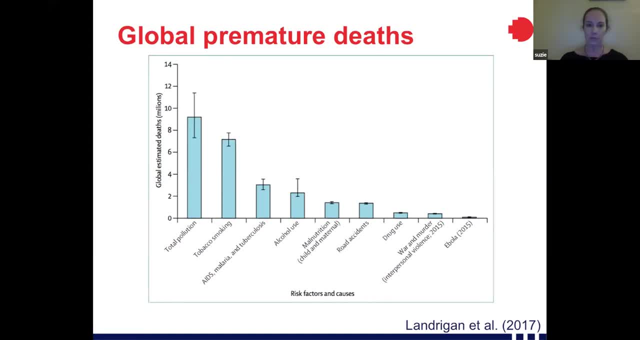 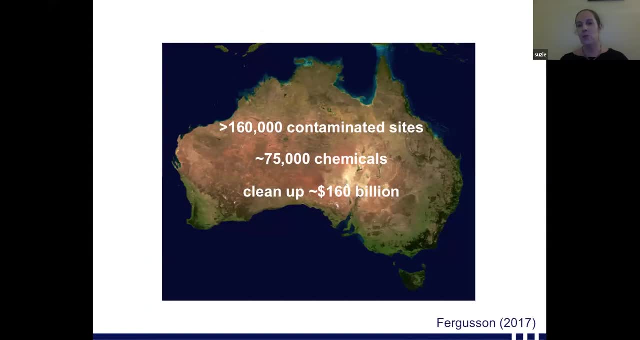 we're getting annually at the moment that they can document really well, And we tend to think of Australia as this clean, green environment, but we have a number of pollution sites to contaminated land as my main area. So again, there was another study that came out in 2017 by Ferguson. 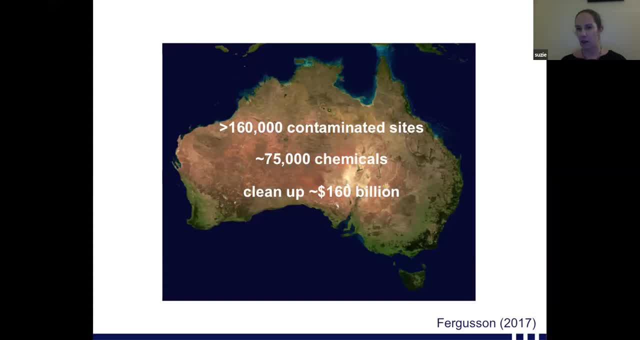 that documented the amount of contaminated land And they found that it's over 160,000, just within Australia, contaminated with approximately up to 75,000 chemicals. So a lot of these are unknown but we know- we know that these chemicals have been used in Australia and are likely to. 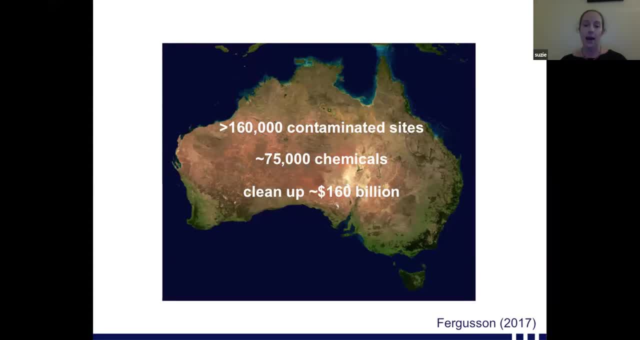 be in these sort of waste sites, And the cleanup is estimated to cost 160 billion. So this is a major issue. It's a major issue globally and it's a major issue in Australia, And so this is again. this is a quote. 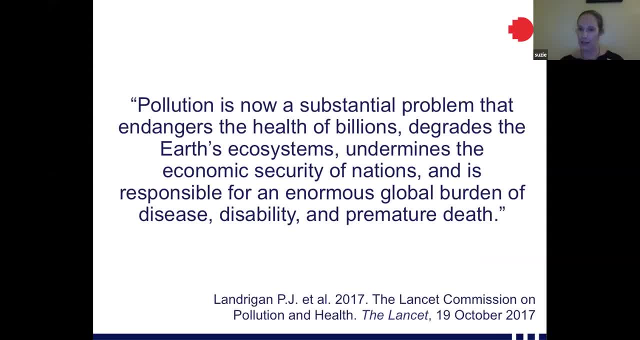 I think that sort of summarizes a really well. that came out of that Lancet article And they said: pollution is now a substantial problem. And you know, because of the little videos down there and I can't read it all, So I'm going to guess at my own quote. 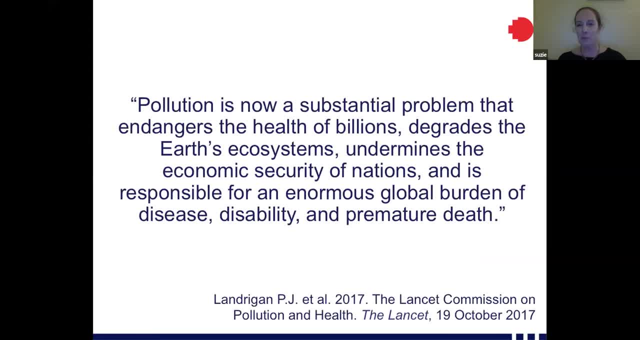 pollution is now a substantial problem, endangers the health of billions, degrades earth's ecosystems, undermines the economic security of nations and is responsible for an enormous global burden of disease, disability and premature death. It summons up that you know this is a serious issue and that it has many 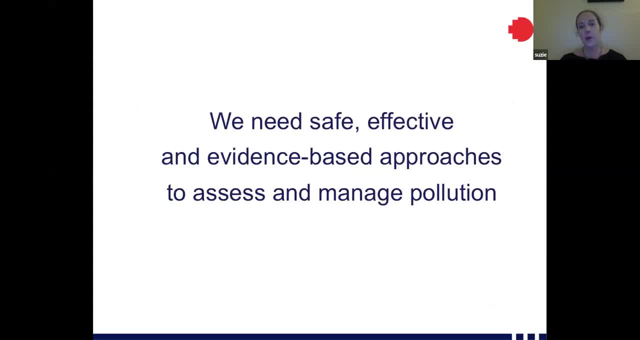 many impacts, And so what we need going forward is safe, effective and evidence-based pollution, evidence-based approaches to assess and manage pollution- And, of course, this is where we as a research team come in- is is getting those evidence-based approaches to being able to assess and manage. 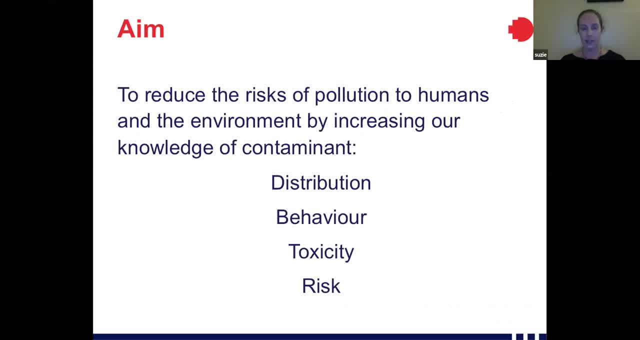 pollution. So I think it's important to think about this pollution out there in the environment, And so the aim of my research team at RMIT is to reduce the risks of pollutions to humans in the environment, where traditionally I've done mostly research in environmental aspects rather than direct human. 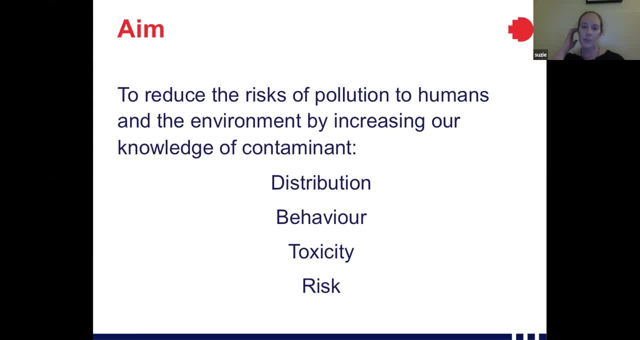 health. but we're starting to do more and more human health And we do that in a number of ways by increasing our knowledge of contaminant distribution, behaviour, toxicity and risk. So I have a number of areas of expertise. It's very multidisciplinary what we're doing. 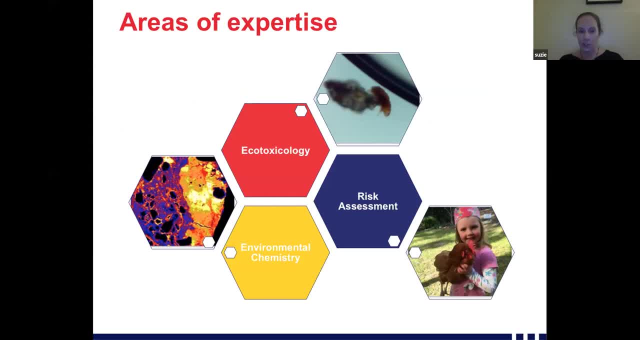 And the main three areas where we're acting in are ecotoxicology, environmental chemistry- which is why I'm here tonight- and then linking them together in risk assessment- And when I say risk assessment because it's research most of the time. 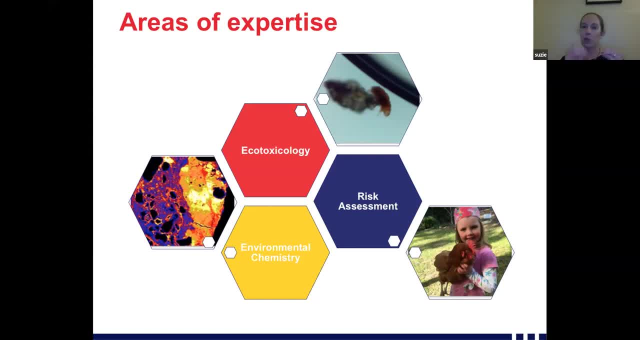 we're not doing a risk assessment from go to woe. we're looking at aspects of risk assessment And how can we provide more information for them, how can we give more certainty around numbers, validate various things that are being done. So it's really in that research context that we're doing parts of. 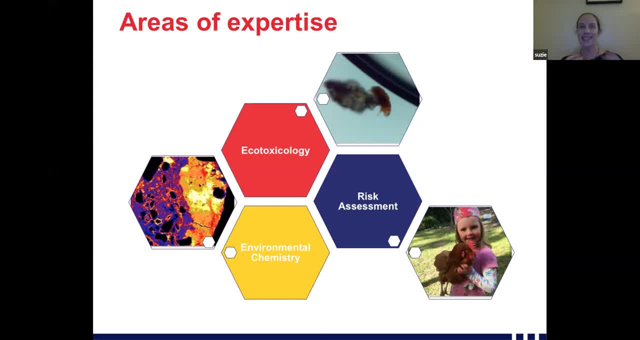 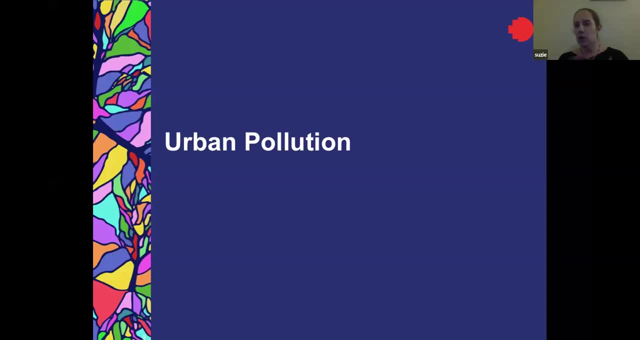 improving risk assessments or assessing, in certain situations, whether or not this might be an issue. So I'm going to talk about three different areas of our research tonight. I'm going to start talking about pollution- Urban pollution- And then move on to looking at ambient background concentrations. 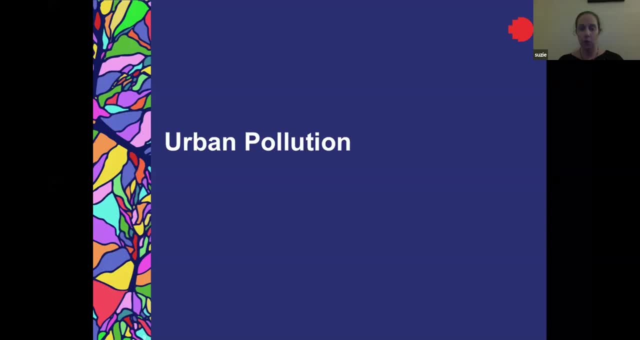 And then finish up with looking at our Antarctic research, which is a bit newer than the other research I'm going to be talking about, And then Juin and Justin are going to go and talk about another couple of aspects that are directly related to their PhDs. 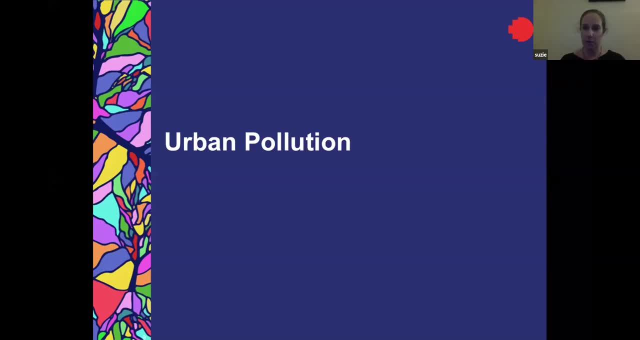 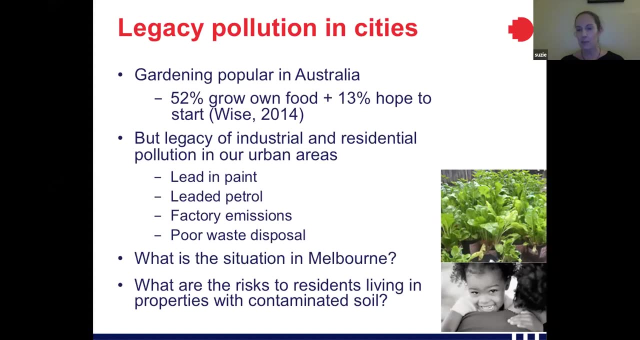 And I'll introduce them as we get up to them. So, moving back to urban pollution, So We have this legacy of pollution in our cities and I'm going to be a bit Melbourne focused tonight because we, you know RMIT's in Melbourne and the 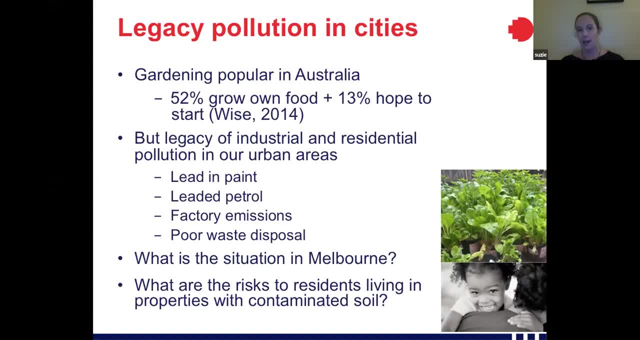 research we're doing has tended to be Melbourne focused, But a lot of what I'm talking about holds in other cities in Australia and around the world. So in 2014,, the study came out looking at how much gardening to grow some of people's food they were doing. 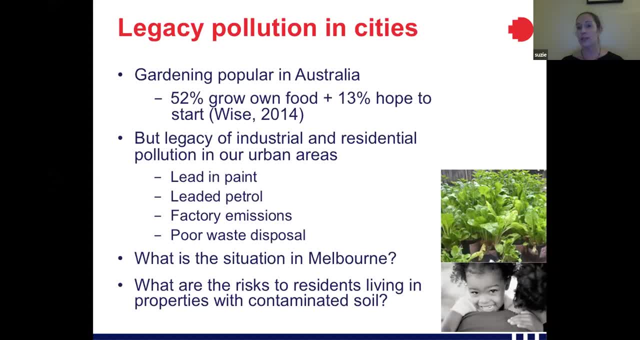 And they found that 52% of people who were doing it were people who were doing it for a living. So a lot of people- about 50% of people- were already growing some of their own food. Now that could be as small as you've got a pot of parsley on your 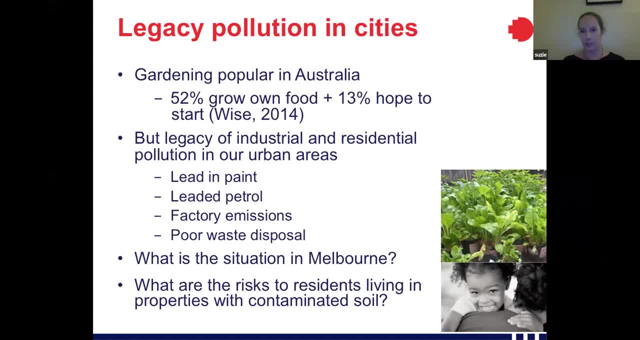 window sill up to you know you're semi self-sufficient kind of thing, or completely self-sufficient in the food you're growing And they've had another 13% were hoping to start. So we're getting up to about two-thirds of people are either growing some 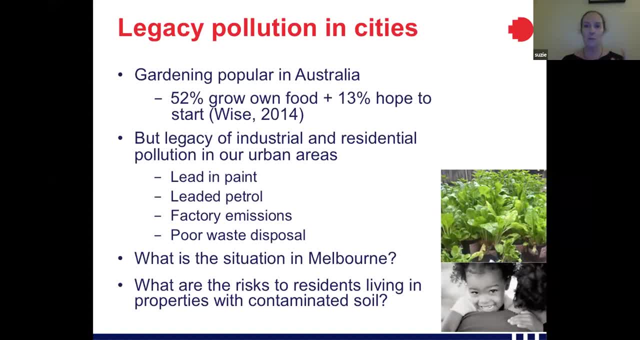 of their own food or really interested in it. And I think if you've been watching the media recently to do with COVID-19, you'll know there's been a lot more people with a problem starting um recently and you know, some of you, even in the audience, may be giving gardening a go. 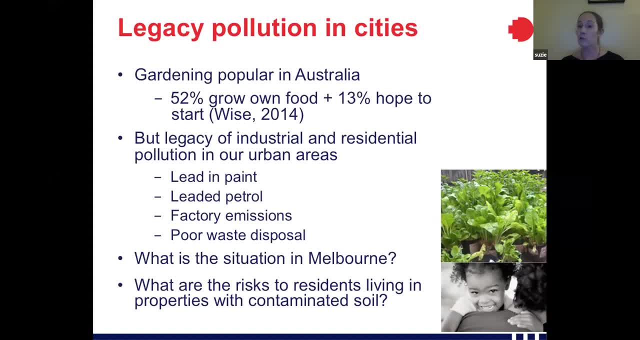 gardening so much, but vegetable gardening ago, or some sort of food production. apparently you can't buy chickens because um, all the chickens, the little baby chickens, are sold out because people are taking up um keeping chickens for the first time too. so we're in a situation where um gardening 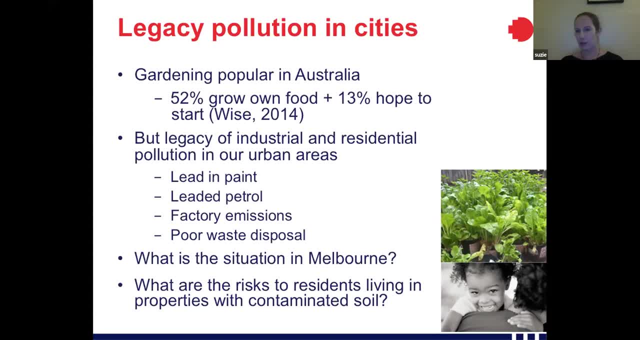 to grow food is popular and at the moment we're seeing it growing even more than it has been previously. um, but when we're in urban areas, we've got this legacy of industrial and residential pollution from a number of sources. uh, for many, many years we had high concentrations of lead. 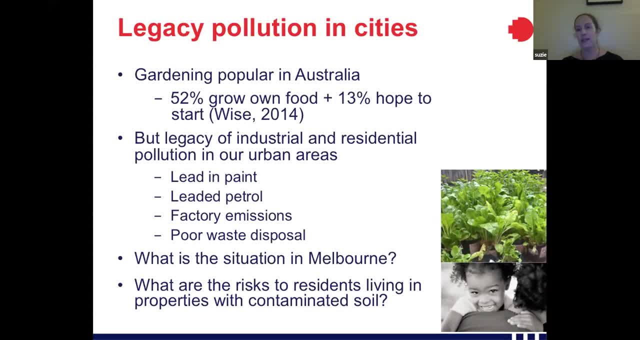 in our paint uh up to 50 percent um and then that decreased throughout the 20th century um. but we've ended up with, as paint flakes off um the painted surfaces and it ends up in the soil and over time that builds up and so we have some soils that are quite contaminated because of that. 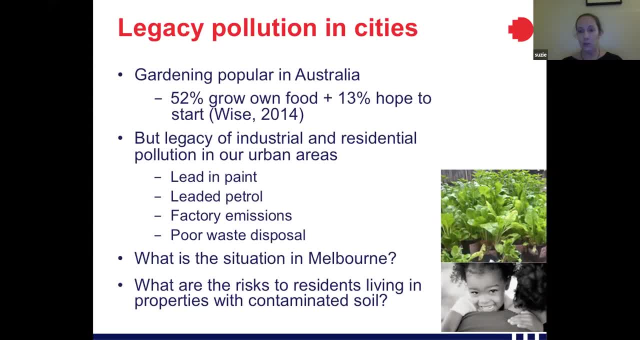 um, and so we've had a lot of people who have been in the industry for a long time, and they've been in the industry for a long time, and they've been in the industry for a long time and they've, of course, we had many years of um lead in our petrol as an anti-knocking agent, and that only. 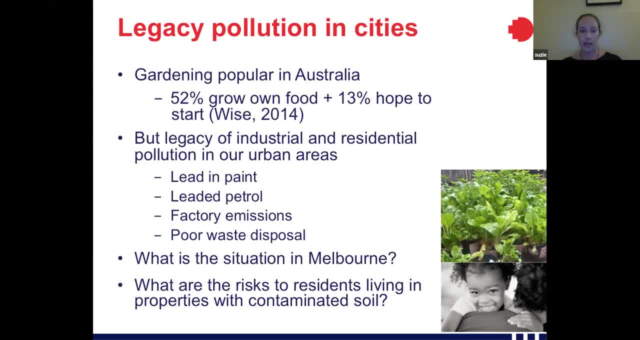 came out completely out of our petrol in australia in the early 2000s, um, and so we have lead even in um quite pristine areas in australia. um we we have a sort of a background amount of um or baseline amount of lead that's there from the lead in our petrol and then of course there. 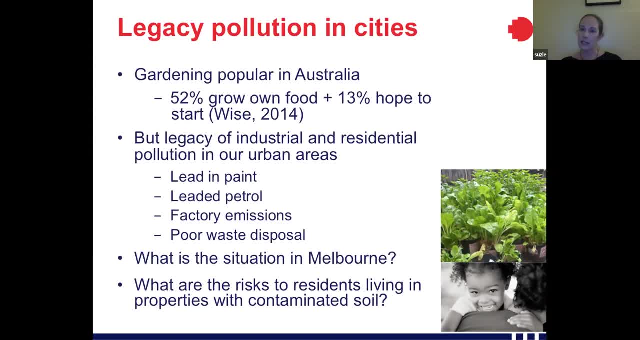 were various factory emissions um. melbourne in particular was a big pottery um and so um producing um town for quite a while and then in various ways, over the um, over the history of melbourne and cities where we weren't so good with our waste disposal and so things weren't 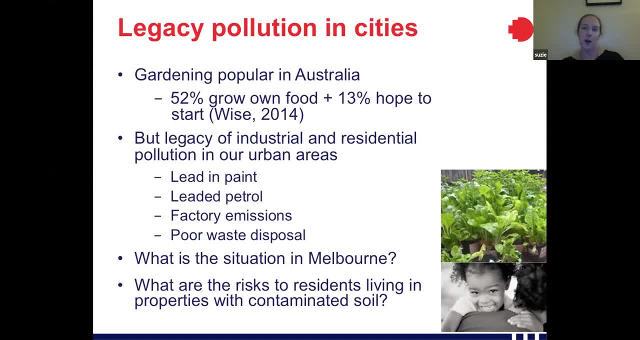 necessarily um disposed of. you know, often they might just be disposed out the back um and you might end up with areas that are quite even in urban environments, that are quite contaminated, and so there hadn't actually really been very much done. i mean, well, there were a lot of. 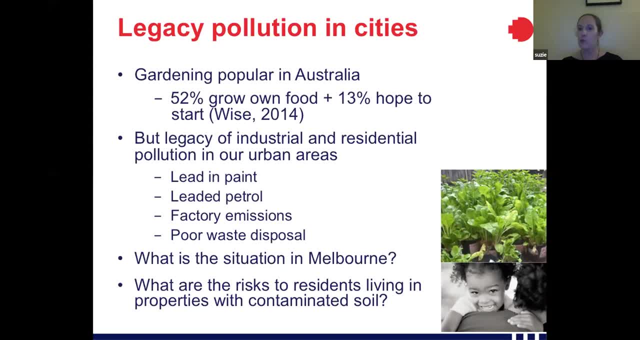 there hadn't been very much done in people's homes. this mainly what had been done was in brownfield sites where they were wanting to redevelop it. but we just wanted to go and say, well, where you know, people have been living there in houses you know, maybe for 100, 150 years, what's. 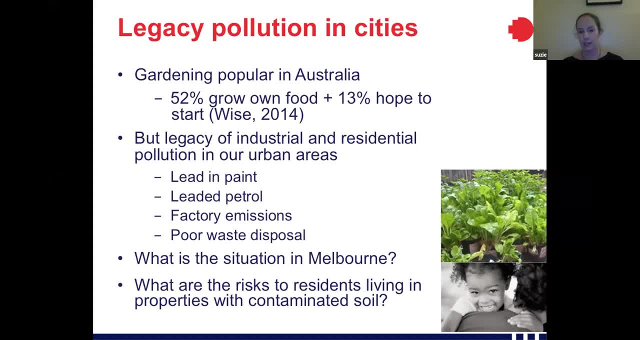 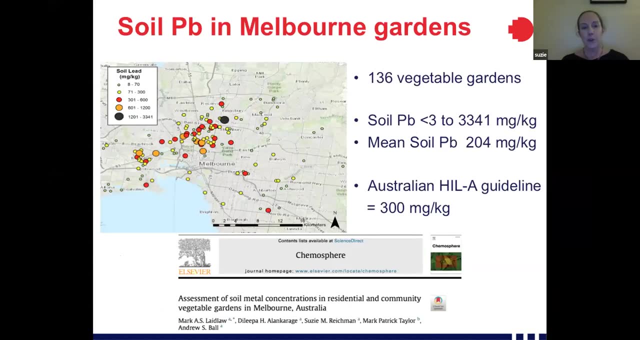 the situation and then what are the risks to residents living in properties with that contaminated soil, which i'm not going to talk so much about um today, just touch on the risks, bit a little bit um, but more sort of talk about what we've been finding. so um first study we undertook um was with a master's student, um dalipa alacaraj, and uh postdoc. 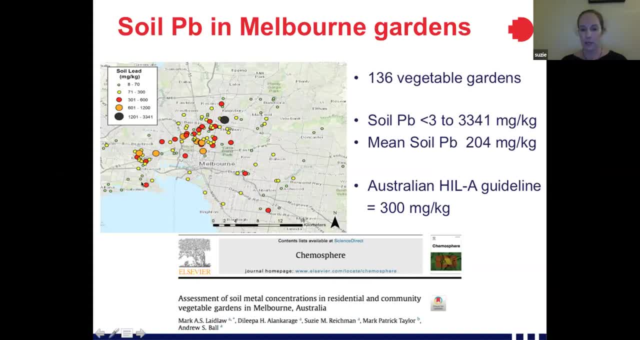 mark laidlaw, and we also collaborated with um for the bit i'm presenting of this study here um. some of you might know mark taylor from um, new south wales and he has his veggie safe program and he donated his veggie safe um data. that's a community um a citizen science program where 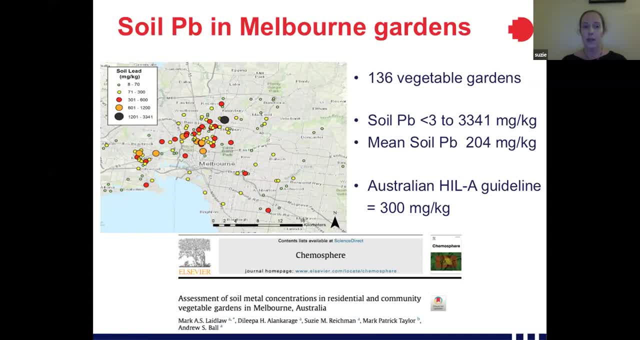 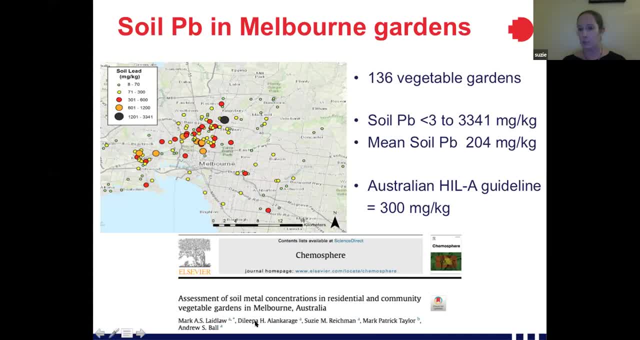 about um ourselves, which was dalipa's um master's project. i'm not going to be talking about that tonight, just to sort of keep things in check. but you know, we ended up with 100 soil from 136 vegetable gardens and we found that the lead in soil ranged from um less than three milligrams. 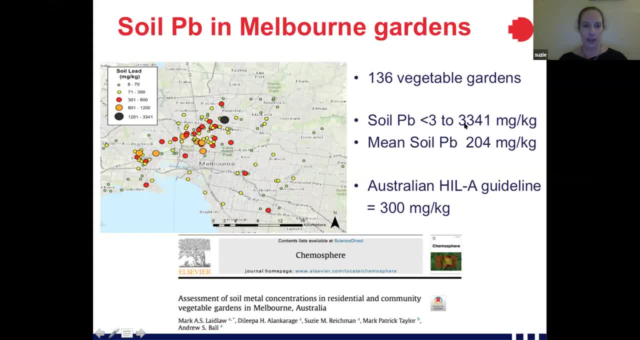 per kilogram up to over three thousand, over three thousand, uh, with a mean soil concentration in the 200s, and so we ended up with quite a lot of soil. if you look at the map here, everything that is orange, red or black is above our australian um health. 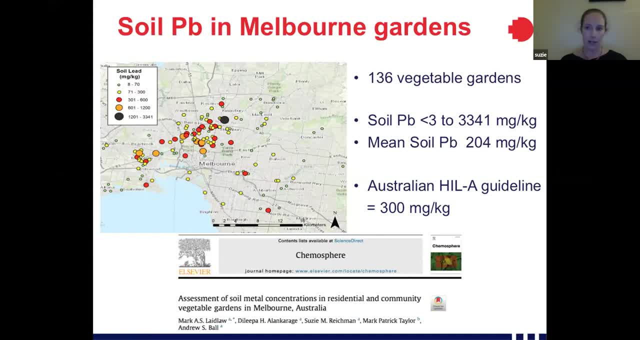 investigation level a. so that's our level of contaminated land um where, if it's above that, you need to the the um. if you were doing a risk assessment, you would suggest that they go away and do a full risk assessment on that land um and so you can see. 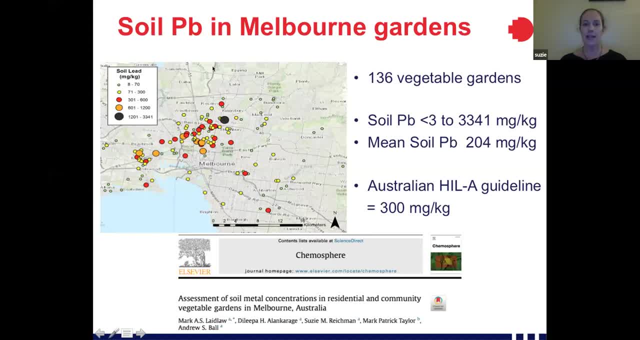 it's. it's pretty um evenly distributed. maybe not in outer melbourne really, when you're getting to outer melbourne, but you know around quite a lot of um. we're still here getting out sort of um 15, 20k and still getting some red ones um out of melbourne. um we found in um this study. we found about 20. 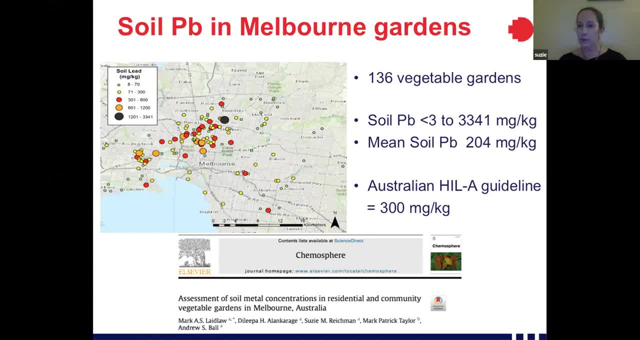 of uh houses had soil that was above the hila and um subsequent studies that we've done, it was more like around about 10 percent, and so we think this was a little bit biased, because people were sending in their soil because they thought that there might. 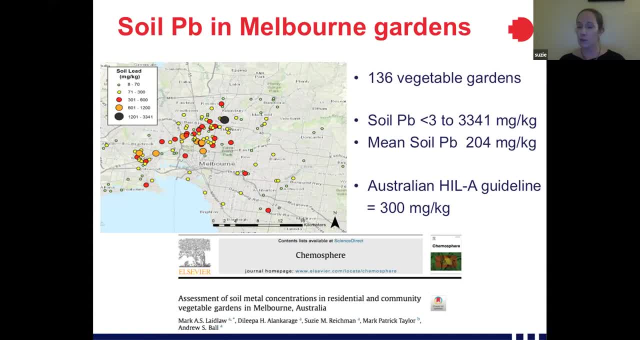 be an issue. so we think it's a bit higher um. this is much lower than the research mark um taylor's done in sydney, where they've gotten up to about 40 percent in sydney, which makes sense. sydney's older um- and this has been published- um in chemosphere and with this piece of information, 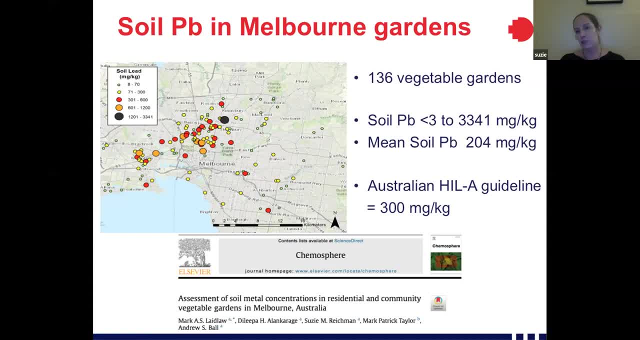 this. it was a fairly simple study, but we thought that this was the sort of thing that, um, the community might be quite interested in, uh, and so we went to the press with it. um, and i have, i've got quite a good. you know, i, um, as richard mentioned, i used to work for. 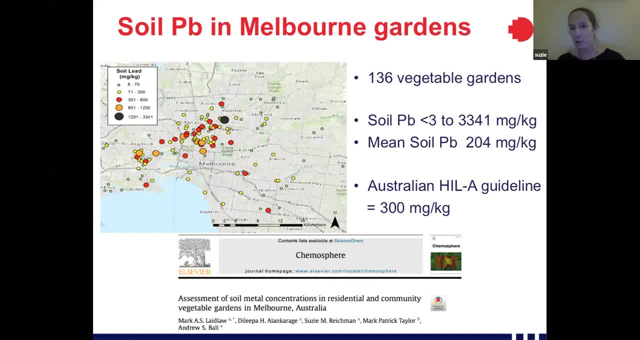 epa victoria. so i've got quite a good relationship with them. i collaborate with them. i didn't want this to hit the press without them being aware, so we actually talked to them before we went to the press and, um, i think i had more impact over. we did this big weekend where i was on the news. 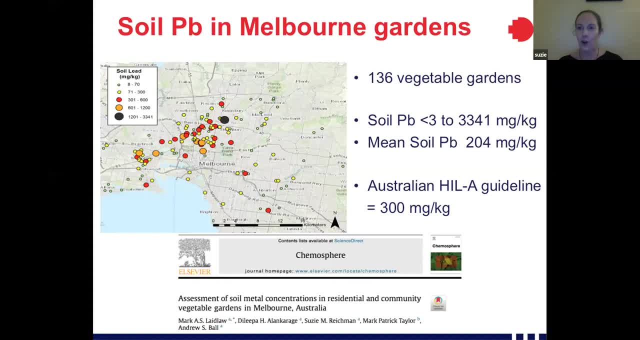 um in newspapers, on the radio um, and because we talked to epa victoria, they had, previous to that, had no um guidance out there for people who might garden and be worried about their um. lead, which was really the only metal that we found, was consistently high um, but by the weekend they 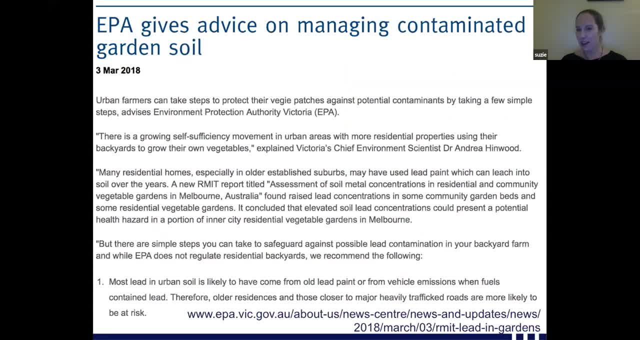 had up some guidance and this is. i think i had more impact um by being involved in this one study and taking it to the press than i did the whole time that i was at epa. i think it's the fastest that i know they've ever gotten guidance out and it's fantastic because 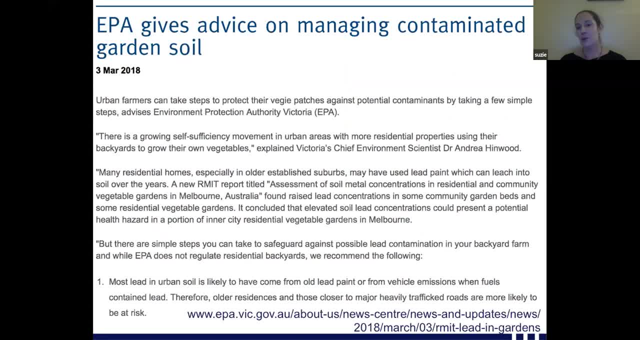 there's now guidance out for people, um, who might be in victoria, for people who might be worried about having lead contaminated soil and how to deal with that. um, and that's up. you can, um, i mean, if you google rmit and soil and lead, um, i think it comes up in the first few. 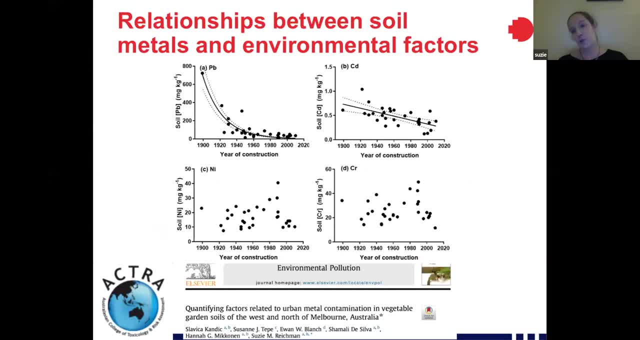 um, so we've been continuing doing more research in this area. i have a phd student um so it's a research and she's just writing up at the moment and she started to look at um more the relationships and the risk, and so she's had a paper published. um we looked at the top one here is lead cadmium. 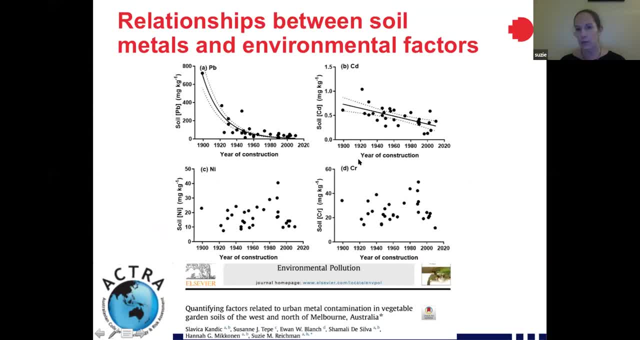 nickel and chromium. we looked at a whole lot of environmental factors, age of house here, so year of construction, you can see we've got fantastic relationship with um lead r squared of over 0.9 um. a good relationship with cadmium, but the cadmium's um it's elevated. 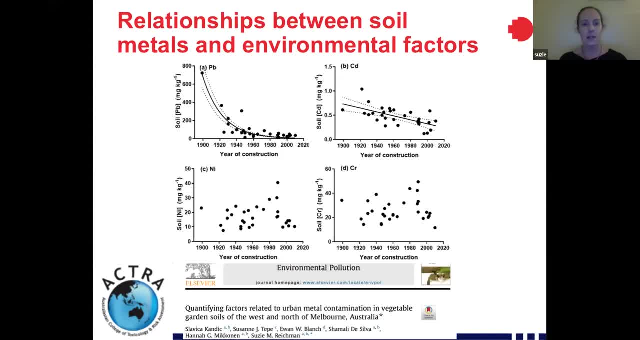 but it's not above levels that you'd be particularly worried about. um, nickel and chromium, we didn't really find any relationship with factors like distance to road or age of house or whether it was painted or not. um, and we think that the nickel and the chromium levels are then 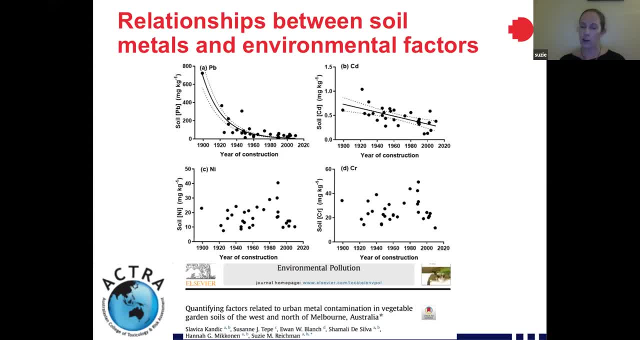 are pretty natural, pretty much those background concentrations that you'd expect. cadmium, we think, is elevated, but not to where you would expect a high risk from it and lead in these older houses um here, anything um below about um the 1950s. you're starting to get really elevated and and back um. 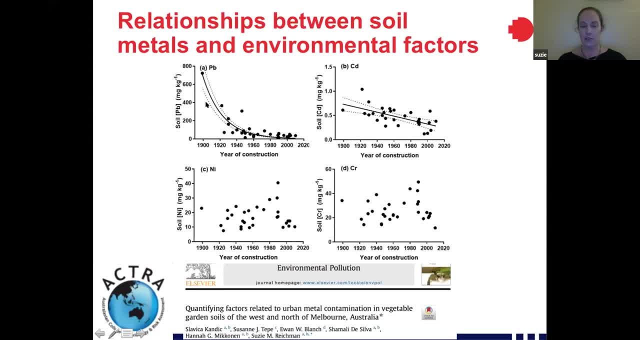 from about 1920. some houses, particularly houses that have been painted um, are having higher concentrations, and so lisa's done a whole lot of um various risk assessments. she's looked at vegetables grown in um like in situ and gone and sampled from people's vegetable gardens as well. 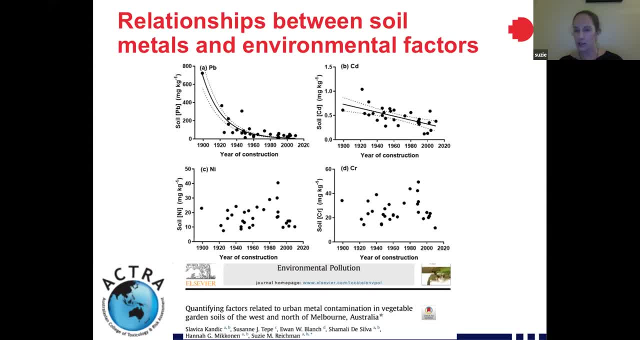 and is: um, i just i didn't want to present that yet because she hasn't published, but she's finding um, mainly that the vegetables themselves are probably fine. um, but this research, she actually won an actra, which is the australian um college of toxicology and risk assessment. she won their. 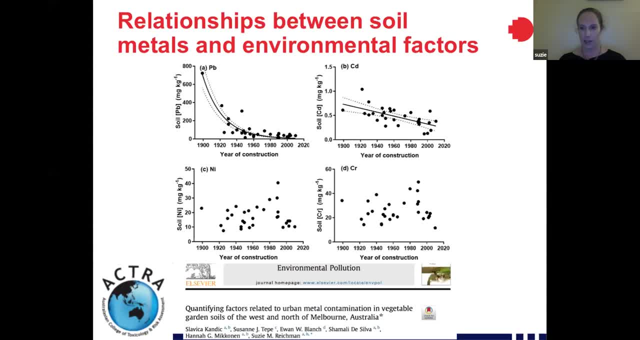 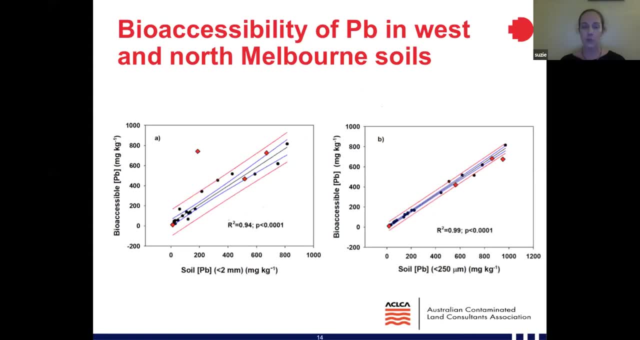 student prize a couple of years ago for it, which was great um for her um. and then just another little bit of work that she's been doing and is writing up is on these same soils. she looked also a subset of these soils. she looked at the bioaccessibility of lead and she looked at the 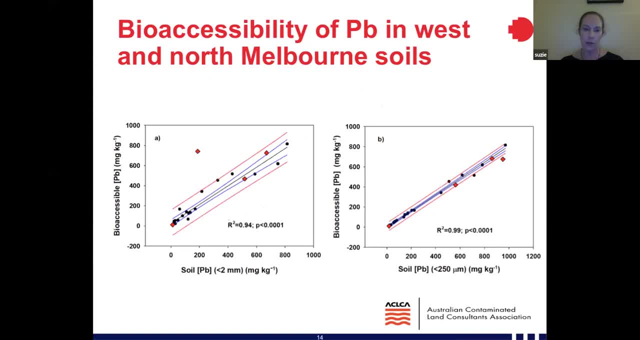 bioaccessibility of lead in. this was all in the western north of melbourne that we we were doing it um for slibitz's work, and this is the australian contaminated land consultants association. have um, uh paid for this, funded this research um because we're interested in seeing. 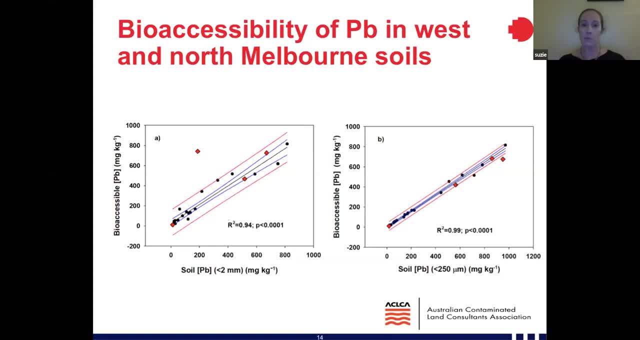 if um bioaccessible lead of people- bioaccessibility of people haven't heard of it- is when it's a um in vitro assay that simulates our digestion of um lead or other metals, other chemicals, and so you can get an idea of what's going on. and you can get an idea of what's going on. 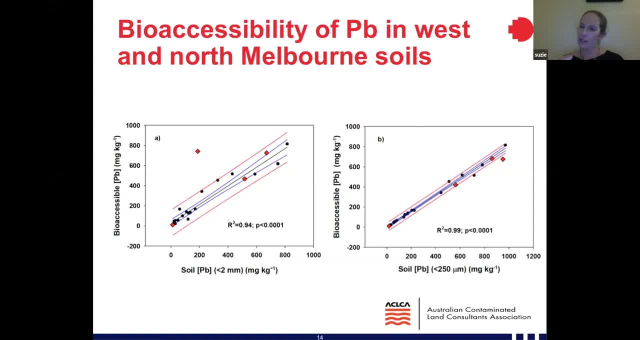 and you can get an idea of um. it's not exactly the bioavailability but it correlates very well with bioavailability. um, an in vitro, um sort of test of how much is in the stomach and able to be absorbed potentially, and it's being used more and more in risk assessment and um we wanted to. 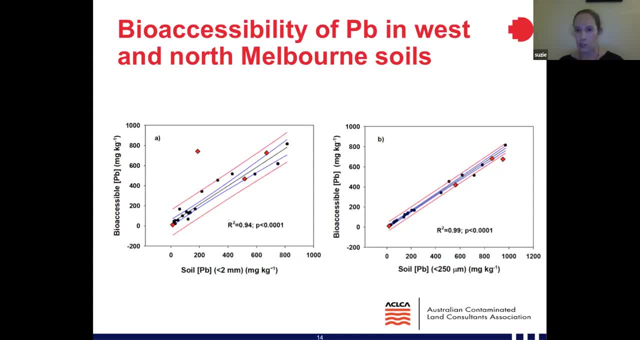 know if you could use. we have a few different questions that she was looking at um. one of them was just: could you measure, use total soil lead, like we've got down here to get a good relationship and see i haven't published the equations up here because we haven't published it yet and we don't 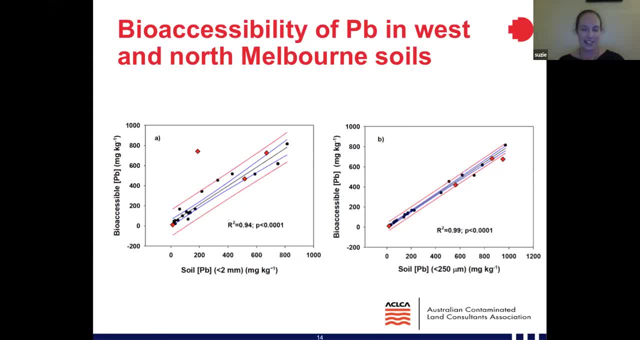 want people to use them, just in case, um, we anything gets corrected, but um, we got some fantastic. this is with soil sieve to less than 250 micrometers, which is the same um size that they use for bioaccessibility testing, because that's connected to um, what they see as the most. 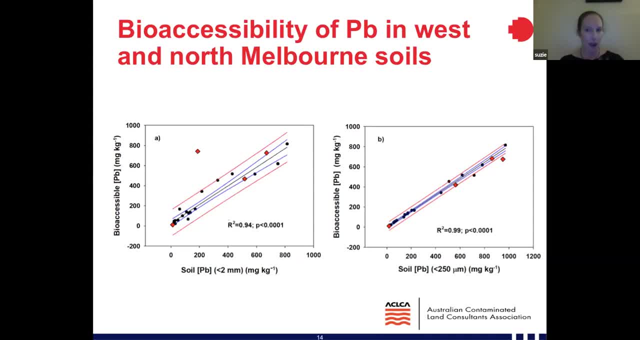 bioavailable fraction of lead and we were like, well, this is great, but it's not um. most people are doing it on larger size, for example, so we're not doing it on larger size, for example. so we're doing it on larger size fraction of soil, and so can you do it on that large size fraction of soil. 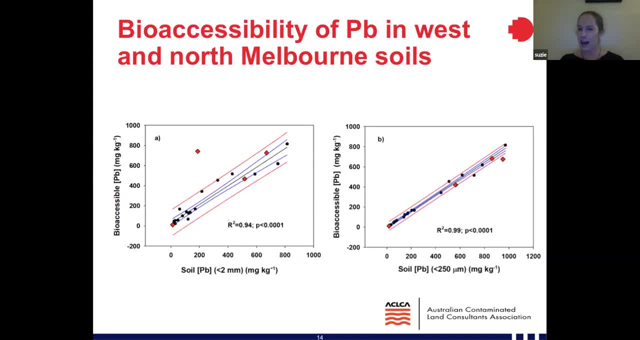 and if you talk to people who are in bioaccessibility they're very um accessibility research. they're very definite that you need that 250 micrometer um fraction or less, and so we tried. it's very relatively small group soils- western north and melbourne um mainly uh formed on. 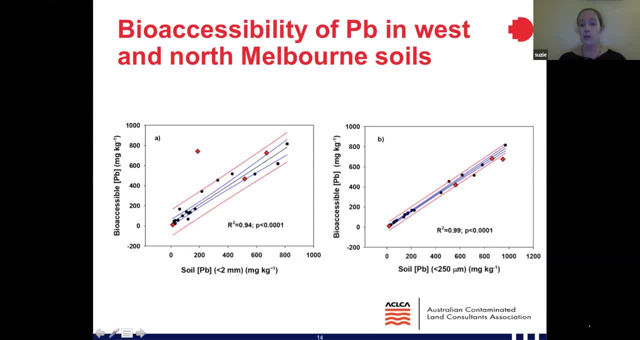 volcanic soils, so they're quite similar. um, but we got, we have some really good relationships. i mean, of course it was. you can see the confidence interval was in red. um, we're much more confident in those results. um, smaller error. uh, if you are sieving to 250. 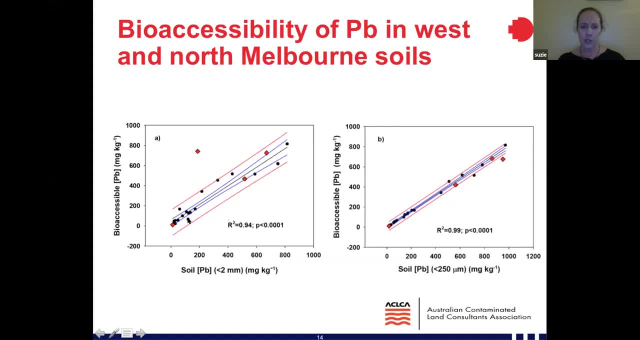 micrometer, but we still get um, we still get good relationships and r squared, 0.94 um if we're just using two millimeters, which, for soil scientists, is that standard size that we sieve to um the red diamonds that you can see? here are our validation points. you can see we've got a little bit of an. 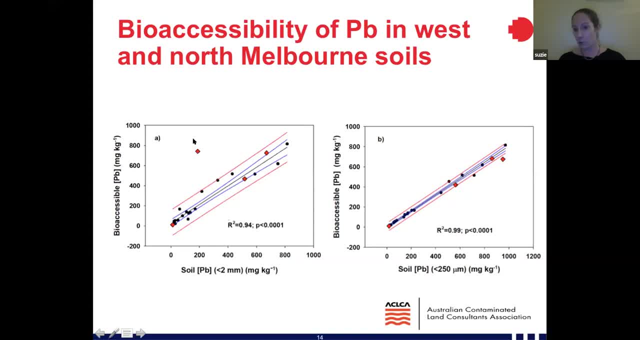 issue here, um, with one of our four validation points and still working that out, but it looks like it's something to do with the iron in the soil, that that soil um, the different relationship between total iron uh and the lead concentration there, and so we, um, it was sort of we think that we'll probably be. 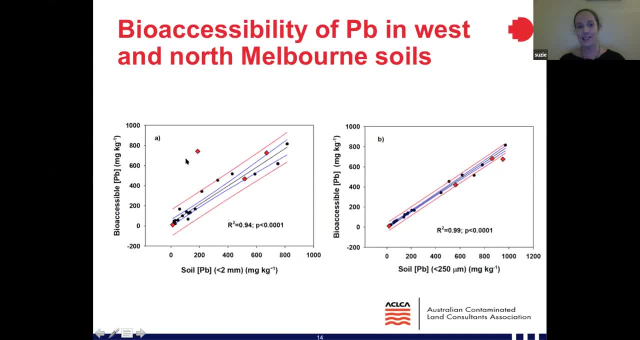 able to overcome that and work out what sort of situations it is where this relationship doesn't hold um but all up it held on the um 20 soil samples, the black dots and the red diamonds and then three of our validation ones. so we think there's something in this um being able to use. 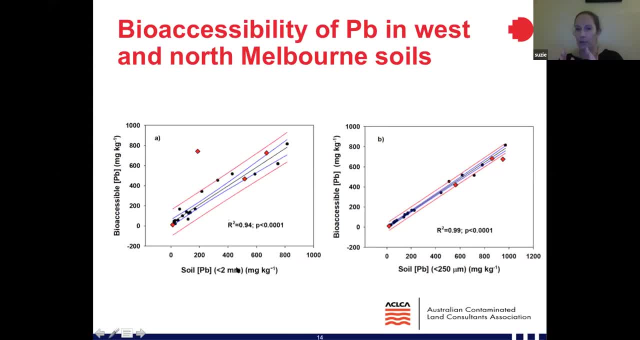 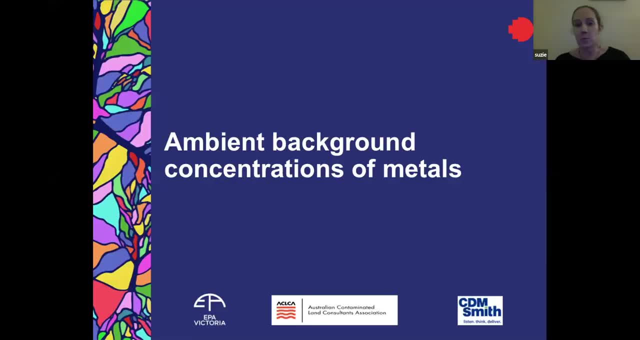 the total soil lead. of course it depends how much um you know, how much uncertainty you're okay with dealing with um. okay, so now i'm going to move on and talk a bit about um, our ambient background concentrations of metals project. this was quite a big project over three, four years. it's technically 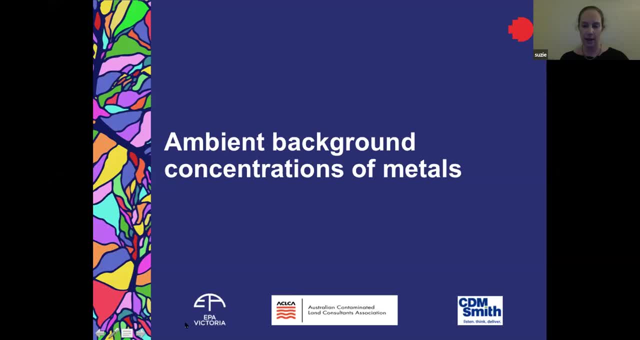 finished now, um, it was a collaboration between um, of course, rmit us and epa via their has waste fund, uh, the australian contaminated land consultants association, and then cdm smith came in at the end and helped us to get the database up that i'm going to talk. 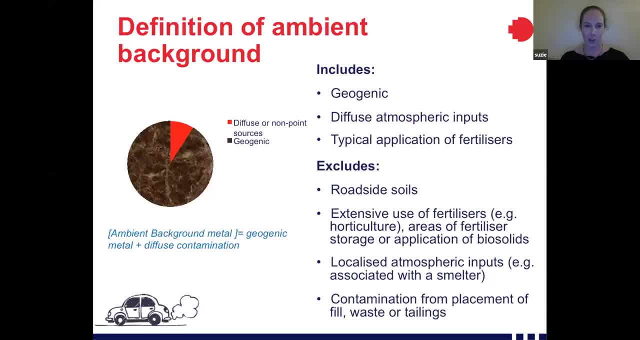 about um as we get towards the end of talking about our background concentrations project. so if you're um, not uh, you know too aware of what i mean by ambient background concentrations of metal. um, in soil we have um. there's the natural concentration, uh, or the geogenic concentration. 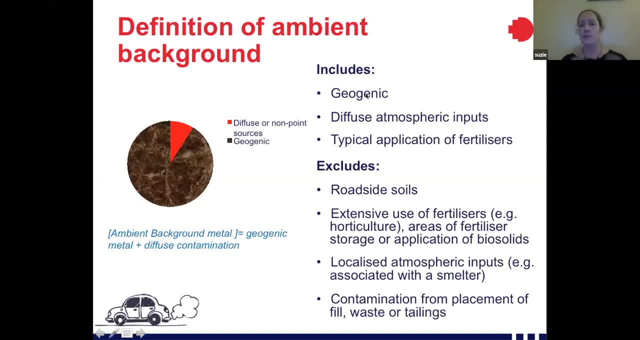 that comes from the soil, and then we have the natural concentration that comes from the soil, from the formation of the soil, and that is called technically, our background concentration. but we have this issue globally that we've been slowly covering the planet in pollutants and even if you go to the top of the himalayas, you can, um, or antarctica, you can measure, uh, our, our impact. 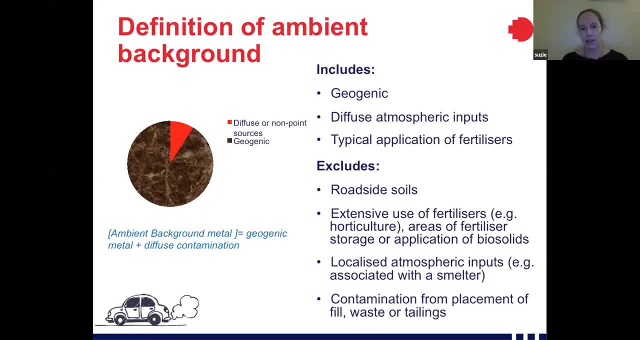 you can pick up that there's been an impact from humans, and so, um, we can't really, most of the time, get back to a true natural concentration in our soils, and so we use this term ambient background, so it includes the geogenic concentration, but it also we allow these diffuse atmospheric inputs. 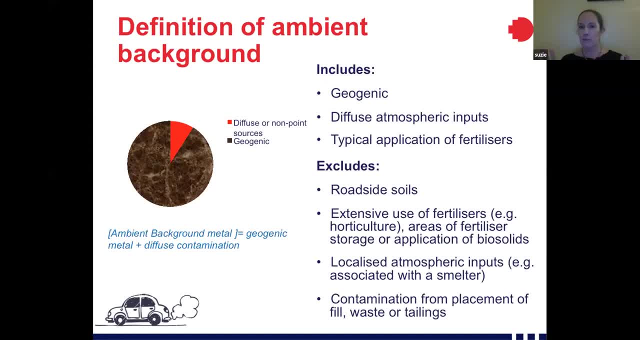 so where we have no idea what the um original pollutant source was, you know like we might. we might be able to do isotopic tests or something and work out it's probably from um fueling cars, but we have, we don't have any idea which cars and it's just basically blanketed the whole of. 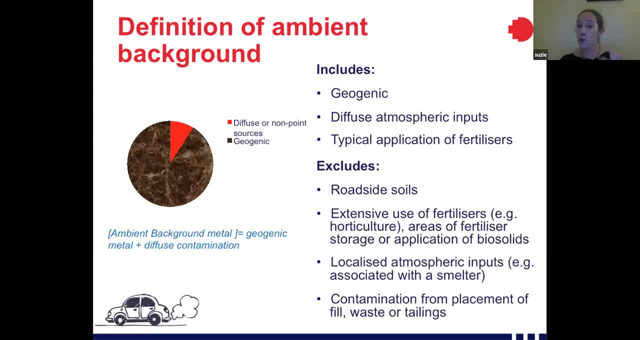 australia say: um, it's to some level and there are people working out what that diffuse atmospheric input of lead, for example, is at the moment. um, and it also comes from just a sort of typical application of fertilizers. we don't that's kind of quite widespread throughout a lot of our soils. 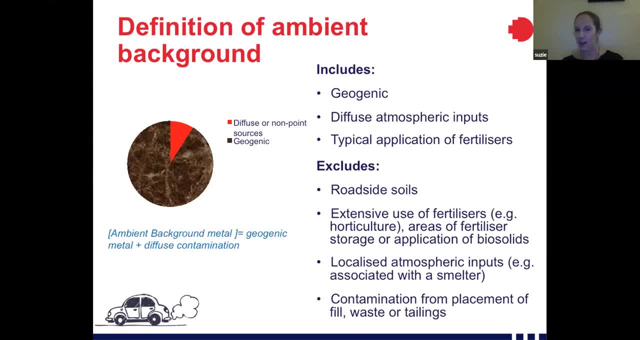 and also we're often using agricultural soils to give us an idea of background, and of course they've all had fertilizer on them. so we tend to allow a typical application, not, though, um extensive use of fertilizers, if you see down in the um exclusions. so not um agriculture like horticulture. 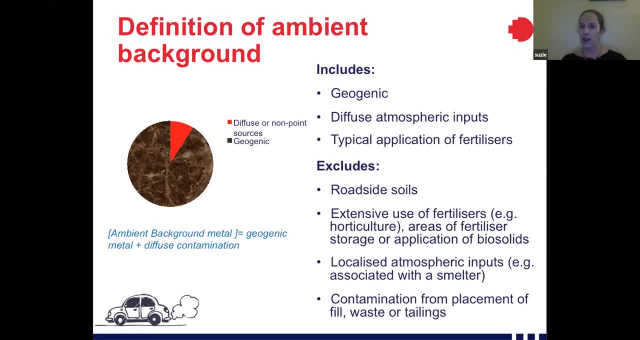 where it's really intense, more like a um, you know like a um. you know like a um. you know like a sort of broad scale pastures where you might have had the occasional addition of fertilizer. um, we also roadside soils are out, that, um, that's seen as more the effectively the roads are point. 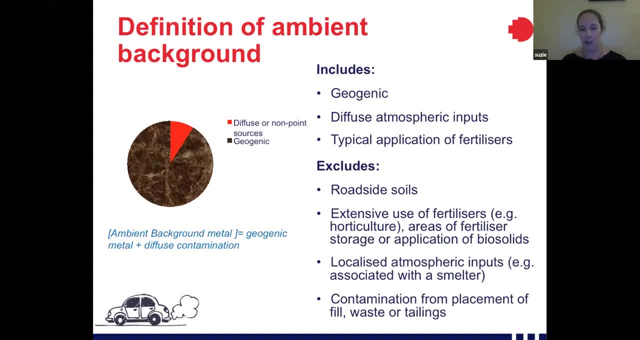 source next to them rather than something that's far away from roads, um any localized point sources and contamination from specifically placing fill or things that is not um that diffuse non-point source that we allow in the ambient part of ambient background, and so what you get for your? 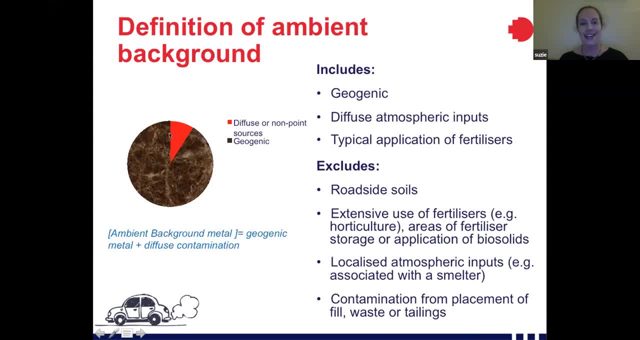 concentration over here is you have your geogenic point and then some small amount um, which we've actually probably exaggerated it's. it's probably a much smaller wedge than this. that's this diffuse, uh, non-point sources that we, we just really it's very hard to separate out, um, and so what you know. 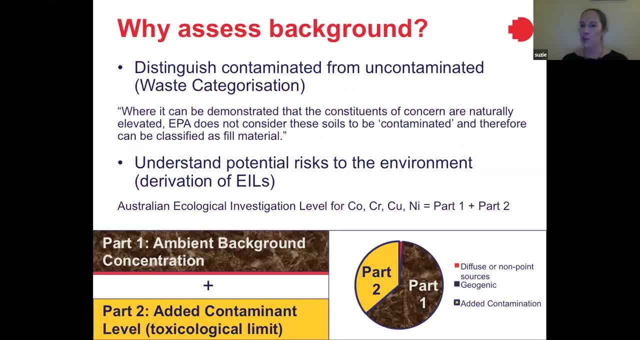 why are we interested in looking at this- natural concentrations- especially when you know i've told you that we do pollution and risk assessment from pollution. well, it's really important to be able to clarify where you're going. we're going to talk a little bit about the us um, and you can find 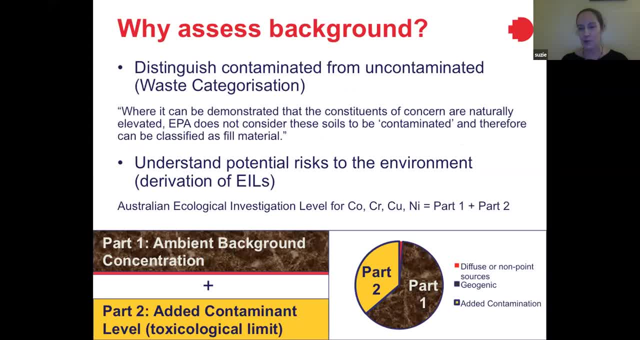 more information about that if you want to. but it's um, it's easy to do, but again, i think we have to stay with the science um on about what's getting produced, you know, um, but we've also we've included a lot of information that's available in the, in the map here in there. 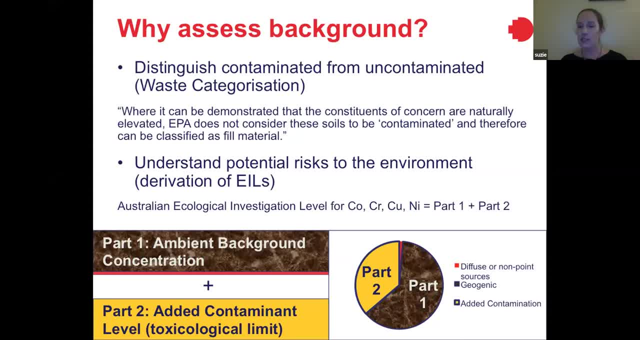 as well. so because i think you know what's definitely going to be being used in this space and the more you're able to use it, then the more opportunities you'll get- is for, um, what's that? you know what's your target for. so, again, we're not looking at anything. that's. 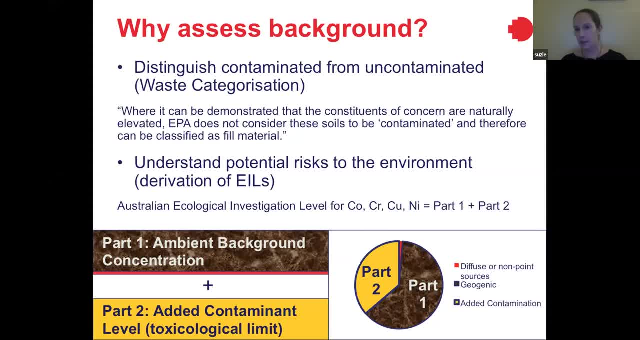 unsupported. if we're looking at whatever is that as an example of how the environment is going to be, It's likely to be highly bound to the soil and not be very bioavailable, not be very mobile And so in waste categorisation, if you can say that what your soil is is naturally elevated. 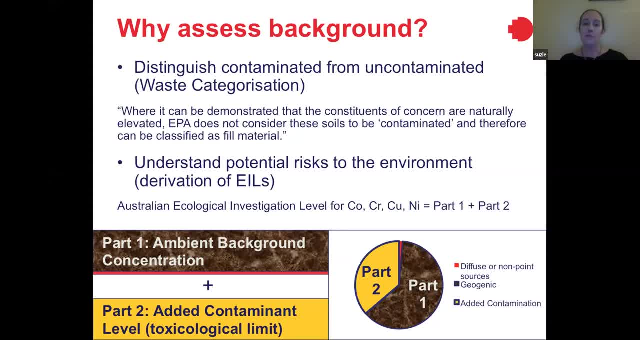 in arsenic or nickel, then you're allowed to treat it as clean fill. However, if that elevation is because of pollution, you then have to deal with it differently and pay to dispose of it or do risk assessments, et cetera. further risk assessment. 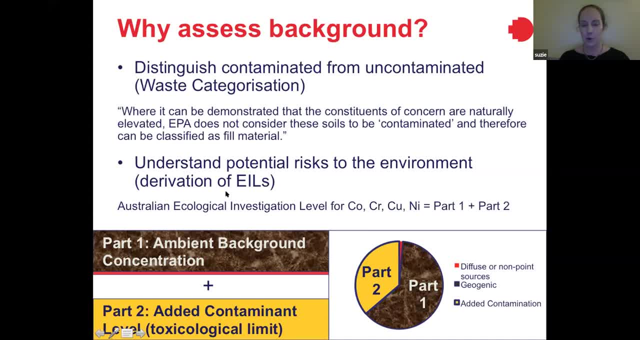 It's also in Australia. it's now very important for understanding the potential risks. In our NEPM, our National Environment Protection Measure, a number of chemicals and the list of them they're hoping will grow have two components to the ecological investigation. 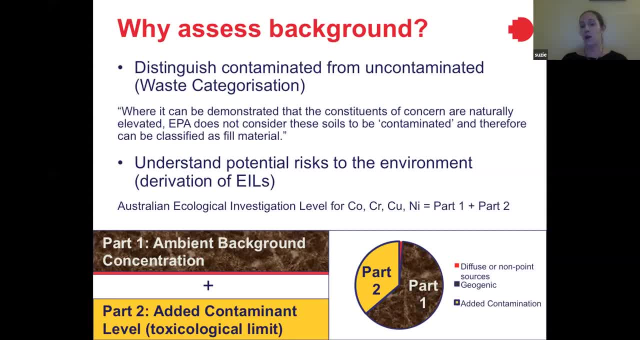 level, which is basically the soil quality guideline, above which you have to do further risk assessment, And so we're looking at that. What it includes is the first part- is this ambient background concentration, which we looked at as the brown parts, the natural part, and then we've got our tiny little bit. 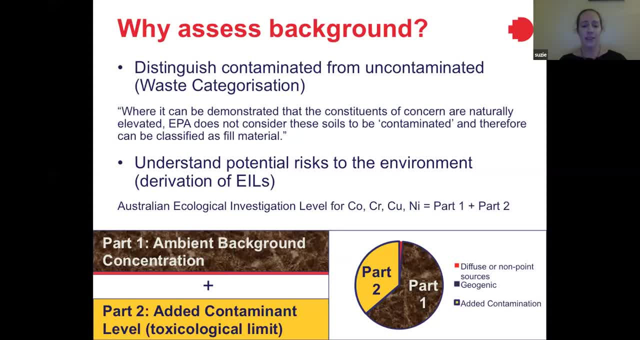 of our ambient part. And then there's the added contaminant level, which is your toxicological limit, And it's still the same concept that the natural part is very, very highly unbioavailable. And so you're really interested in what's added above it, mainly for your risk assessment. 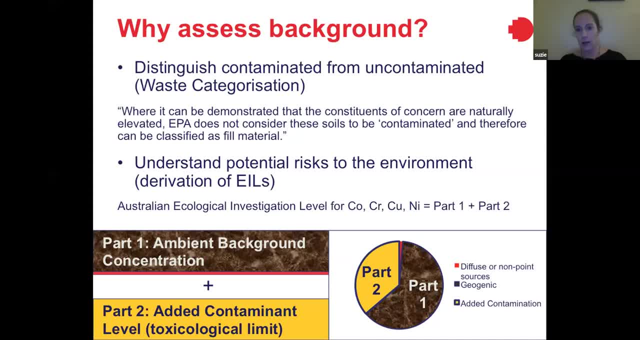 There are a few chemicals which they've said that doesn't hold. But it's the general idea underpinning the NEPM for ecological risk assessment. is this idea So for risk assessment of contaminated land in Australia? they're really interested in having ambient background metal concentrations. 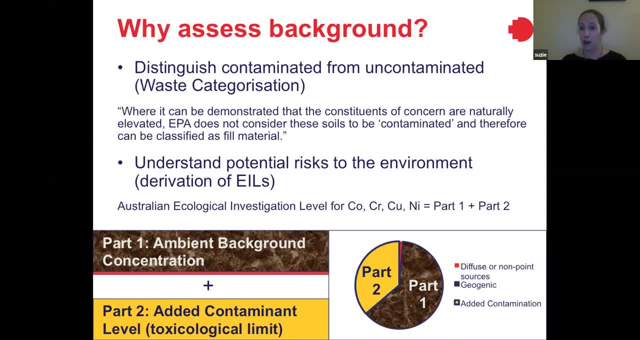 And we really didn't have very much in Australia when we started our project, And particularly in Victoria, the contaminated land industry were quite concerned that there were a number of- I don't know- There were a number of areas that weren't being picked up by the general guidance, where 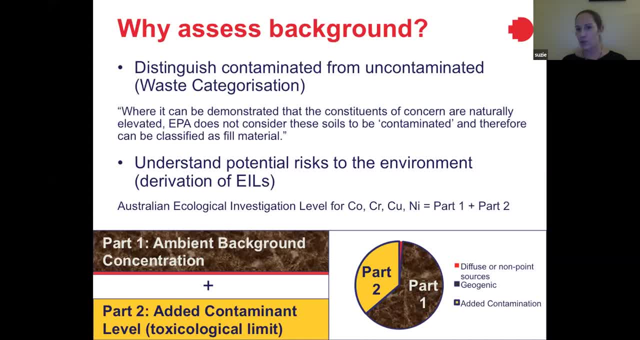 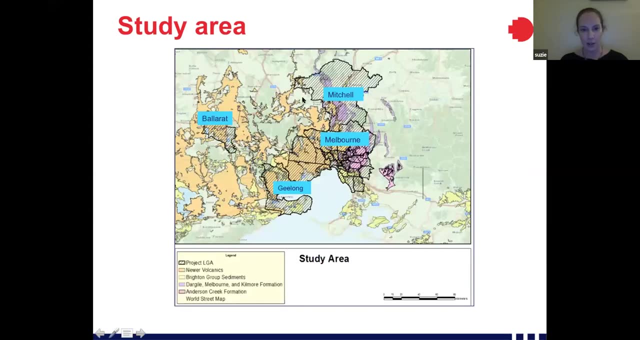 they knew from experience that Australian soils were. these soils were naturally elevated and enriched, but they couldn't demonstrate it, And so they wanted that information, and EPA was really keen to get that information too. So our study area, we looked at soils, all the grayed out areas. 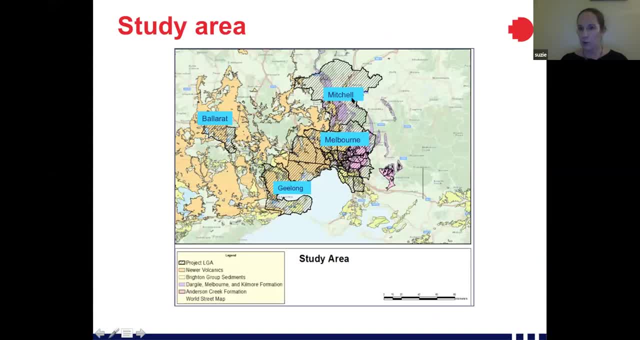 We looked at soils across Melbourne. Mitchell is an area that Melbourne's moving into, Geelong is an area of high industry, And then we looked at other areas. We looked at other areas, We looked at high industry and then also Ballarat. 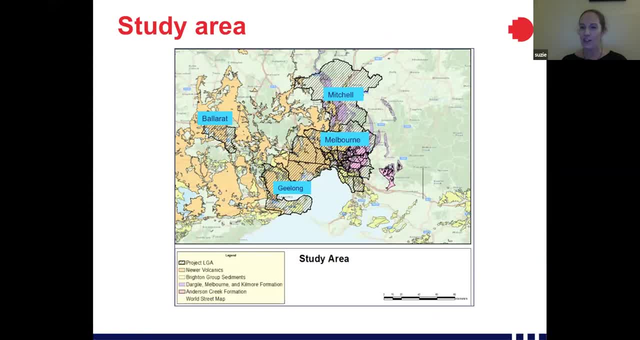 Although, interestingly, when we looked at it, they didn't want us to look at the traditional areas of Ballarat that are high in arsenic. They wanted us to look at the other areas which hadn't been looked at very much. Everyone knows those areas where the mining, the gold mining, has traditionally been a high 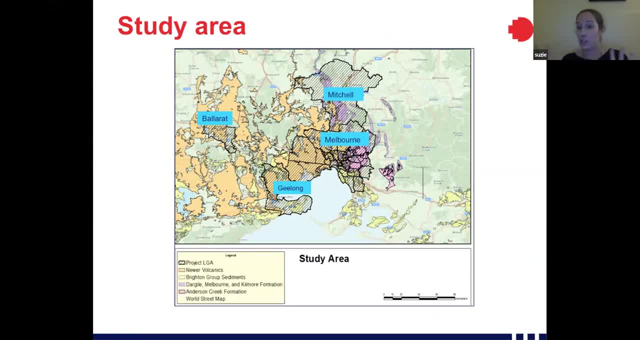 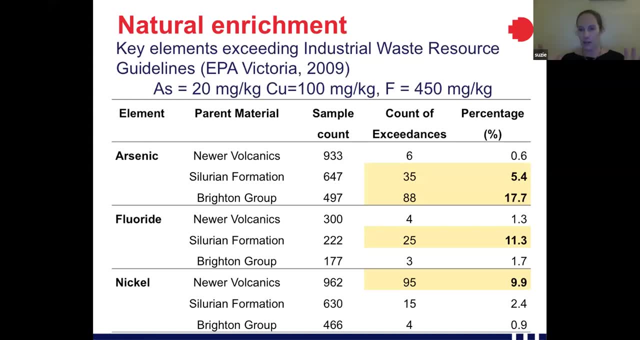 in arsenic and they didn't want us to look at that, So we didn't look at that part. That's not included when you look at the data and see the data. So this is just a real summary of The results that came out. 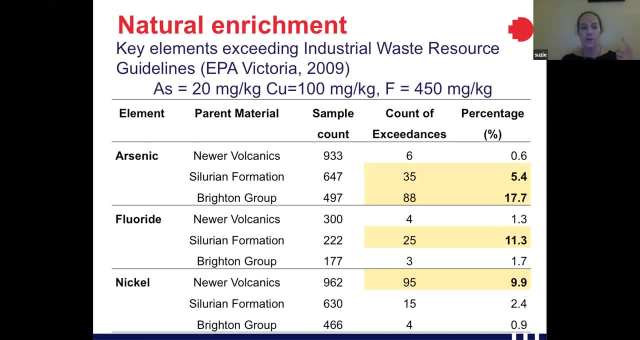 We found that arsenic, copper, fluoride and nickel were the elements that were the most likely, had the most incidences where they exceeded the industrial waste guidelines, which were the sort of cutoffs for whether or not you could treat the soil as clean fill. 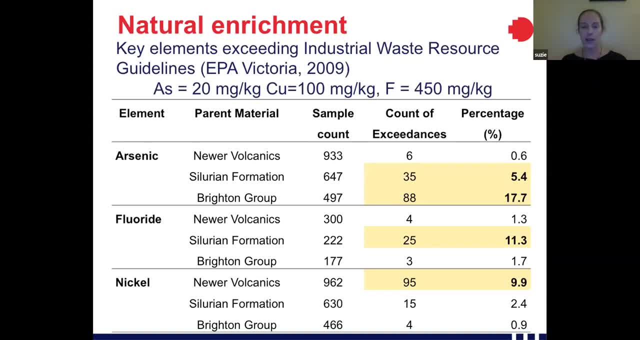 And we looked at it in a number of other ways too. but it's a pretty simple way to sort of look at it And I've got these what the values were at the top here, and I can no longer see my actual numbers on the side. 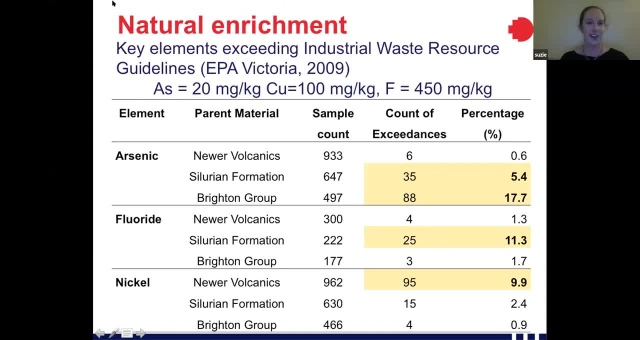 I'm just going to see if I can move this. Oh, I can. Oh, brilliant, Okay, I can talk to it now. Okay, So for arsenic we found in the Silurian Formation and Brighton Group, which Brighton Group is? 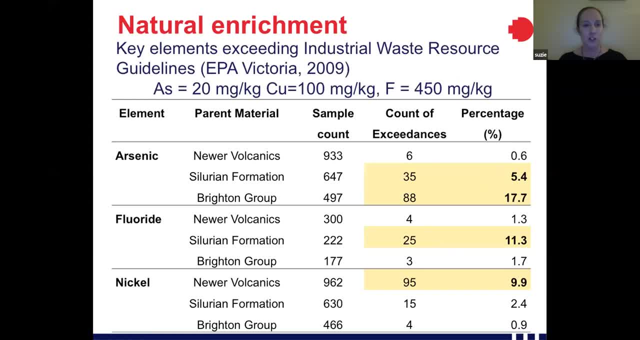 down around Brighton in Melbourne to give people from Melbourne an idea. Silurian Formation is more in the north of Melbourne. These are the, These are the, These are the parent materials, the geologies that soils were formed on, And so we had some issues, particularly Brighton Group, and Brighton Group was 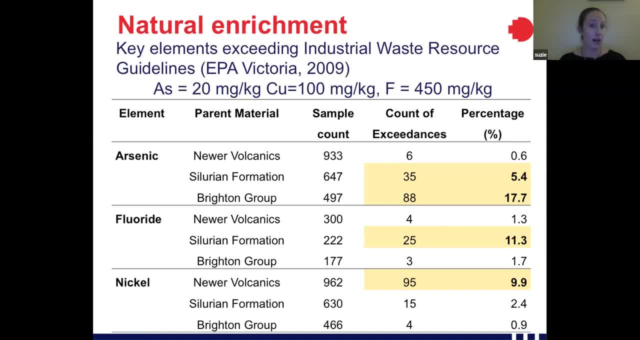 The industry knew that there were areas where it was high in arsenic, And so we had almost 20% in the Brighton Group of our samples, And I should say I'm not talking about detail, but we had this very rigorous way of sampling. 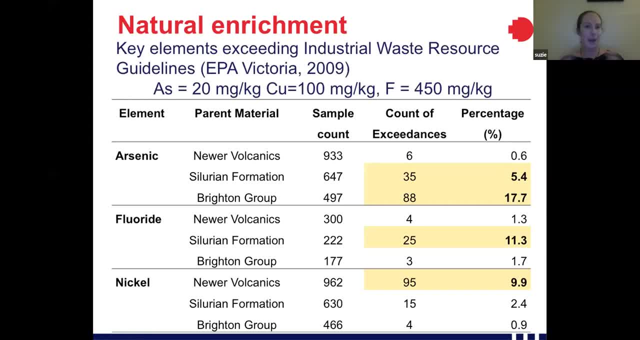 soils and making sure that we really were collecting ambient background soils. They had to be a certain distance from From roads, Couldn't be quite a long way away from any industry, et cetera. I'm not going to talk about that today because there's not time, but I will put up a paper. 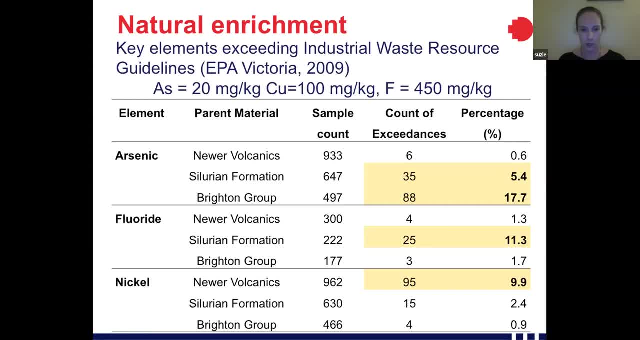 at the end where we went, We had a paper on the methodology that we used published And I should say this is the I'm presenting Hannah McConnan's PhD. She's finished now here. And then we also had fluoride, particularly in the Silurian Formation. 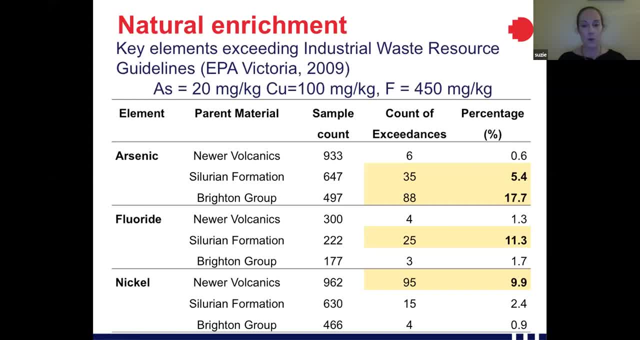 So this is in the north of Melbourne where we had a bit over 10%. And then we also had fluoride, particularly in the Silurian Formation. So this is in the north of Melbourne where we had a bit over 10%. 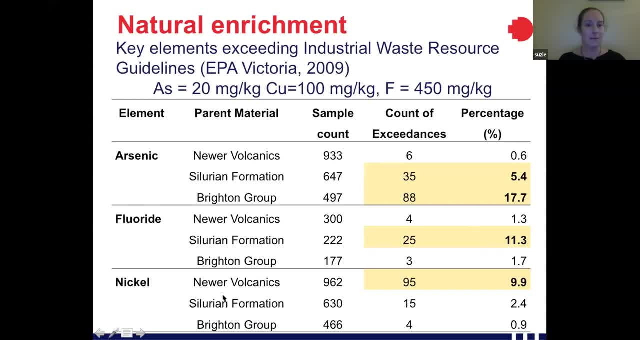 And then we also had fluoride, particularly in the Silurian Formation. So this is in the north of Melbourne where we had a bit over 10%, And then nickel again, And this was what we'd been told by industry to expect. 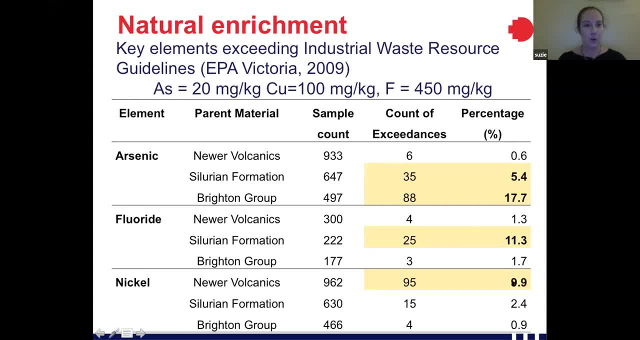 Nickel again around about 10% of samples in the newer volcanics- That's out in the west of Melbourne and continues right out through western Victoria- of volcanic soils, And the interesting thing was, though, even though we found, quite a few were high in nickel. 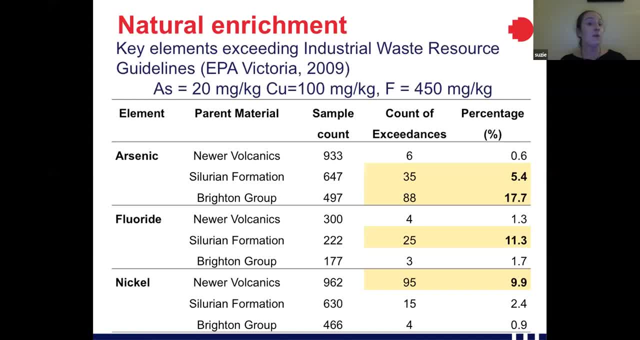 it was not to the levels that I know from when I was at EPA. some people in industry had been thinking So. when I was at EPA, there were people trying to pass soils up to about 400 ppm as nickel, as being natural. 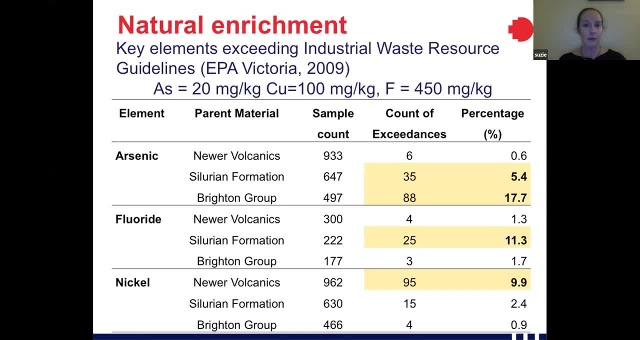 And in our research we didn't find much over 100.. Oh, and I didn't put the nickel level in. the nickel level is 60. So we got maybe up to about 120, about double, but not up around the 400 that previously. 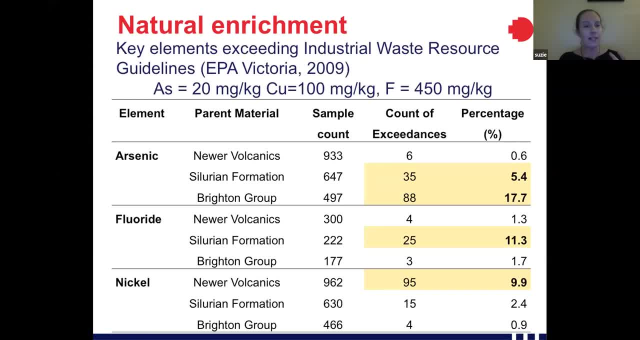 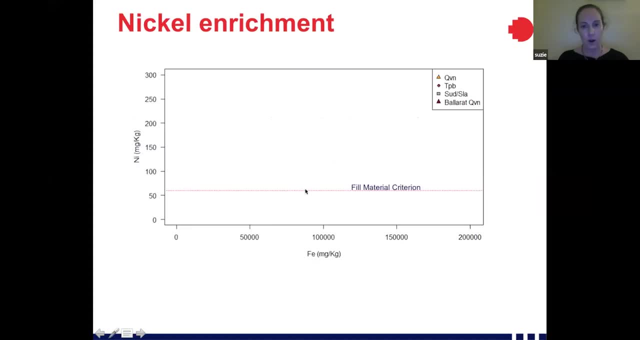 there'd been this case for. So it sort of confirmed what industry thought, But also kind of brought it back down to a bit more realistic values. Now I'm having trouble. oh, there we go, All right, And so just looking at some of the more detail that we looked at here, this is just nickel. 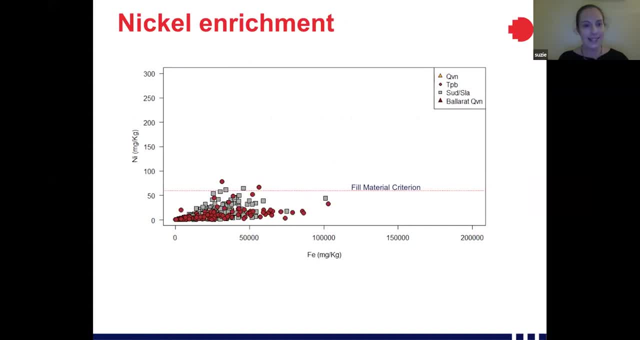 enrichment And different. this is in the different, different soil parent materials. So I just the grey is that north of Melbourne, The red is those Ballarat volcanic soils. The yellow is just the rest of the volcanic soils And what we found out was that you can see this sort of looks like there's two relationships. 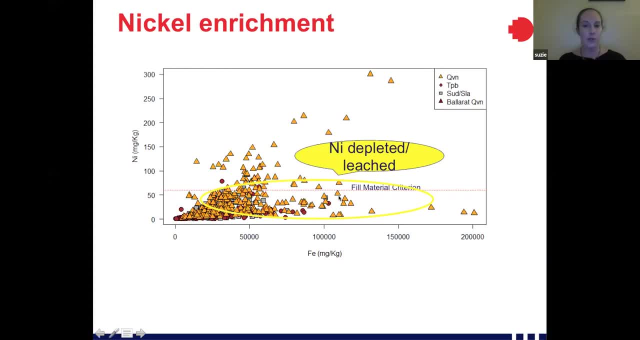 going on. We've got our bottom. one which we've we worked out was these were where nickel was quite heavily leached relative. these were much more weathered soils versus. oh, it's going off. What's happening? 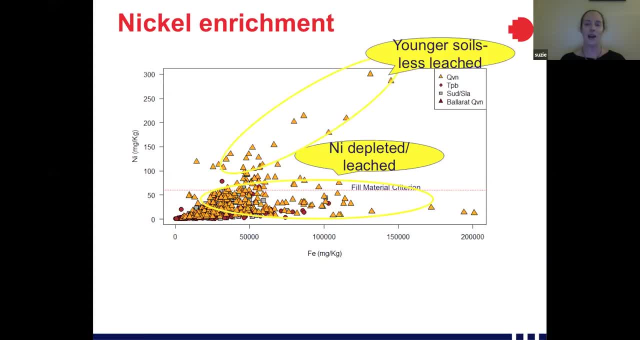 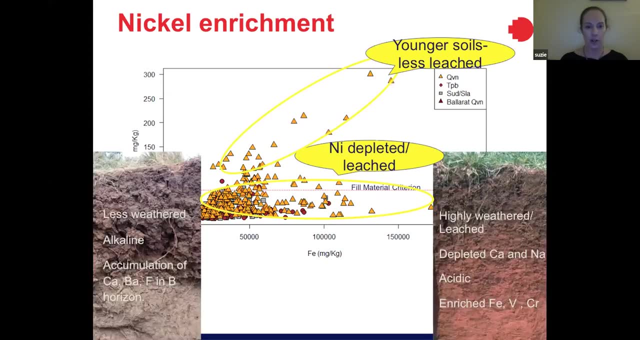 Something weird- Oh, I got it the wrong way- Versus our younger soils that were a lot less leached and had much higher concentration. So we had two relationships going on And you can see here there's an example of the younger soils on the left and these more. 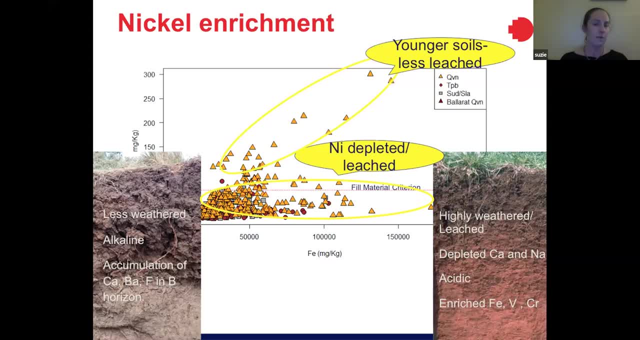 highly weathered, leached soils, And you can see they look quite different, even though they're on the same, developed out of the same geology underlying parent material, And so what we ended up doing? Nickel was the one that was the most weathered. 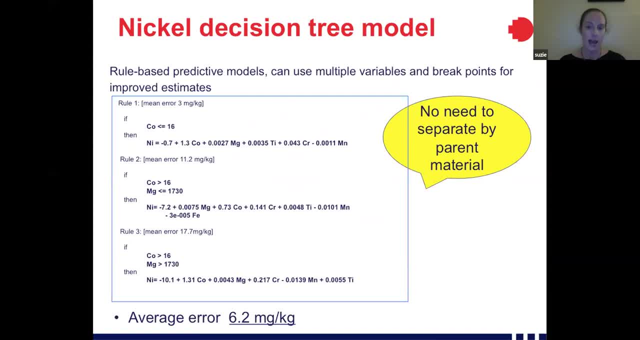 It was the one that was the most weathered, And so what we did was we did some decision tree modelling with it, And so you could have one relationship, but depending. it didn't matter whether your soils were leached or not. you could work through this decision model and industry could come. 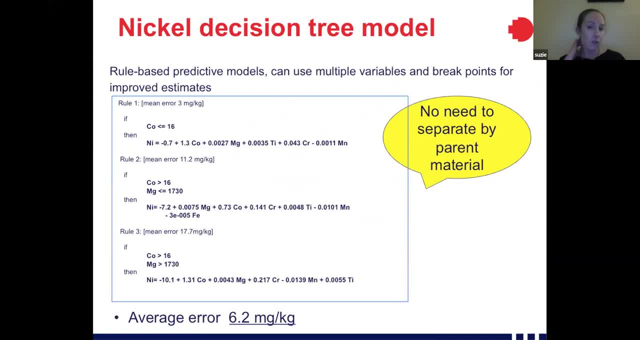 up with. they could predict from other metals that they were measuring anyway, whether or not the nickel in their soil was likely to be from contamination or whether it was likely to be natural for any given site, And we had an average error of plus or minus 6.2 milligrams per kilogram of nickel using 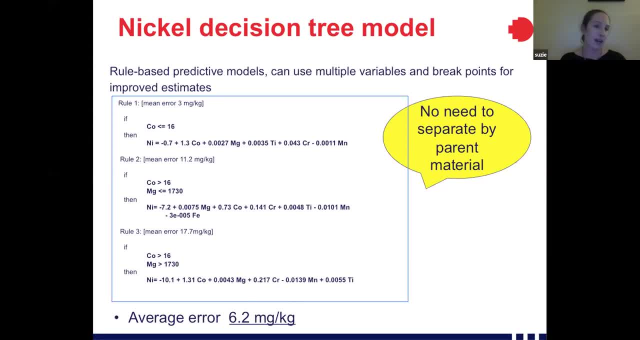 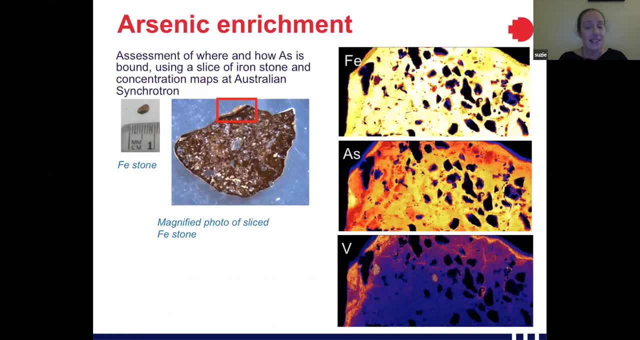 this decision tree, which is just amazing. when you're talking, you know. nickel, up around a hundred, is where you're interested in working out whether it's natural or whether it's contamination Arsenic. we went and did some research at the synchrotron, particularly interested in 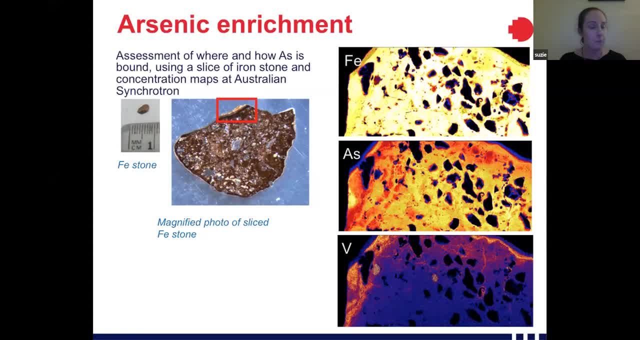 those brightened sands. So the the down around the south of Melbourne where we had high arsenic, We found a lot of arsenic. A lot of it was connected with these iron stones that were very high in arsenic And we you can see here this red. here is what's the, the results here. 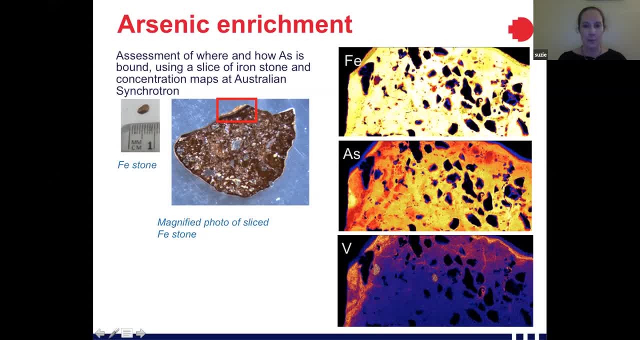 And it had ironed throughout- except these little bits that are these ones here- that we didn't fully work out what they were because there was a bit out of scope. But you can see the arsenic is mainly in the middle of the iron stones. 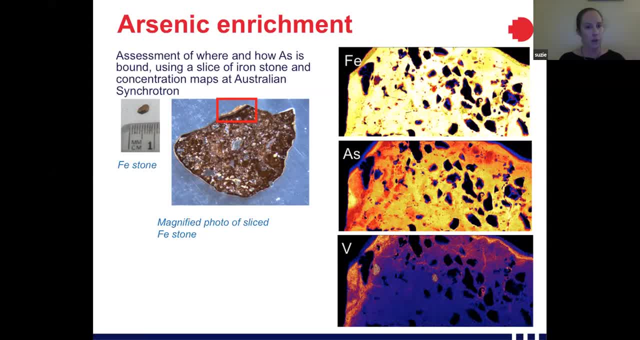 And we also had very high vanadium in these, not throughout the whole soil, but in these little stones And but the vanadium was really high more around the outside, And so it seems like we've had two different when the arsenic was forming around these. 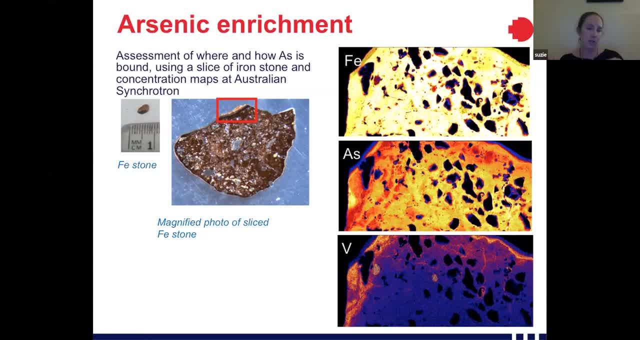 iron stones was a different period of time with different environmental conditions, to when they became high in vanadium. And Here we go: arsenic throughout the iron stone up to 7,000 milligrams per kilogram, So massive when you consider that 20 is the level at which you have to consider it contaminated. 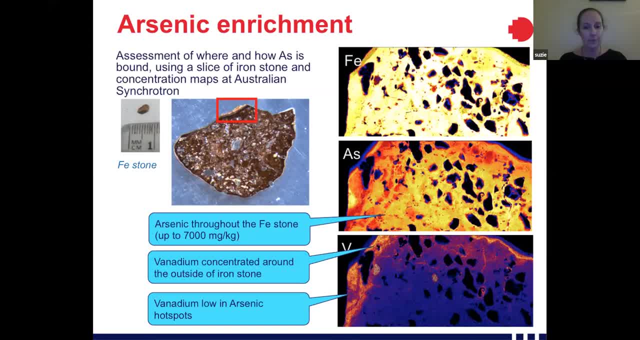 but this is natural arsenic And, and and then also the vanadium there And we think that it's come what the the arsenics come from. our sort of conceptual model of where it's come from is there's an area just outside of Melbourne. 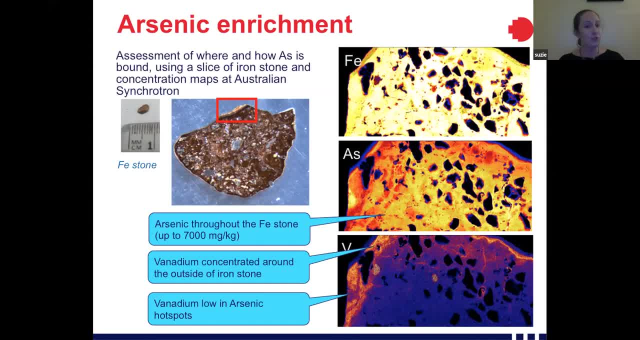 Where A gold mining area and gold is often naturally co-occurs with arsenic And we think over time there's been a movement of arsenic and a leaching and mobility of arsenic in closer to the coast And it's built up in those coastal soils there. 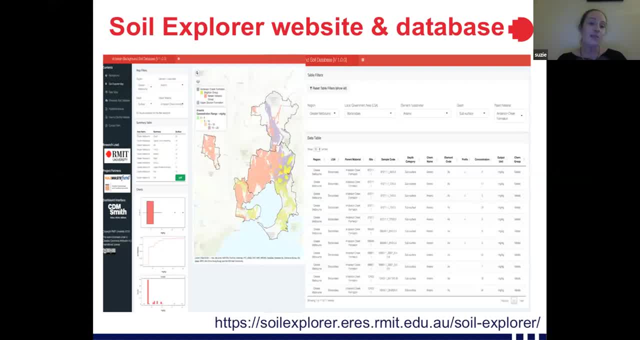 That's where we think that it's come from. Okay, So out of this it was. it was definitely. this was a very industry collaborative Project And I think we have Phil Sinclair in the audience tonight and and Phil was part of our advisory. 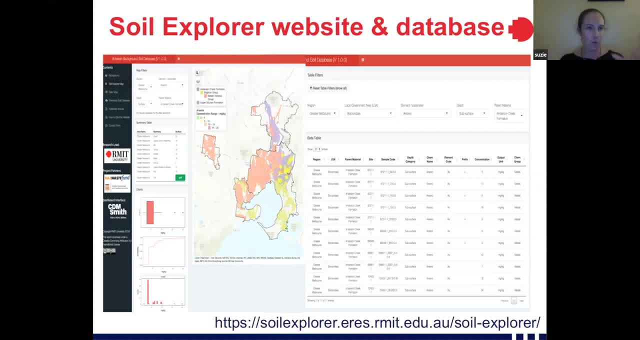 Sort of committee on this. at different times We had some workshops with groups of people. you know. are we on the right track? Can you use this data? And one of the outcomes from this project was our soil Explorer website and database, And it's. it's up now if people want to go and have a look at it afterwards. 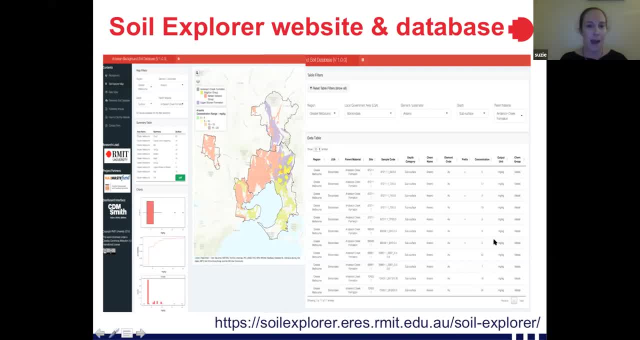 And it's it's a great big database. We've got a map of the site. You can type in particular Areas of Melbourne and get up the arsenic. You can also get Things like: the typical pH is that we found? or soil, organic matter, the cation exchange. 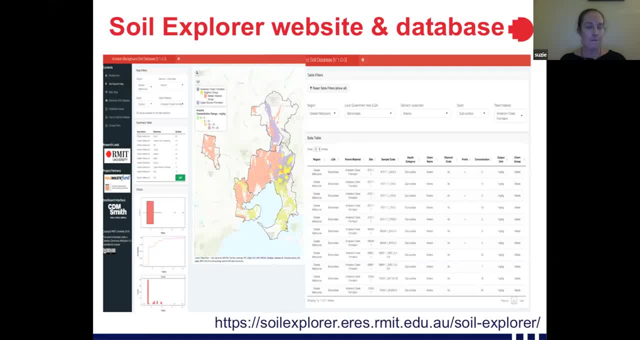 capacity as well. So it's whole range of metals, But also some of those other factors that can help you, And you can then compare that to where your site is and see what's. you know, what's around your site and what the issues are likely to be. 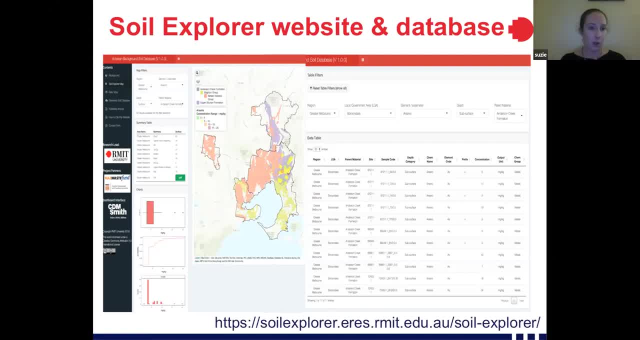 You can download the database and use it in your own modeling. It's all open source And that's. it's been downloaded. I haven't looked at it recently. It was on my list of resources. It was on my list of things to do tonight. 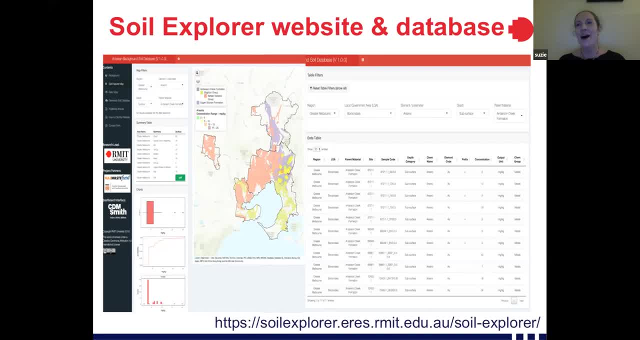 And I didn't end up doing it before I got here. But we've had multiple thousand people go and use this soil Explorer website as far away as America, which is fantastic, but many, of course, mostly in Victoria and mostly, and then quite a few in the rest of Australia as well. 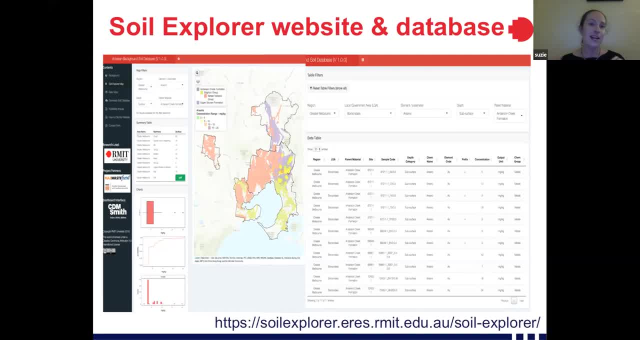 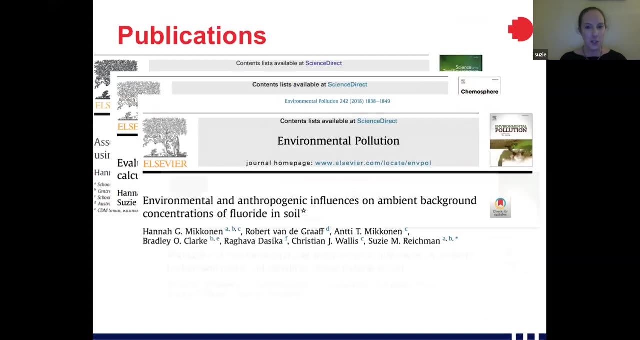 And I am talking to a range of people about possibly repeating some of these studies and doing different versions in other States, Because It seems, like Victoria, we have a lot of information on this. So we have a number of publications that have come out of this study that have been used. 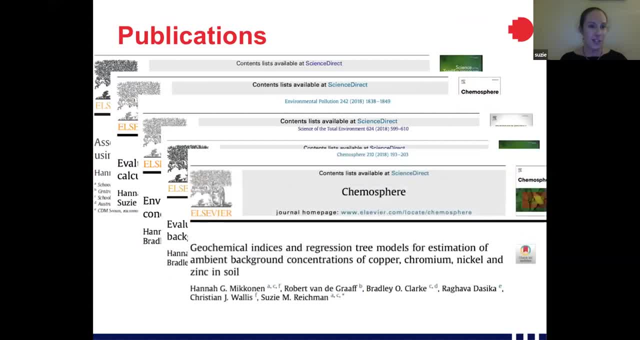 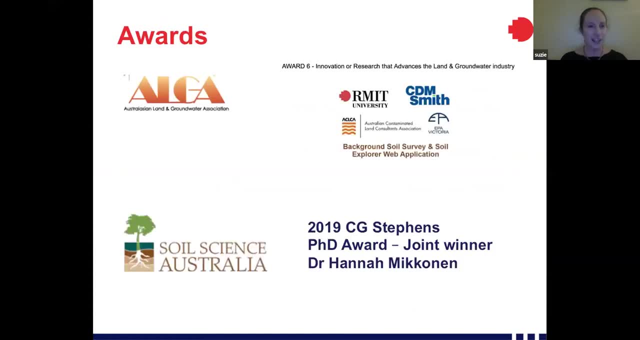 by industry. If you want any of these, if you're interested, please, you know, get in contact with me afterwards and I'm happy to send them. Hannah did a fantastic job of this project, with this project, and we ended up winning. 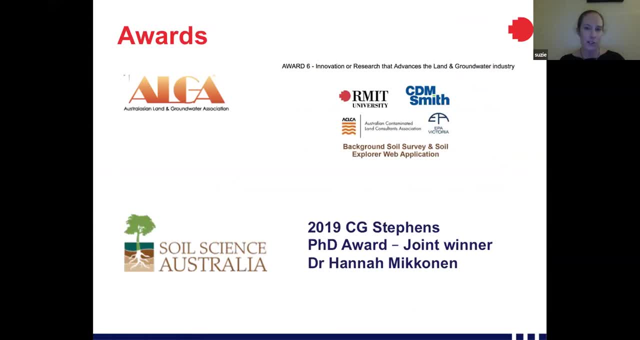 as a team. The Australian land and groundwater association Innovation Research Award Last year- And Hannah had just found out- has won the 2019 CJ Stevens award. She was a joint winner of that. They had two people winning this year. 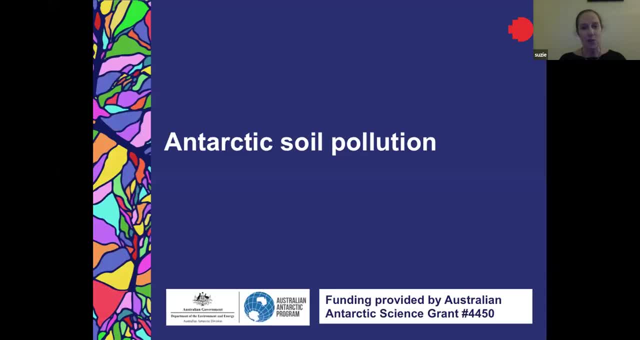 Okay, So final topic, we can talk a bit about our Antarctic soil pollution project, and this is funded by an Australian Antarctic science grant and beginning of last year we all got to go down, or the group, myself and the two students. We all got to go down. 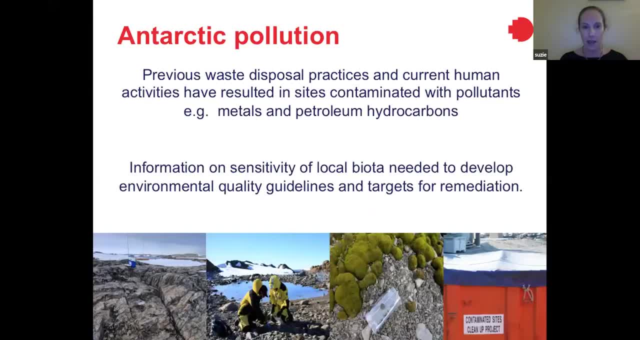 We got to go down to Antarctica, which was just an amazing experience, And people normally think of Antarctica is pretty pristine, but of course, where we've got human bases in the past, we didn't necessarily dispose of our waste like we should have. 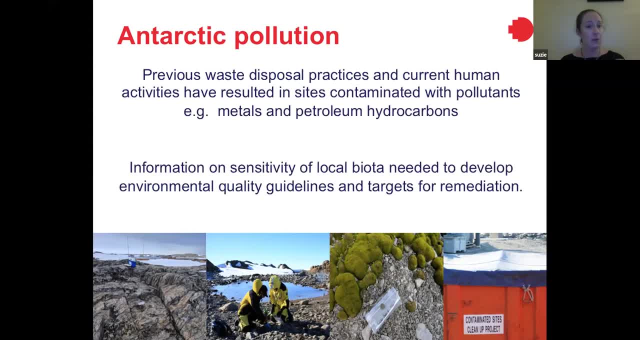 And they still have spills and things happening every so often. So around our wastes- sorry, around our bases- there are some significant contamination issues And they want to work out guidelines both for risk assessment And for mediation that are based on the biota. 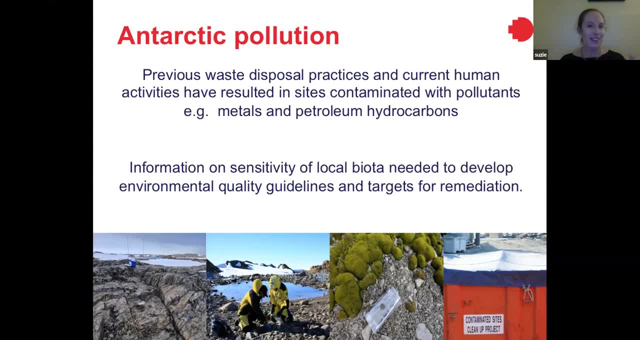 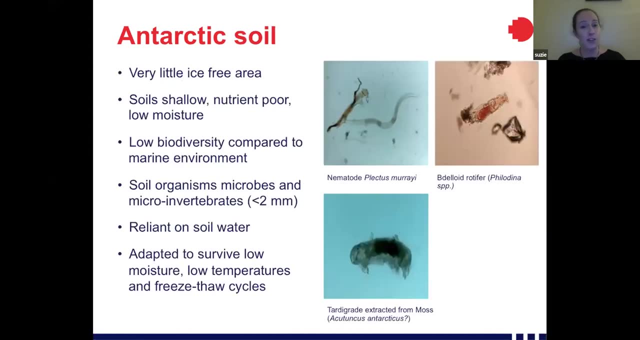 So they've been doing work on Marine- you know we all think about the seals and the penguins and things like that- for a number of years. but they really wanted to get some of the soil, biota, the terrestrial biota And so Antarctic soil. there's not very much of it, but of course we tend to put our bases. 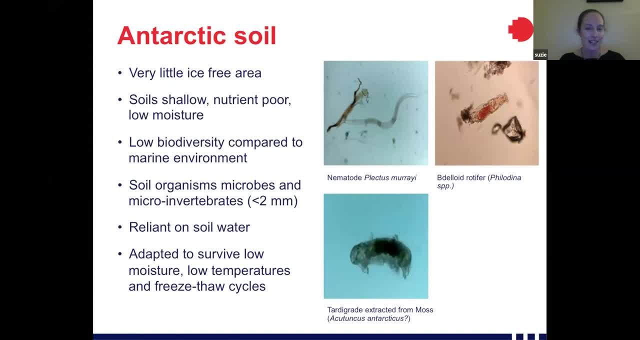 where it is, So it tends to be quite highly inundated, Yeah, And they tend to be impacted. They tend to be shallow, nutrient poor and most of the time, low in moisture, although you can get localised areas where they're quite damp. 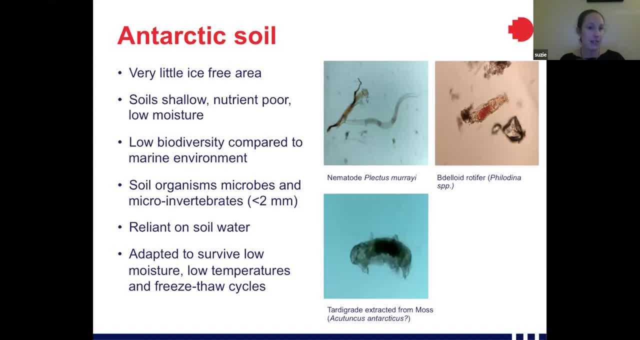 And they have much lower biodiversity when you compare to the Marine environment And it's dominated by microbes, which there's a group at University of New South Wales looking at- Excuse me, I just need to grab a tissue. A group at the University of New South Wales looking at. 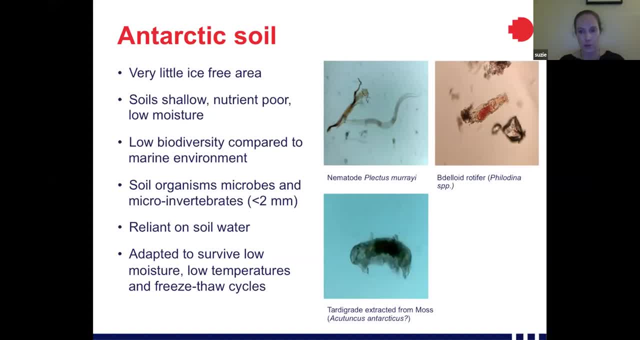 And we're doing the soil microinvertebrates, And so I've got the three main sort of species that have been investigated, So nematodes, rotifers and then tardigrades, And they're all relying on soil water, So we often we call them limnoterrestrial. 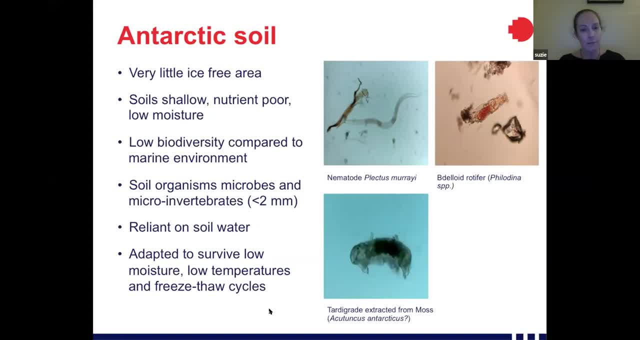 So they're terrestrial, but they're reliant on water And they're adapted to survive in these low moisture, low temperature, freeze, thaw cycle sort of environments. But we don't, we have no idea of their tolerance to pollutants, And so I've got a little video. 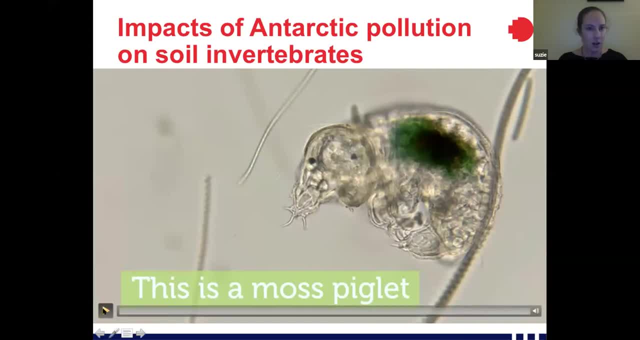 Hopefully this worked when I we did a video of our tardigrades- because they're so cute- with RMIT media people And I'm just going to show that to you now. Whoops, What's happening here? Here we go And try and show that video. 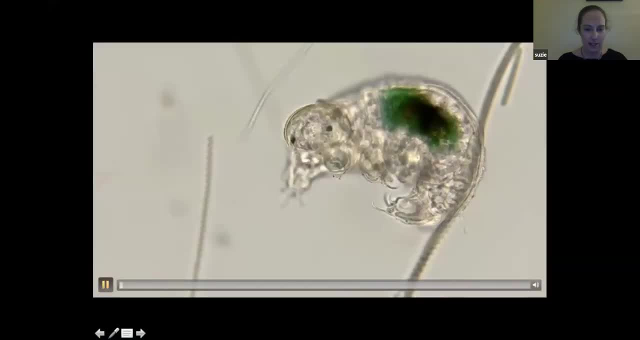 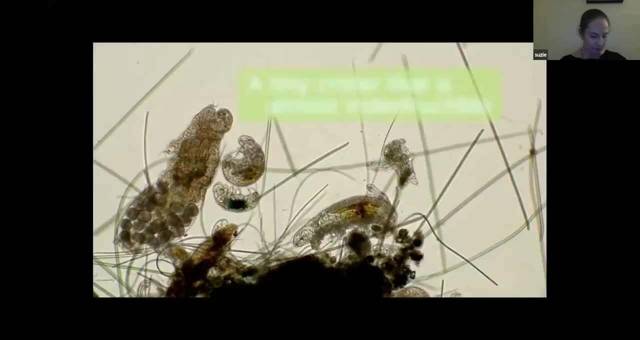 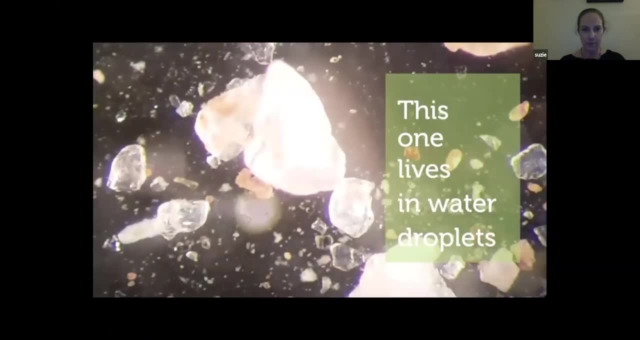 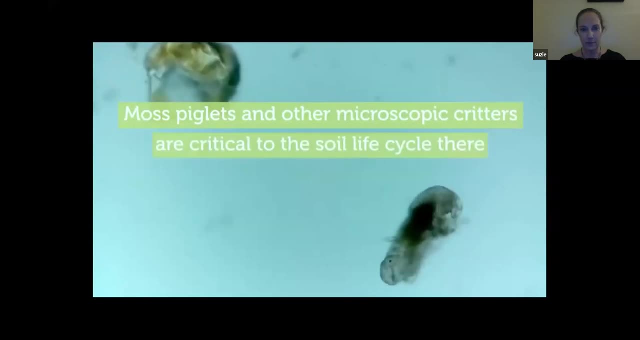 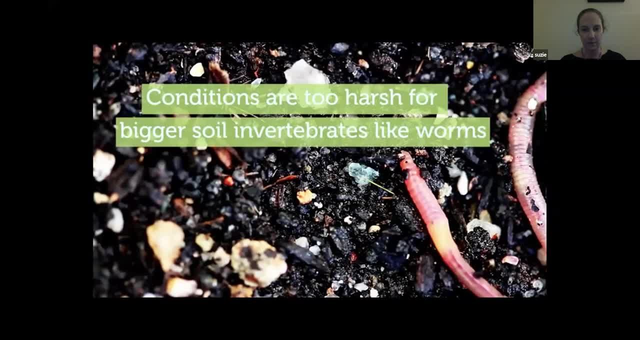 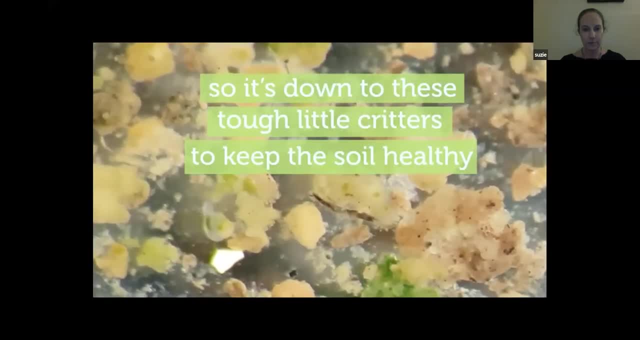 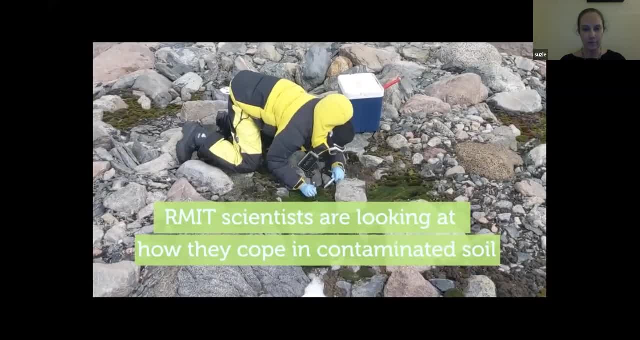 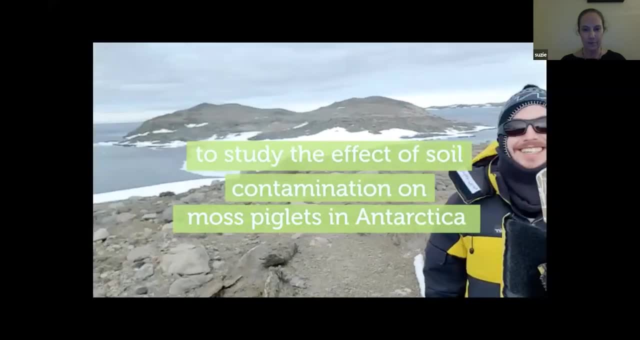 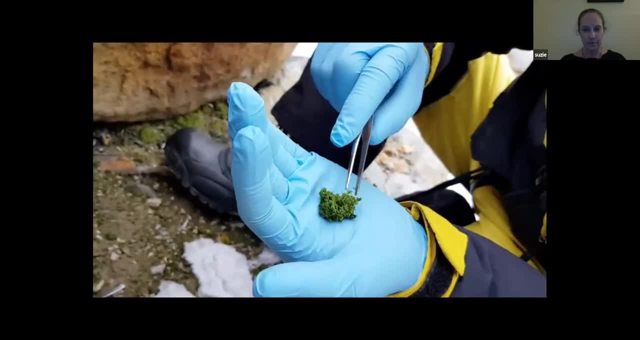 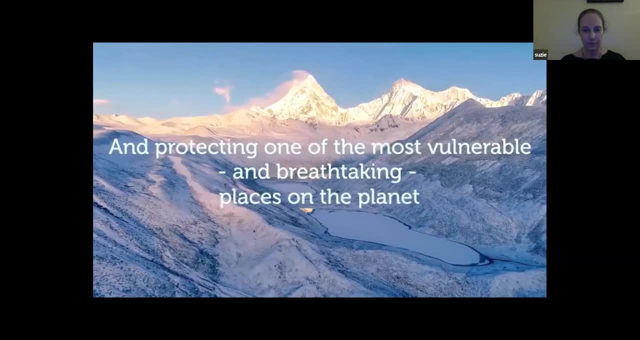 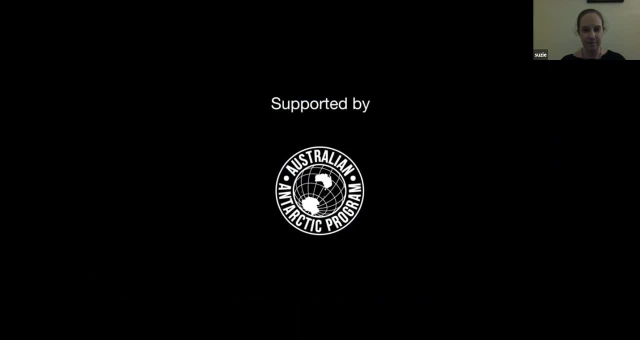 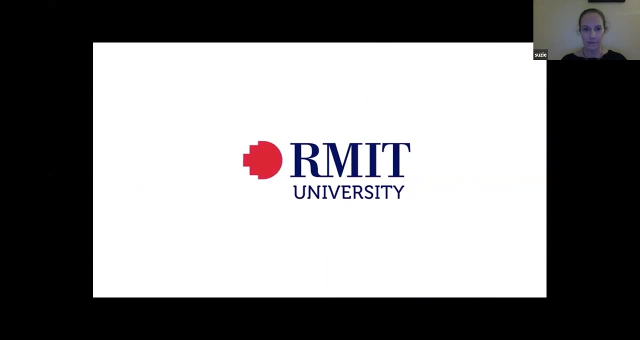 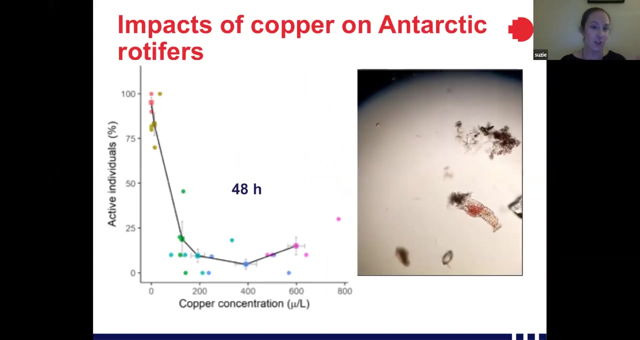 Here we go, Here we go. Okay, so that's so. it's pretty cool. basically, I think it's amazing that we're getting the opportunity to go to Antarctica and come back and do the research on these little Antarctic critters. 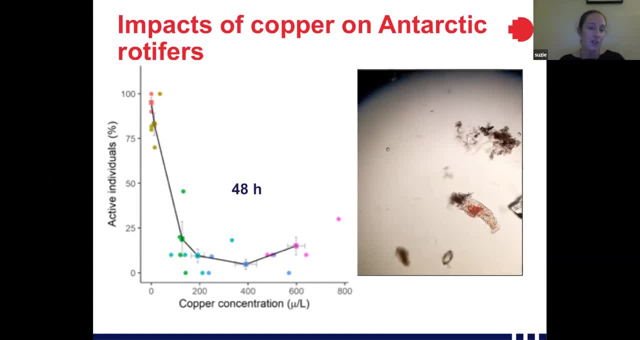 The two people in the video were Jordan McCarthy, whose research I'm presenting tonight. He's focusing on the metals, And then Steph Wallace-Polly, who is focusing on hydrocarbon contamination, And she's just starting to get results now, whereas Jordan 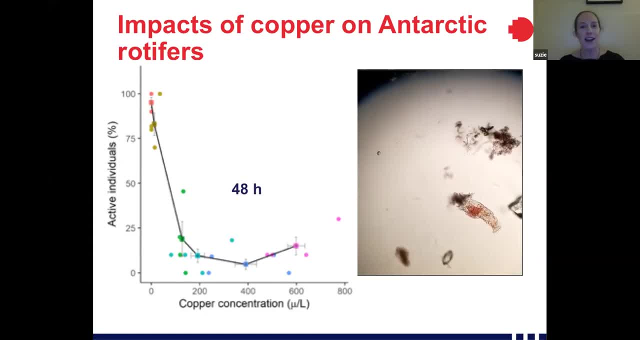 we've got a few results, And I'm just going to talk about our copper ones on rotifers today. So you can see a little video down here of a rotifer moving around And our ecotoxal, his ecotoxal. 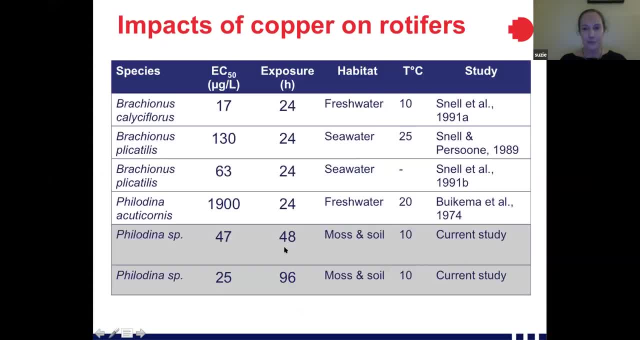 his ecological study on copper. to give some context here, We have some other research that's been done on rotifers We had. there hasn't been any research looking at the toxicity of terrestrial rotifers to copper. We've only got some ones in various aquatic environments to compare to. 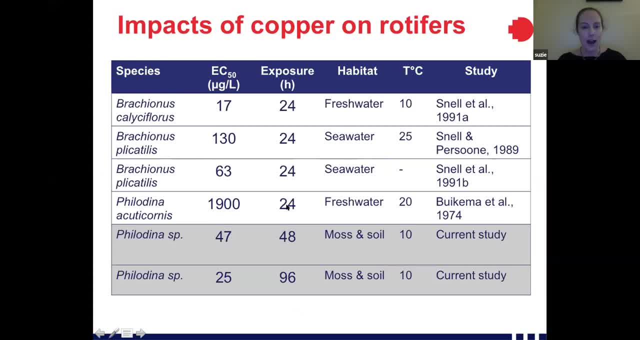 But what you can see is where it's looking like these Antarctic species, the philodena species that we're looking at and we're still in the process. if we hadn't been in shutdown, we'd have the species name now, but at the moment 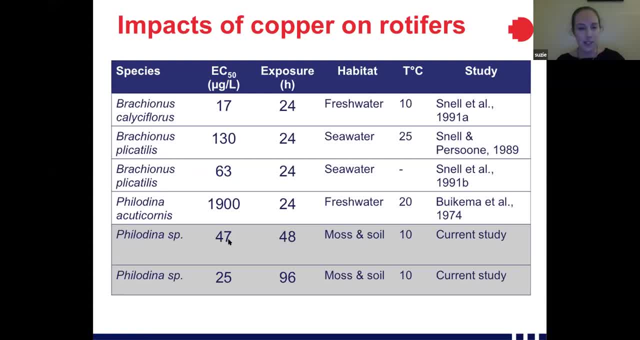 we've only got the genus. It looks like these Antarctic species. this Antarctic species is down, down towards the more sensitive end of things, And so it's really good. You know, the first indications are that it's really good that the Australian 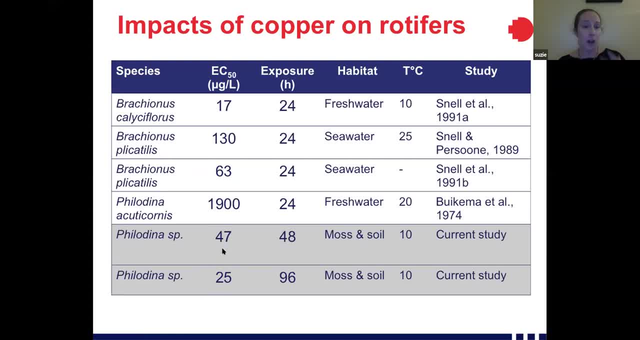 Antarctic division wants to do these guidelines based on the fact that they're going to be used in the future. So it's really good that the Australian Antarctic division wants to do these guidelines, based on the fact that they're going to be used in the future. 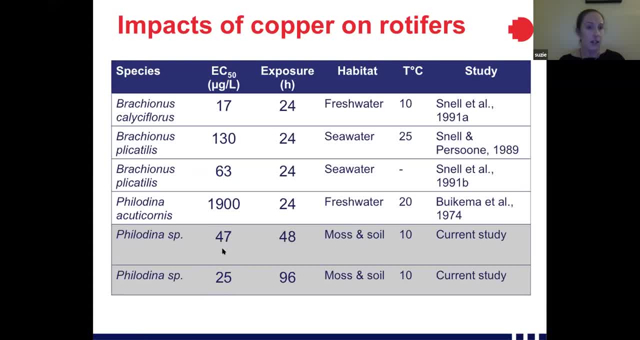 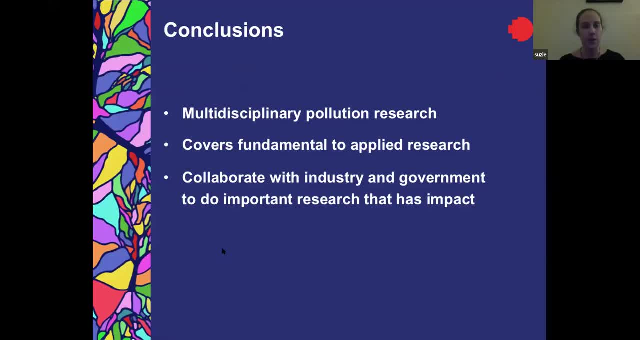 Antarctic species, rather than, for example, just bringing you in our Australian guidelines that we have, because they do appear to be down the more tolerant end, at least for copper so far. So just to conclude, we do really multidisciplinary pollution research. 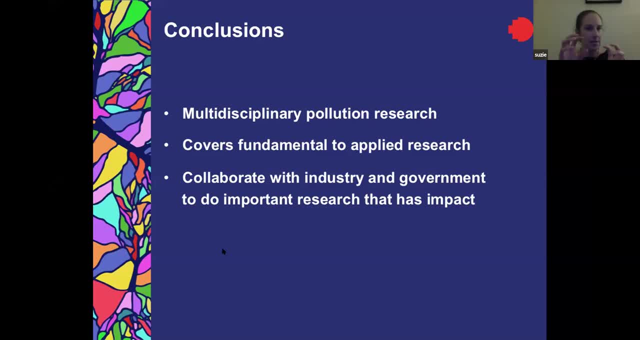 I think really, if you're in the pollution space, you need to be moving within those different areas and incorporating chemistry but also the biology, and then bringing that around to the risk assessment. We're doing everything from fundamental up to very applied research. 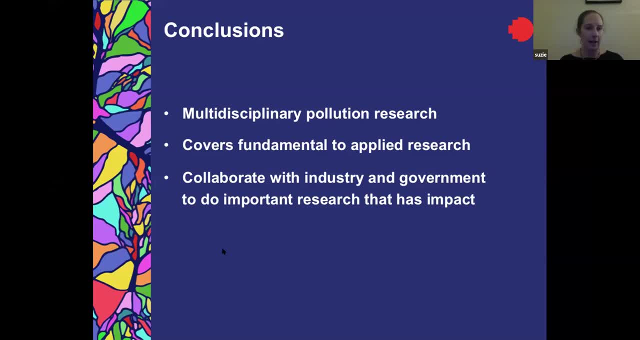 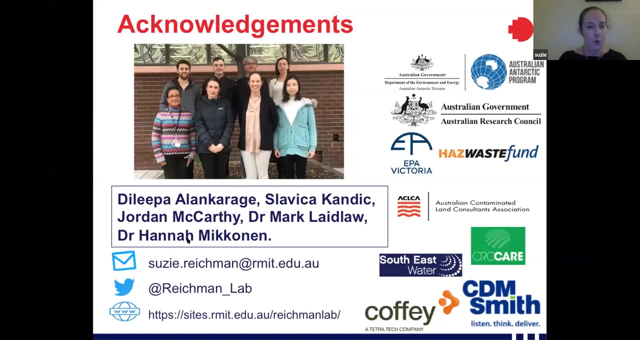 applied research, where we're collaborating with industry and government to do that sort of research that really has impact and where it's ending up, you know, really being used. And so I've listed here all the people's research who I've been talking about tonight. Here's the team you can see. 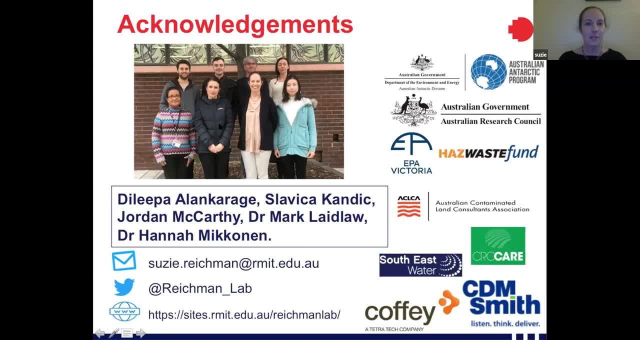 Justin there and Du Nguyen, who are going to talk, Slavica, whose research I talked about, Jordan and Steph, who did the Antarctic researchwhoopsa, number of our collaborators, including the ones from tonight, and then just some contact details if anyone's interested in getting in contact with me later, And 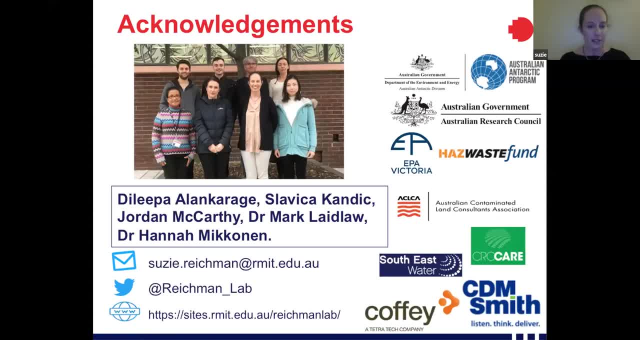 I think now we're going to goI'm going to stop sharing my screen and we're going to move across to Du Nguyen is our second speaker, so I'm going to give her the microphone and let her talk, going to stop my share and enable Juin a little bit of time to get hers up, and I'll just tell you. 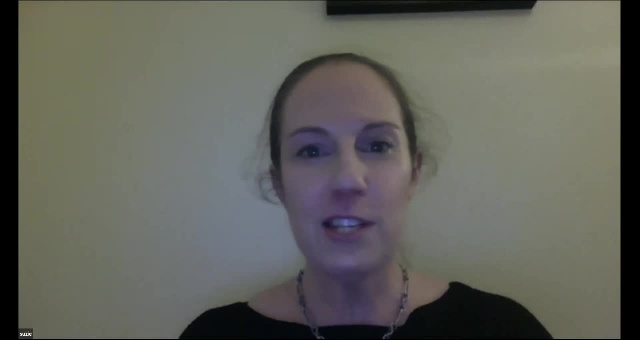 very quickly about Juin's PhD. So this is: Juin is going to be presenting some of the research from her first experiment that she's done and she's looking at platinum growth, platinum group elements from vehicle emissions, and then we use platinum group elements and catalytic converters, which 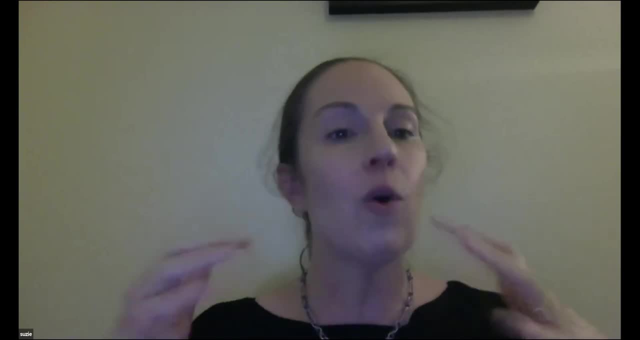 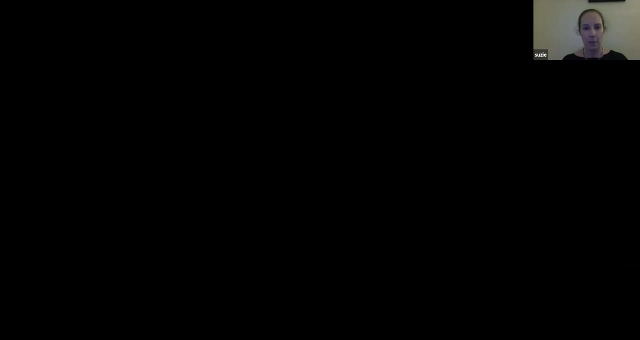 she'll talk about, and we're seeing growing concentrations of these pges in roadside soils and so she's investigating the chemistry of what's happening in these soils and also going to look a little bit at the toxicity of these platinum group elements, and it looks like she's starting. 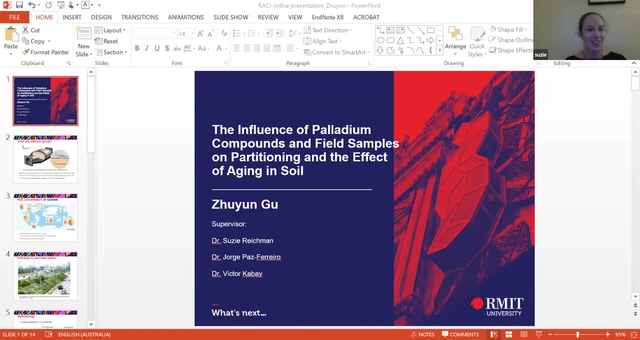 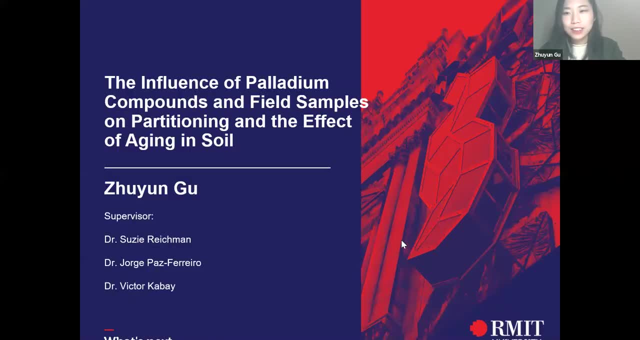 to share her screen, so I'll now hand over to Juin. Thank you, Juin. Can you all hear me clearly? I can hear you. Okay, cool, yeah, all right, and hello everyone. I'm Juin and thank you for coming here and hear my presentation, and today I'm going to talk about the influence of 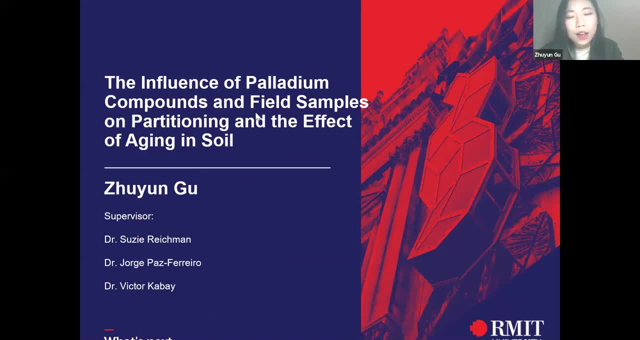 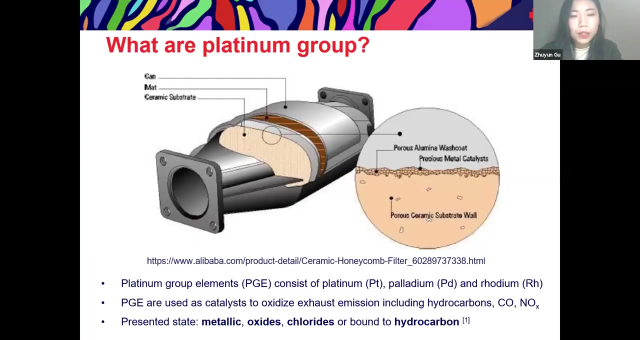 palladium compounds and few examples on partitioning and the effect of aging in soil. So first, before I get into my research topic, let's first discuss a few questions. So what palladium is used for and why do we investigate them? So palladium is one of the metal group called platinum group, which consists of platinum palladium. 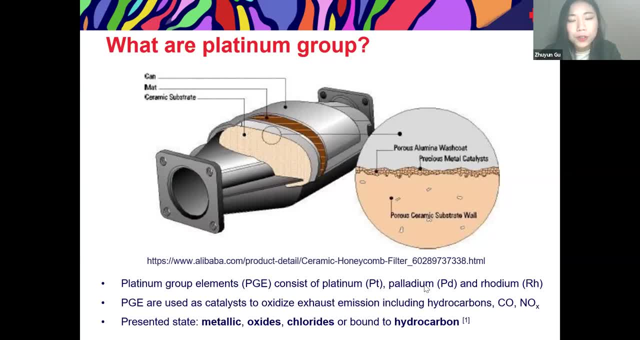 and rhodium, and they are mainly used in auto catalyst. This picture shows catalytic converters, and here the orange part is the ceramic substrate, So the platinum group is dispersed as a layer of wash coat on the substrate, so and they are mainly used to oxidize exhaust emissions, including. 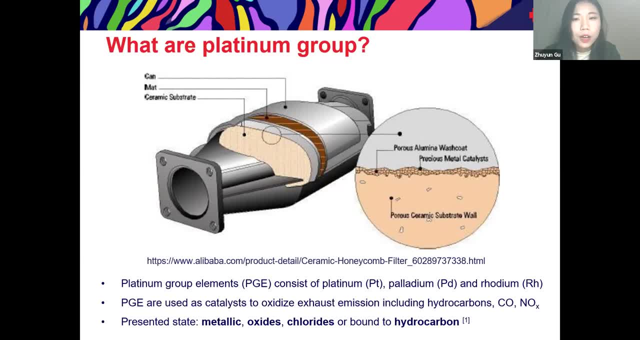 hydrocarbons and minoxides and during operations. due to surface separation, these metals are gradually emitted into the environment. So the platinum group is emitted at an estimated rate of 10 to 100 nanogram per kilometers. So the emitted platinum group are mostly presented at metallic states. 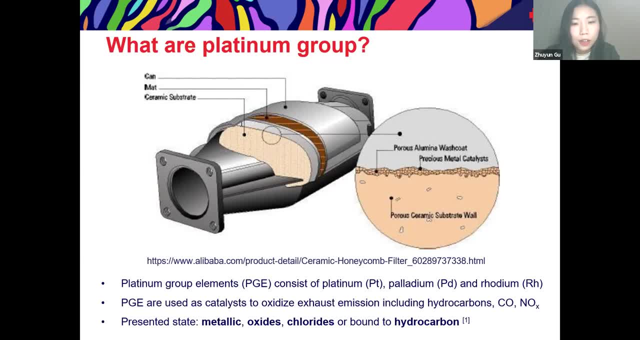 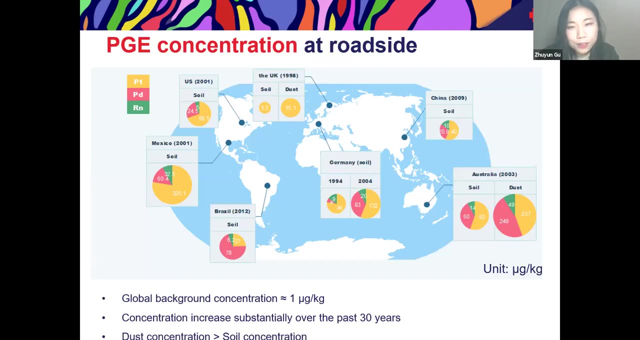 and some of them presented as oxides, chlorides, all bound to hydrocarbons. So now we know what platinum group are, but why do we investigate them? So, first of all, it's an anthropogenic source, so which means we need to assess its impact on the environment. 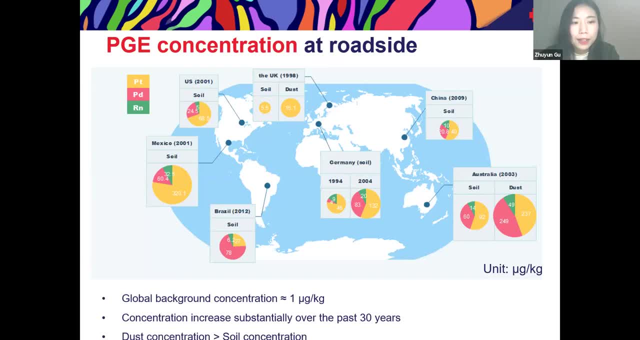 So here I summarize the platinum group concentration at road sites worldwide and plot this graph and and so the natural background. concentration of platinum group is around one microgram per kilogram and we can clearly see that um there's been substantial increase of platinum group concentrations worldwide and it's over. 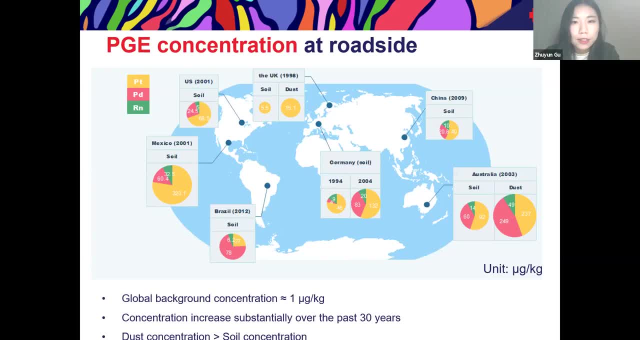 the past decades and according to the data from UK. so here's my UK and Australia. so we can see that the concentration in dust are higher than the concentration in soils, and this is because the emitted platinum group are actually first deposited as a dust and then gradually diluted in the soil. 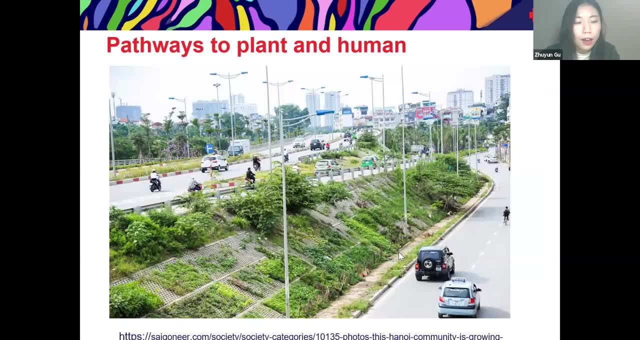 so, and another reason for is the potential linkage back to the plant and thereby entering the food chain. so, for example, in Australia we a lot of people have their back to back to food chain because of the concentration of platinum from their backyard and from your gardens. they are growing food in their 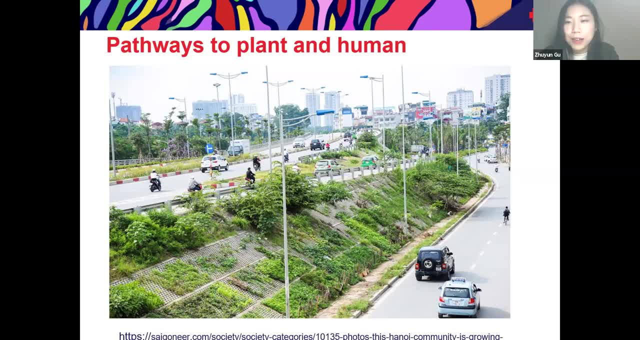 backyard garden, as Lizzie has already mentioned before, and also some agricultural lands that along the highways can also be affected, and recent year combining urban development with agriculture is also a hot spot and it discussed a lot, and all of them make us to think that we should have water and that would be the most beneficial and plentiful. 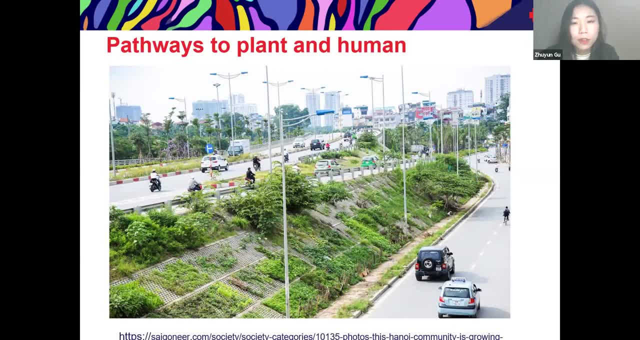 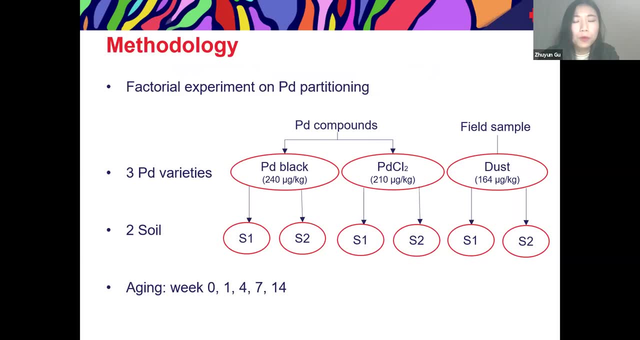 like how to assess the risk of platinum group in the soil. so in order to do that, we first know we. we first need to know what happened in the soil once it enters. so we developed a factorial experiment on platinum partitioning. so the partitioning is the distribution of metal among rice. soil component. 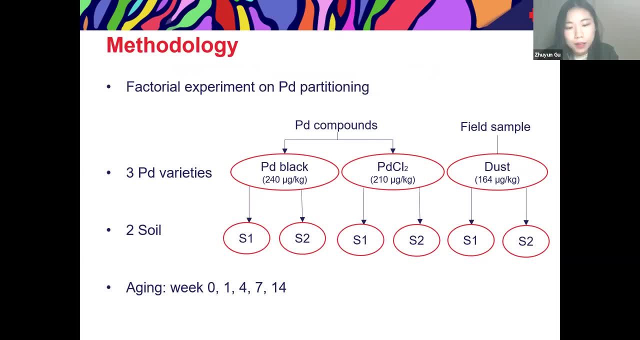 it can be either dissolved in water or be absorbed onto rice soil components, and we want to know whether the form of um palladium sources can affect its partitioning. so we choose on three form of palladium varieties. which is played in black, also known as metallic. 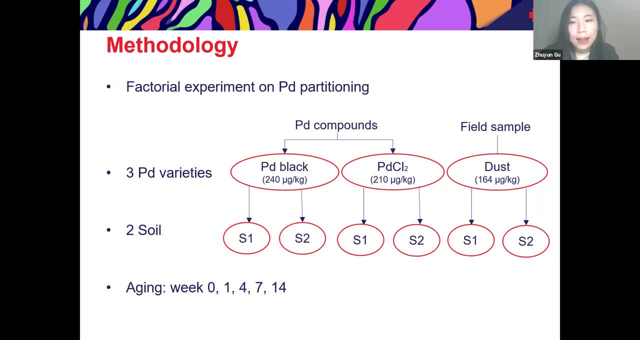 palladium and also played in chlorides and dust. so the um, as i mentioned before on metallic palladium and palladium chloride are the two main forms of emitted palladium and they can be regarded as the freshly emitted palladium and also rough side dust was collected as a few samples. 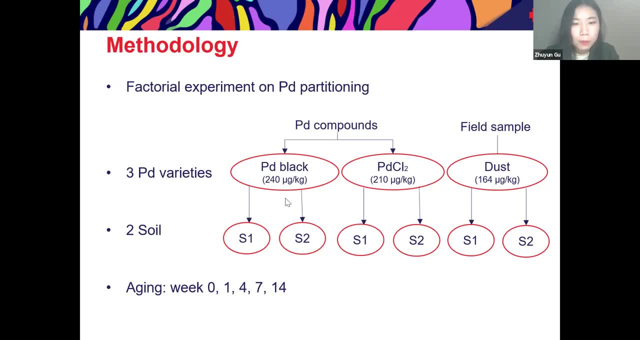 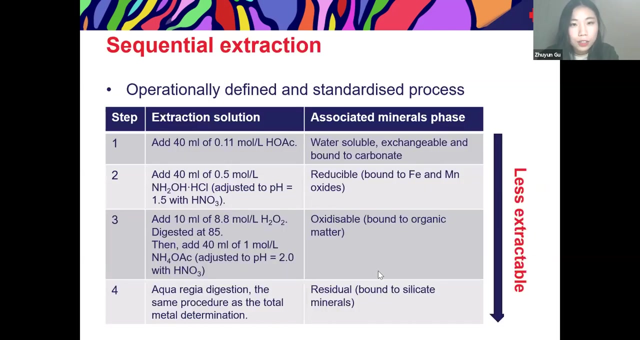 and we put the particle waterettener in that palladium and we got the sample that was collected. so i can just finish the right, so you can see the image here. so we use and i'm going to Harry say: um, we have four Adult machines on this Makai Lab. 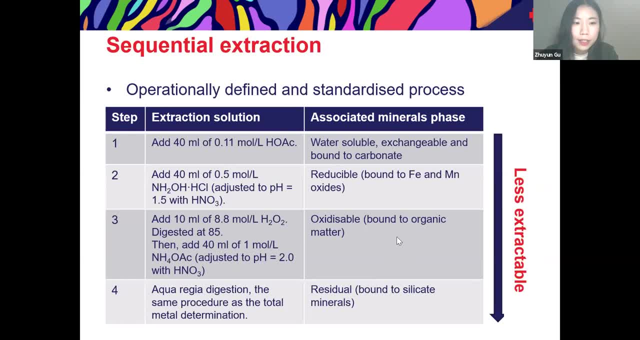 we use different chemical reagent to extract metals associated with a particular bonding sites in a defined order from easy to hard extracted And in the third column with associated mineral phase from top to bottom is getting actually harder to extract and which means the chemical bonds between metal. 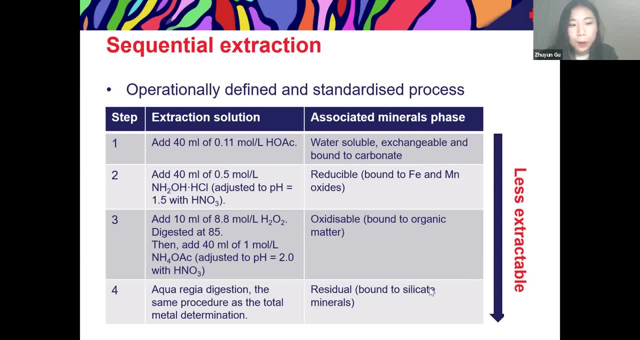 and soil components are getting stronger, And those which cannot be extracted, like the silicate minerals, we call residues. So what are these minerals means? So here is an illustration of a soil, and it consists of soil particles, which is the majority part. 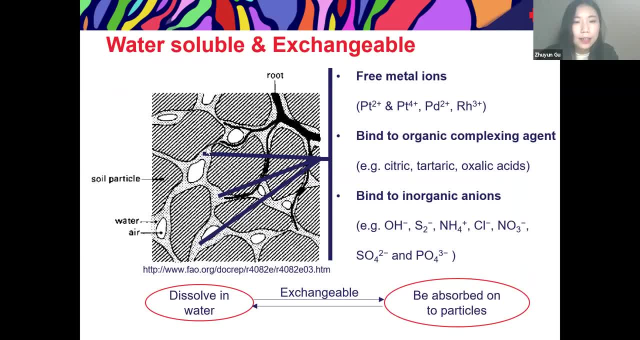 and then water, which is the main part, and then the soil Water and then sometimes air, And once platinum group enters the soil they may either dissolve in water or be absorbed onto various soil particles. So free metal ions binds to organic complexing agent. 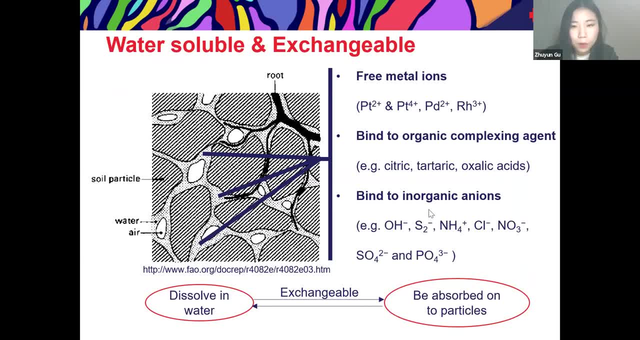 bind to organic ions. They are all dissolved in water, which comprise the first fraction And then exchangeable. Exchangeable is they can inter-exchange between the states in dissolving water and being absorbed onto particles when the soil environment change, for example pH. 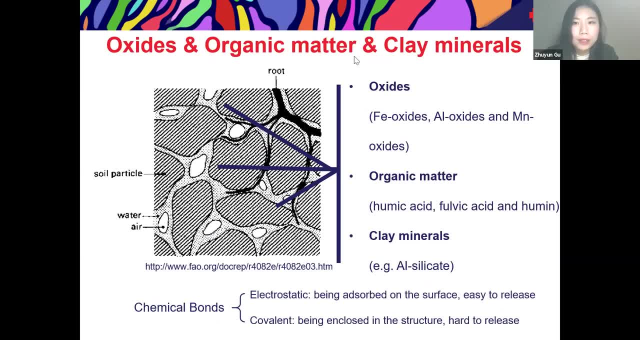 And, on the other hand, oxides, organic matter and clay, minerals are insoluble and they provide the majority of binding sites and they provide the majority of binding sites to soil to fix the metals And there are two kinds of chemical bindings. 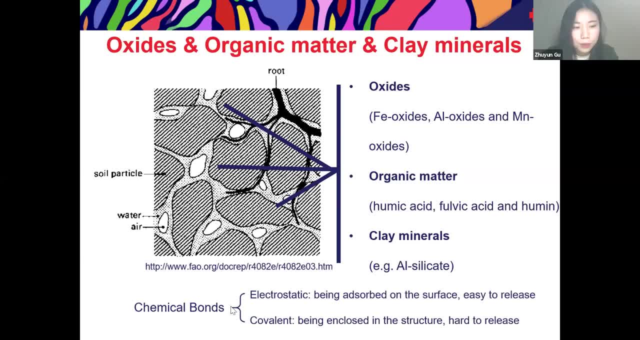 Electrostatic bind and which, being absorbed onto the surface and it's easy to release, it's a weak bind. The other is the covalent binding, which is being enclosed into the structure and which is a strong bind And, unlike covalent bind, 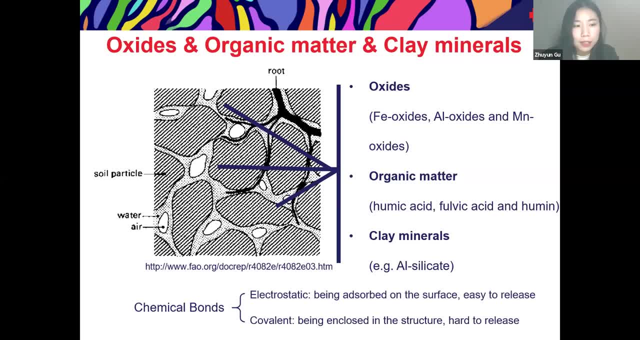 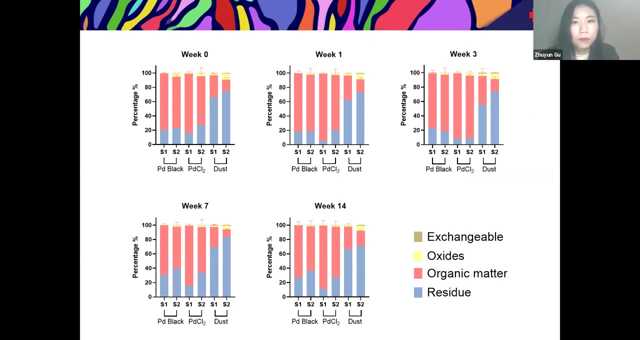 the electrostatic bind, the metal can be released back to the solution for plants to uptake and which becomes exchangeable. So some bindings, like clay minerals, are too strong to be extracted, so they're left in as a new residue. So here's what we we've got over the three months of 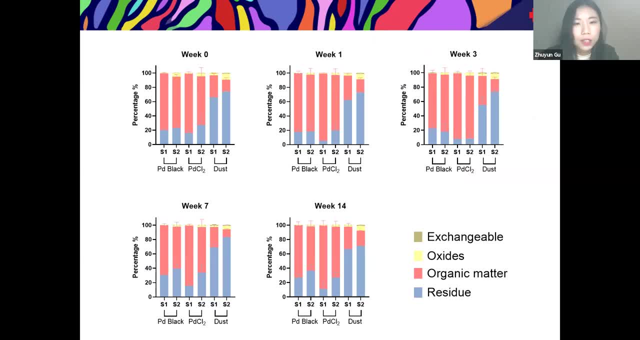 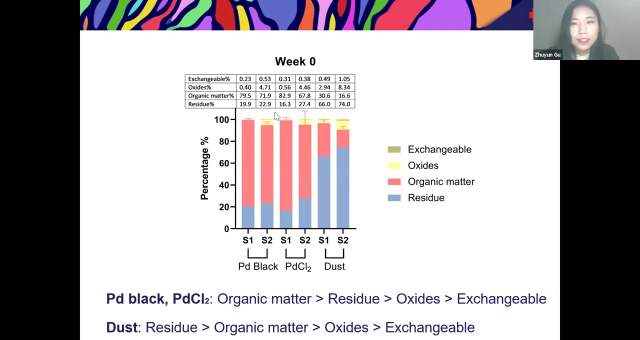 experience and we divided the concentration of each fraction by total concentration and get this percentage graph and we noticed that there's some general pattern in each graph. so I'll just take the first one, for example. So from the graph actually you can hardly see the first two fraction: exchangeable and oxides. 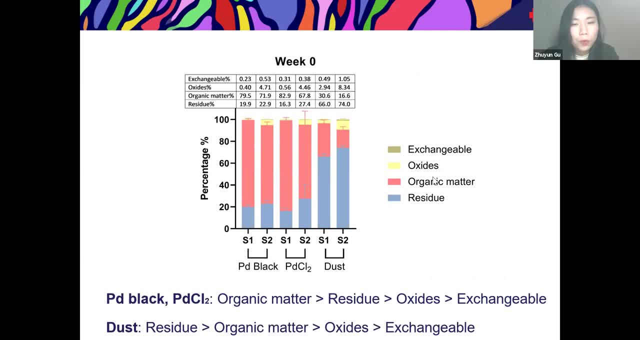 and indeed they comprise the concentration of the first two fractions. So what we found is that the first fraction is really low percentage, from 0 to 5 percent, while the largest component for platinum black and platinum chloride is organic matter, followed by residual oxides and exchangeable, and which suggests the majority of the 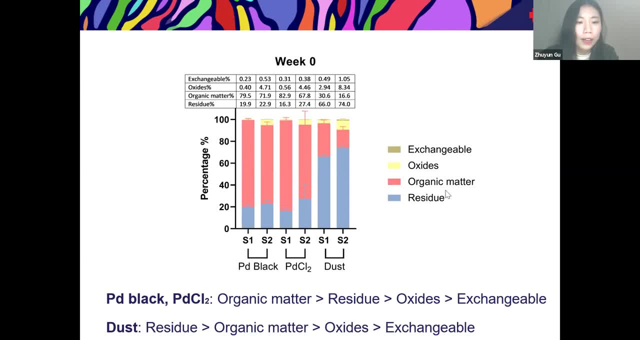 freshly emitted palladium can be potentially fixed by organic matter and dig around hand. the distribution of palladium in dust are quite differently. The residue takes up the largest part and followed by organic matter oxides and oxygen- sorry exchangeables. 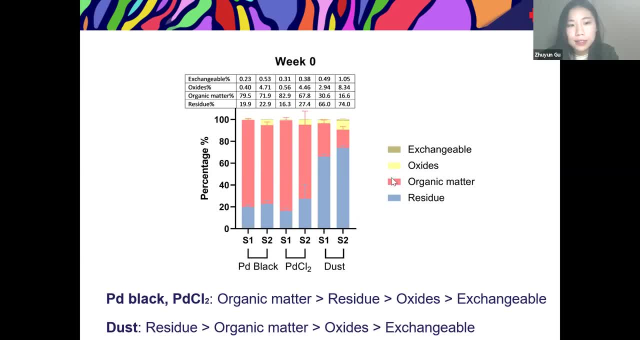 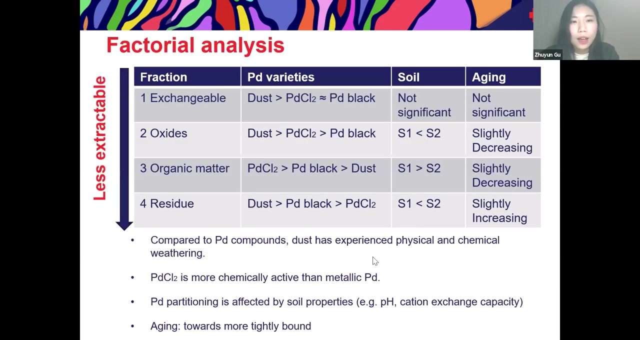 And that suggests the majority of the palladium in dust are quite tightly onto clay minerals. So the significant difference between palladium compounds and dust field samples also highlights the importance of including actual field samples in such experiments. We also analyze how each fraction responds to different factors that we tested. 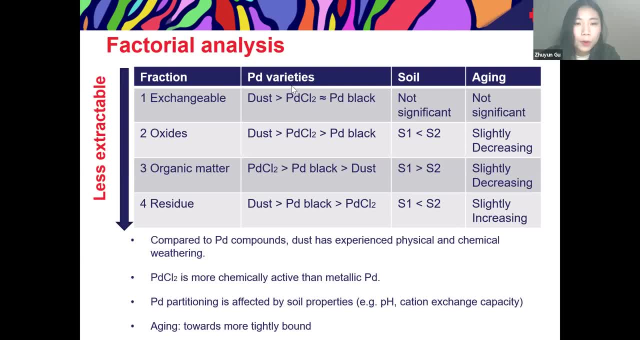 So in the palladium varieties column, if we regard palladium black and palladium chloride as a group, we can find that the dust got high- high in fraction in exchangeable oxides and residues. And this difference could be as a result of physical and chemical weathering in the environment. And if we compare palladium chloride, with palladium chloride we can find a large amount of mechanical action. This also makes to fooled us a little bit, for example, that there are applicable factors in the fraunchy dust category. know this kind of addition of calcgrunting oxide, vin 3000,있anolre denial and. diethylamine lockout住室. shape of this process: The common alpha and fat is about 1200% of in one second of no casual ajudaous stage inもう. for the other, please note, is that in prevarications. 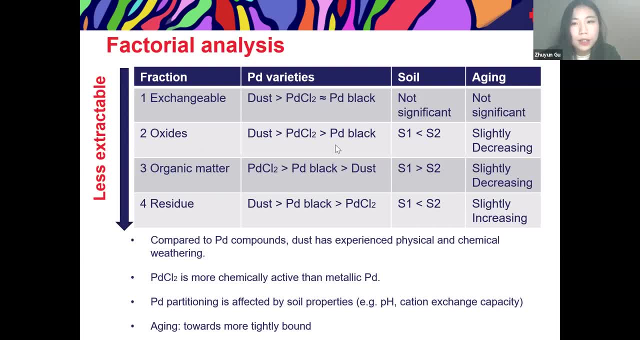 and also in travel 3024, Microsoft Alice Doc said before that heavy Excほi with palladium black. we could see that they got equivalent or higher figures in the first three rows And this is in line with the chemistry behavior. 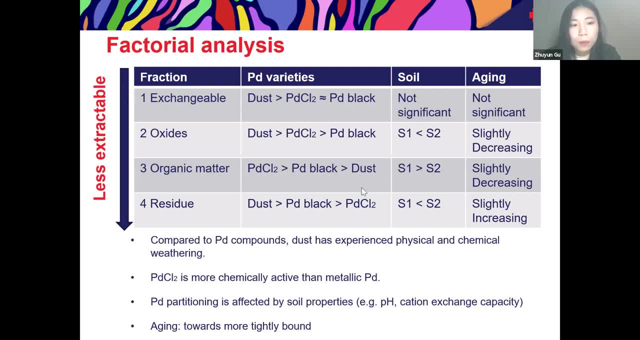 which palladium chloride is relatively active than metallic palladiums, And the only exception is the residues, And it is instead of suggesting that the palladium black is more active than chloride and bonds to more clay minerals, it is more likely that it is too inert to be dissolved. 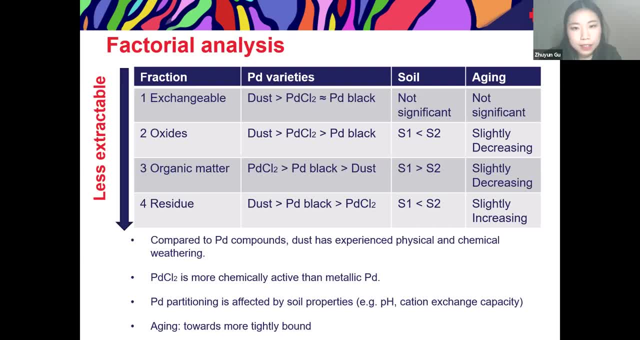 by the extraction solutions and thereby left inert And the residues And for soil- except for the first row, where the data of exchange flow is too low to be significant different, and the rest of them all shows different preference to soils. 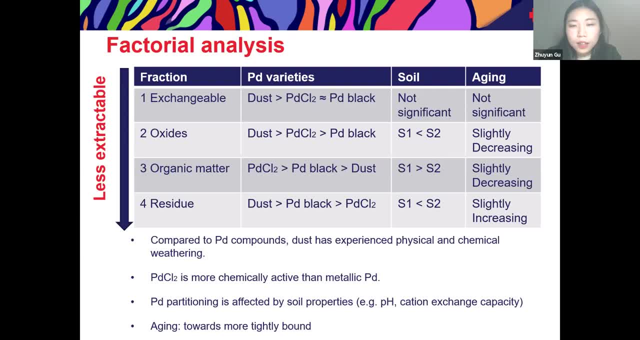 And this suggests that the partitioning of palladium are affected by the soil properties Such as pH or cation exchange capacities For agents. similarly, we couldn't see a significant difference for the exchangeful fractions, But we can see that for the oxides and organic matter. 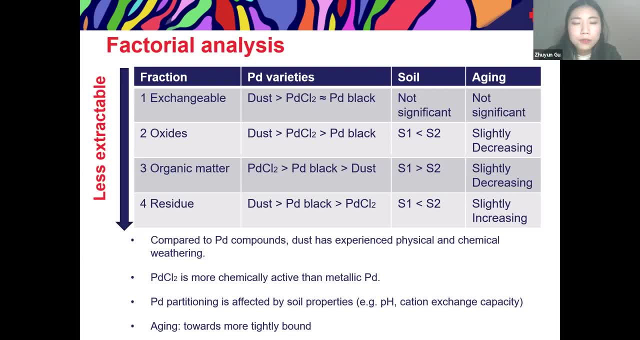 they are slightly decreasing, while the residue is slightly increasing, So it's suggesting that it's getting more and more towards tightly bound. And for the first row, as you can see, these were not the same And they were not the same. 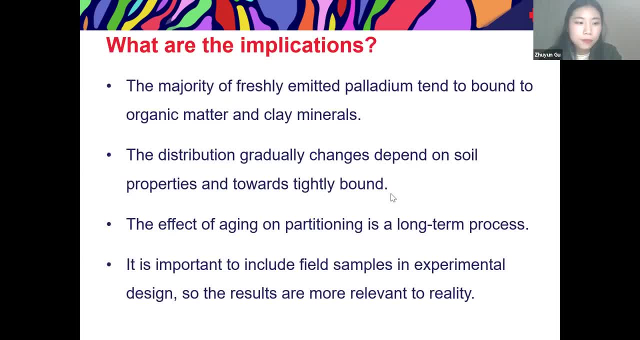 So it's very different. um, so what are the implications? first of all, we could establish a storyline of what happened. what happened to palladium? once they enters the soil, and the majority of them tend to bound to organic matter and clay minerals. as the and as the time goes, with constant physical and chemical 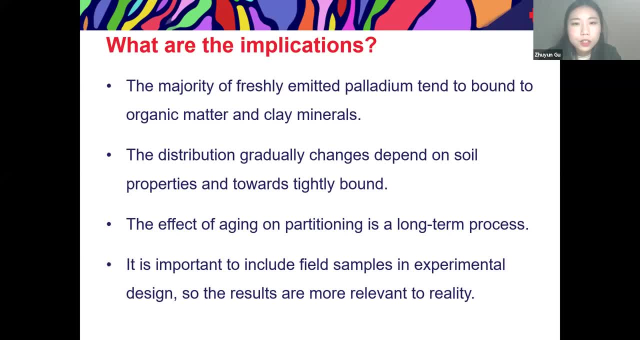 weathering, the distribution are gradually changed, depend on different soil properties and, in general, going towards more tightly bound. however, this time period could be much longer than our experiment period, because in the duration of three months we could only see the slight change of each fraction, and we also kept one batch and left it for a year. 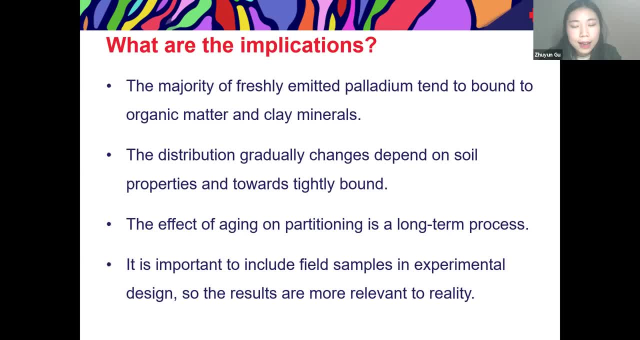 and it would be interesting to see what's the results and whether it can provide us any new thoughts, also the significant difference between palladium compounds and field samples, suggesting that in the face of experiment design, it's important to include field samples where possible so the results are more relevant to reality. and here's the reference. thank you for. 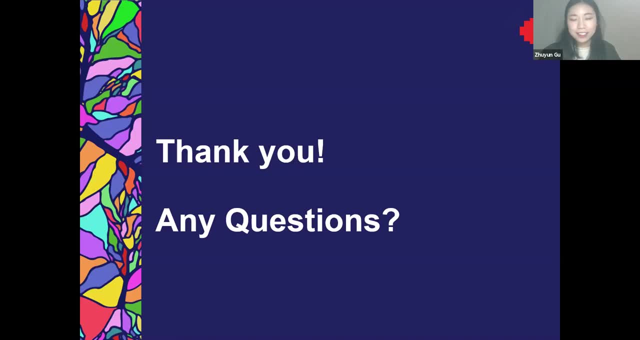 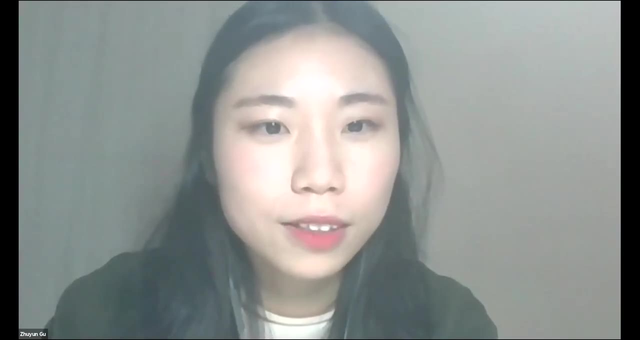 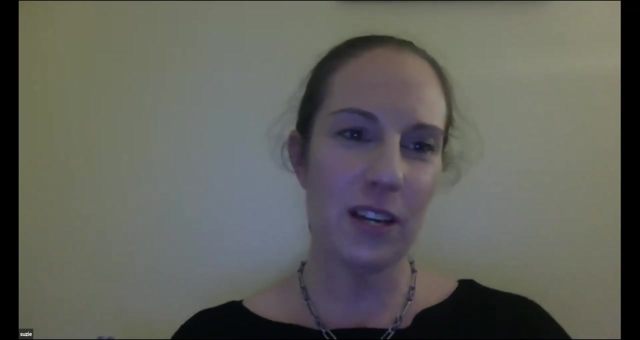 this meeting, my presentation, um, so i will just hand over to stop sharing, okay. okay, thanks, juan. um, so now we're gonna have justin uh coming up and talking about part of his phd research, so just um chat while justin's sharing his screen. 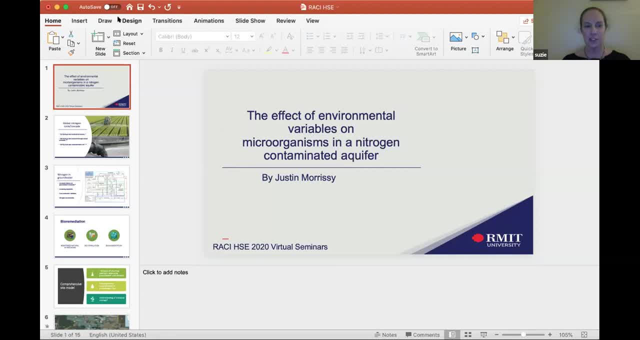 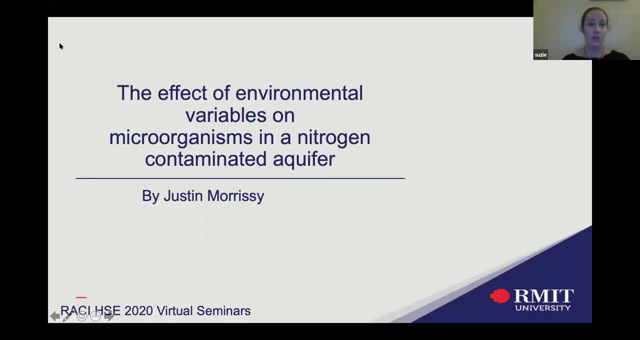 um. so justin's research is a little bit different to a lot of the research that we have in our group. he's been looking at groundwater and um nitrogen contamination coming from um sewage treatment plants and trying to bioremediate that uh, the nitrogen i mean he's not typically talking about. 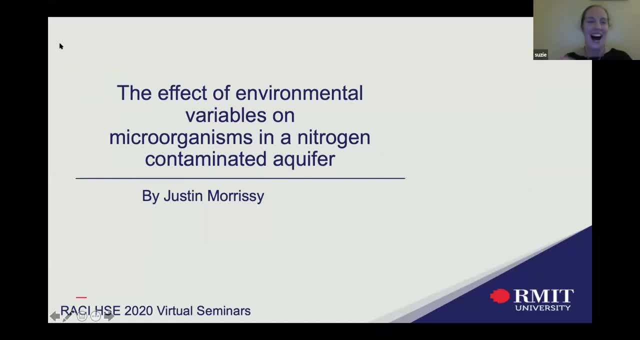 the buyer, you're trying not always easy um and he's not going to be talking about the bioremediation part of it tonight. he's going to be talking about understanding the natural um organisms that are in that um nitrogen contaminated aquifer, because the idea with um the 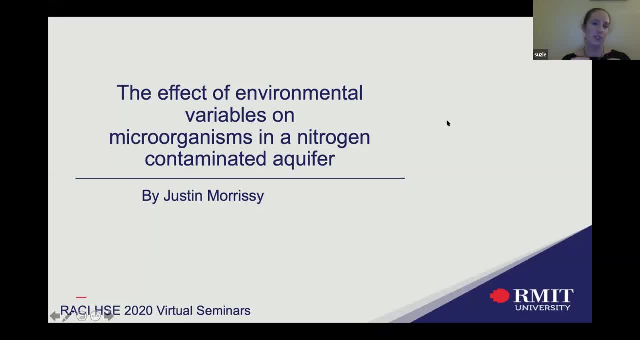 by remediation. that he wants to do is to use those indigenous um bacteria and encourage them. that's, you know, the first, much easier, much more environmentally sustainable way to do it: to encourage those bacteria, um and overcome any limitations that they have. and so he's just. 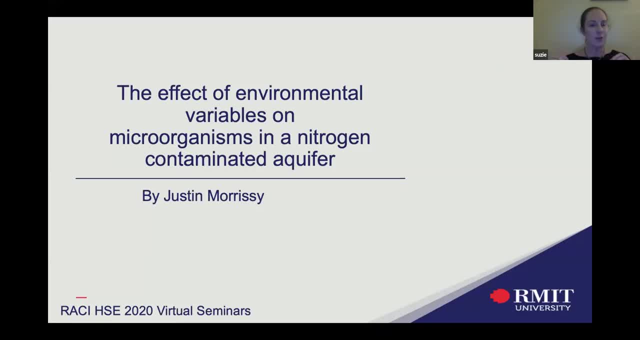 going to talk about the environmental variables in the bioremediation part of his talk. so justí, environmental variables in that aquifer and how they relate to the different micro-organisms, and trying to get an idea on what are the factors that affect those micro-organisms. 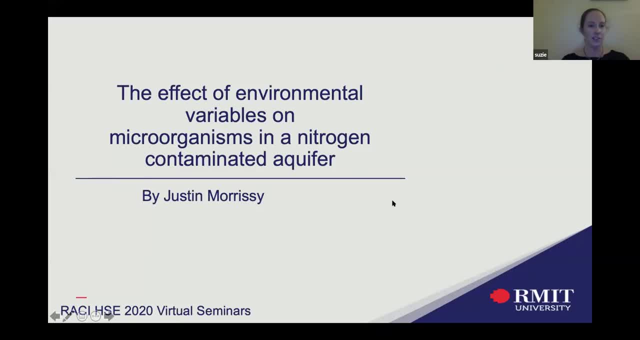 being successful And I'll hand it over to you now, Jason. ah, Justin, sorry, Everyone can see my screen, Yes, Cool. So yeah, this is my talk. the effect of environmental variables on micro-organisms in a nitrogen. 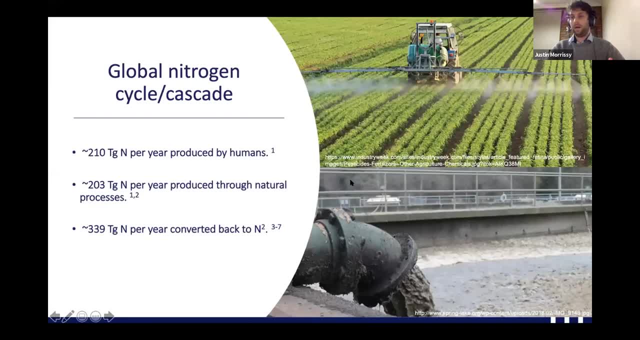 contaminated aquifer. So we know that globally, approximately 210 teragrams of nitrogen is annually by humans and an estimated 203 teragrams is produced through natural processes. And we also know well- we estimate- that approximately 339 teragrams is being converted back into. 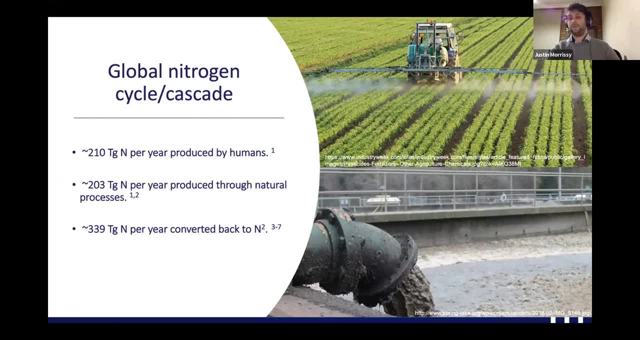 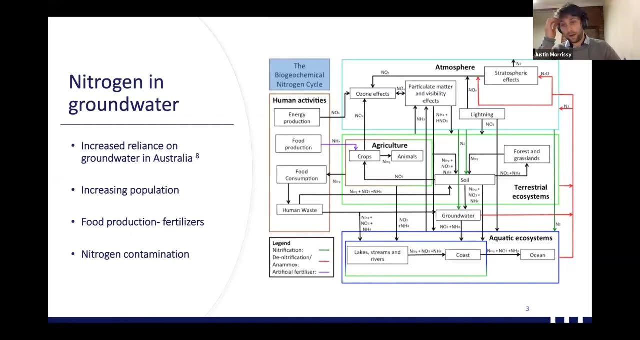 nitrogen gas annually. This leaves about 75% of the world's nitrogen-contaminated aquifer. So we know that about 74 teragrams or 74 billion kilograms of nitrogen accumulating in our environment annually, According to the CSIRO as of 2004 and 5, approximately 25% of Australia's groundwater. 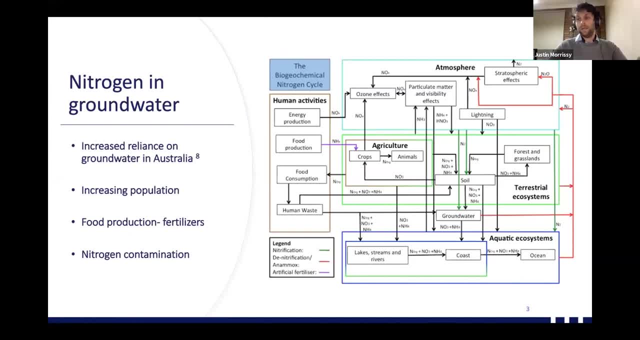 use comes from ah. water use comes from groundwater, And as the severity and length of droughts in Australia increase and surface water reserves deplete, this number is steadily increasing. In addition to that, we also know that the amount of carbon dioxide that is produced 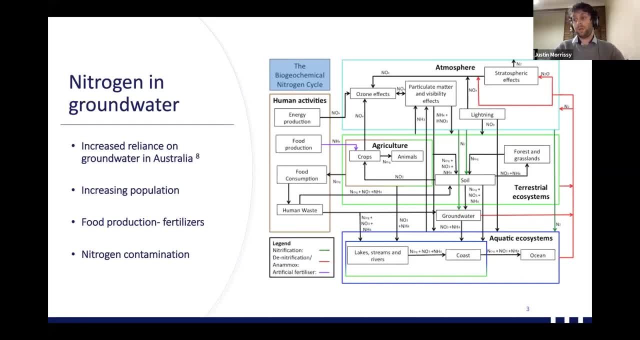 in the environment is increasing. In addition to this, increasing population is putting strain on wastewater treatment plants, and increasing food production is causing more fertilizer use, both of which can lead to nitrogen contamination. When these factors are combined, we begin to get a picture of increasing reliance on. 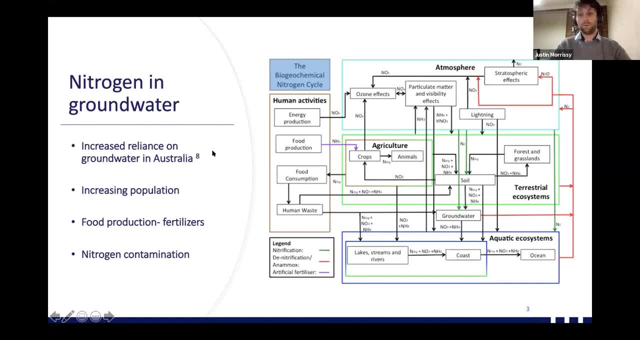 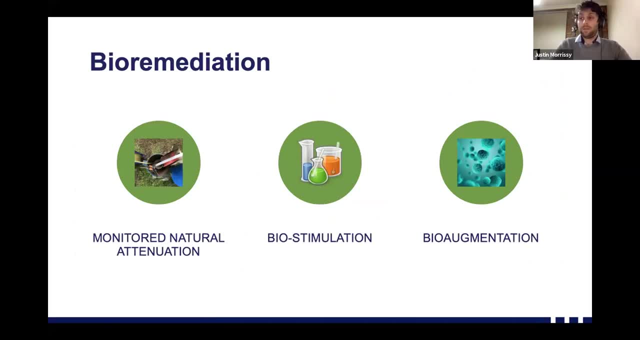 increasingly nitrogen-contaminated groundwater reserves. To combat the increasing incidence of nitrogen contamination, in many instances some form of remediation is necessary By understanding and working with the environment. bioremediation techniques aim to decrease the time and cost typically associated with a lot of remediation techniques. 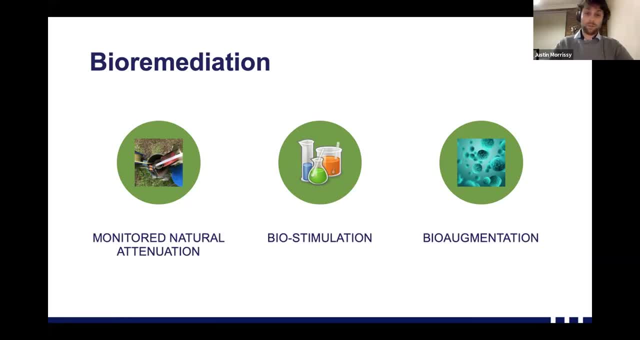 There are three primary bioremediation techniques: monitored natural attenuation, biostimulation and bioaugmentation. Monitored natural attenuation involves observing the groundwater to determine whether or not it's remediating on its own. Biostimulation, as Susie mentioned before, involves adding limiting nutrients to the 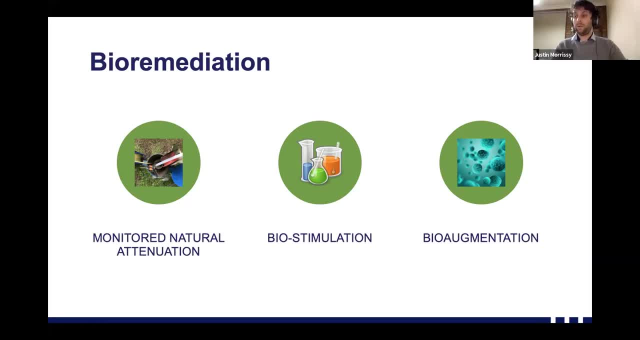 environment. And bioremediation involves adding more nitrogen to the environment. The bioremediation techniques: use bioremediation techniques to simulate the groundwater ecosystems and speed up the natural attenuation. And bioaugmentation involves adding an organism to the groundwater. 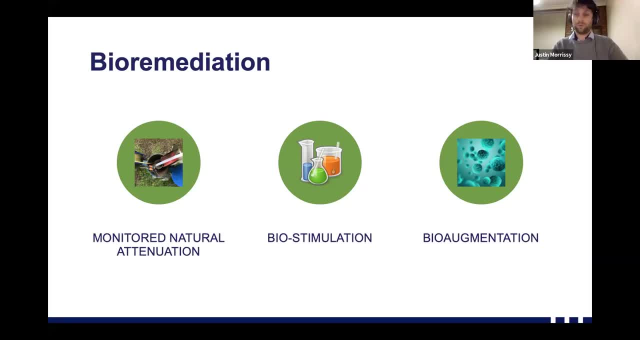 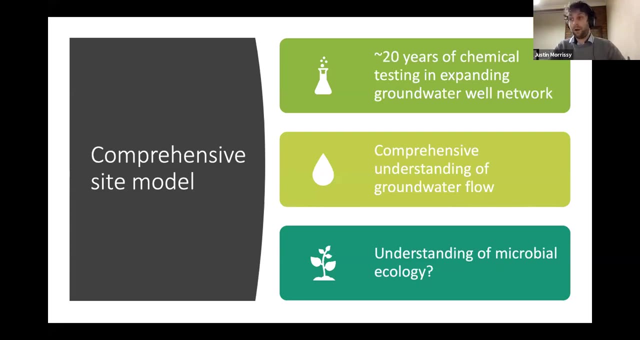 This is typically only done in remediation, if it's not possible to remediate the area due to some sort of missing biological process or if monitored natural attenuation and biostimulation didn't work. The first and most important step to effective bioremediation is a comprehensive site model. 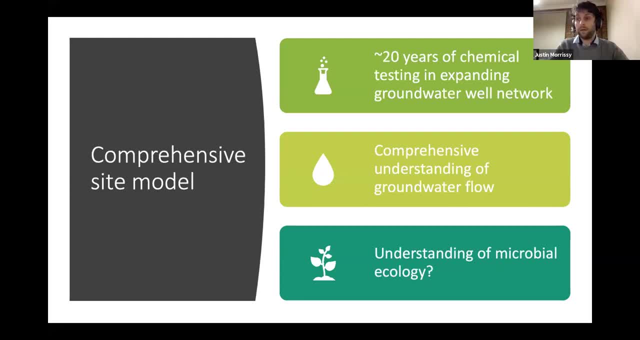 model. At the site I mainly work at, we have approximately 20 years of groundwater data and we have a pretty comprehensive understanding of the groundwater flow. However, like most sites, especially in Australia, we have little to no understanding of the groundwater microbial. 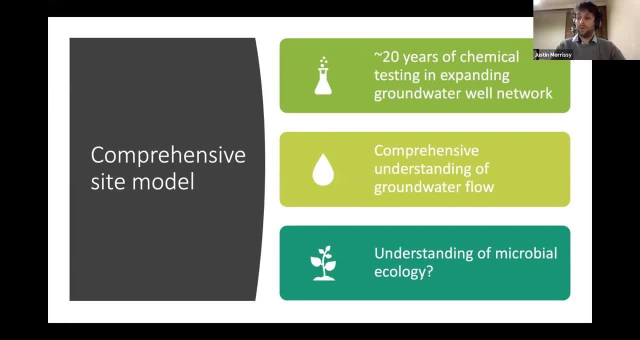 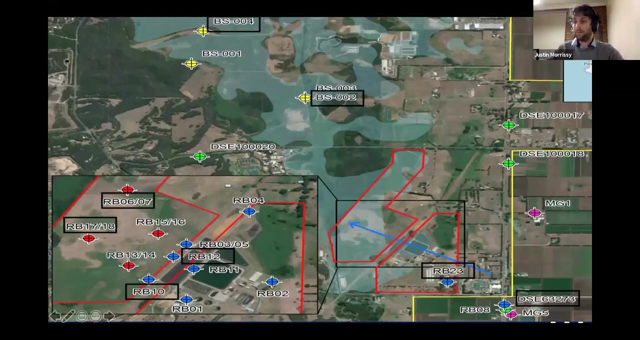 ecology and its interactions with environmental variables. To better understand this, I've combined chemical testing with 16S RNA next-gen sequencing data that's been sorted into relevant functional groups. This will hopefully enable me to look at how chemicals affect their relevant functional groups in the environment. So this is a site map for my main site: The locations. 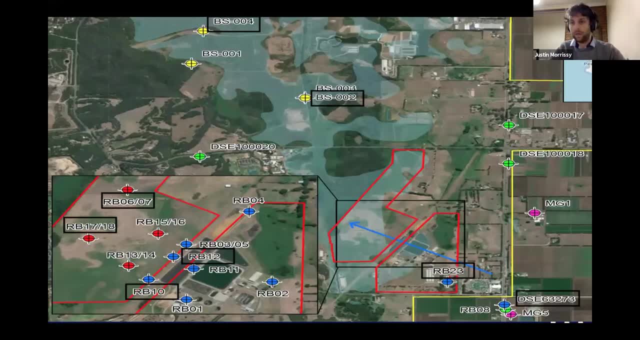 that I sample from are in the little black squares And the groundwater flow direction is indicated by the blue arrow. This is the approximate contaminant plume. This is the site model, which there is one out there, but I don't have access to it. But this is. 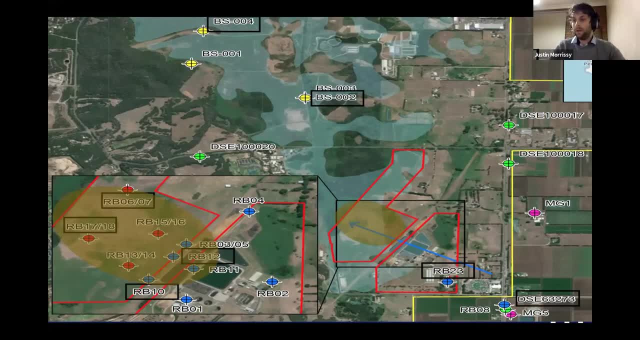 the approximate area that the plume covers, And there are several groupings on the site map. We have RB23 and DSE down in the corner. Those are upstream from our main site And they're not affected by the main contaminant plume. However, there is also agricultural. 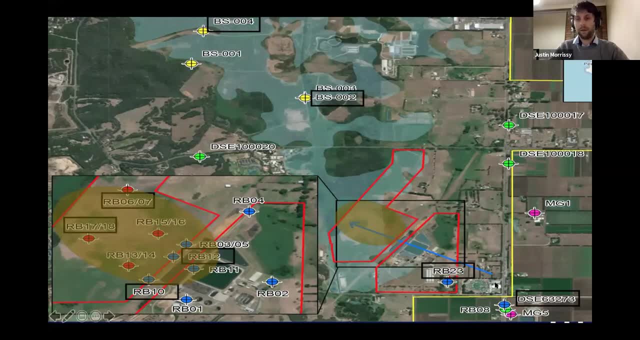 regions upstream, So those sites are affected by the agricultural regions. So I'm going to go ahead and show you some of the sites that I sample from. I'm going to go ahead and show you some of the sites that I sample from. We have RB10 and 12, which 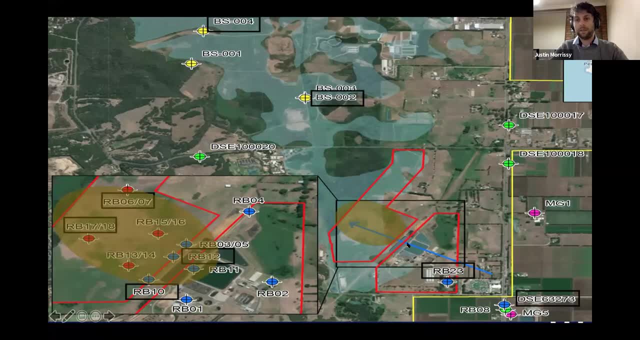 is down here. This is just a zoomed-in version of the main site. We have RB10 and 12, which are kind of right at the forefront of the contaminant plume, right where all of the point source contamination is coming from, which is the wastewater treatment plant itself. 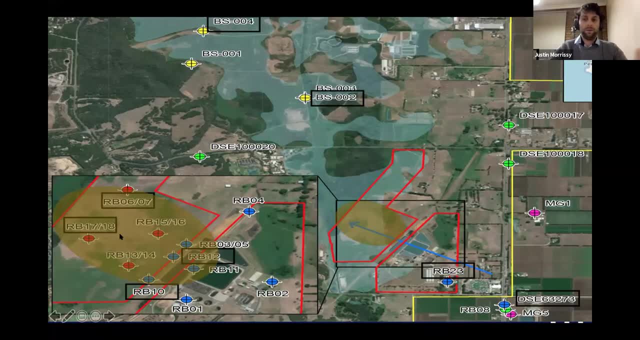 We have RB17 and 18,, which is kind of right in the middle of the plume, And RB6 and 7,, which are on the upper edge of the plume, And then we have all the way up. here we have 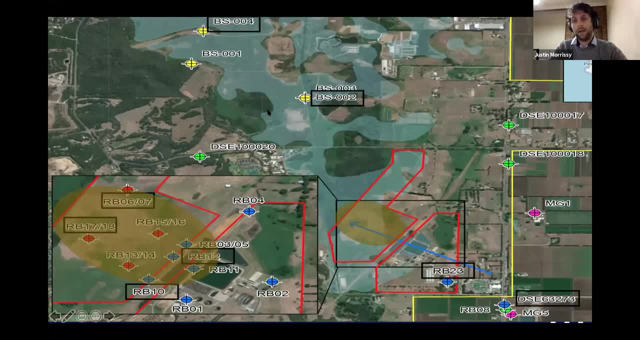 BSO2 and BSO4, which are our downstream kind of control bores. They're well and truly outside of the effect area of the plume and downstream Because unfortunately we can't use upstream bores because they're all contaminated by the agricultural region. So here we have. 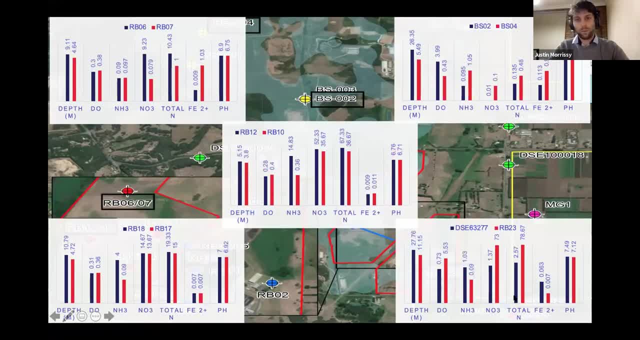 some of the chemical data. I've grouped it based upon those groupings that I just mentioned: the upstream bores, RB10 and 12,, RB17 and 18,, 6 and 7, and BSO2 and BSO4.. 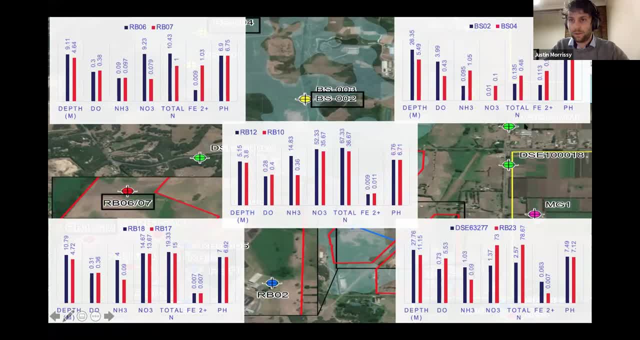 If I can move this, I can actually see There we go. So there's seven environmental variables that we're looking at. We've got depth dissolved oxygen, ammonia nitrate, total nitrogen, ferrous iron and pH, And I've showed just. 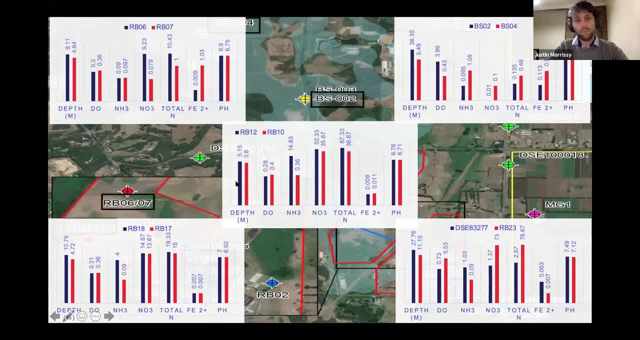 a little bit of the data on the left. And then we have the next-gen sequencing data, And this is just for convenience of analysis of this. all of the deeper wells in these pairs are in blue and all of the shallow wells are in red. 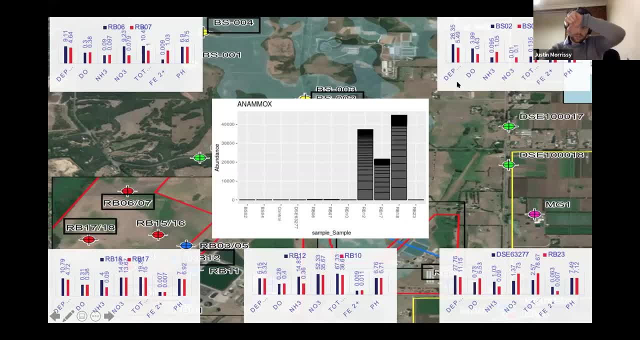 So the first step: we've got Anammox, So to preface all of this next-gen sequencing data is preliminary data, So we haven't done any statistical analysis on it, So we're mostly looking at just surface interactions for all of this. But this it does, that we do glean. 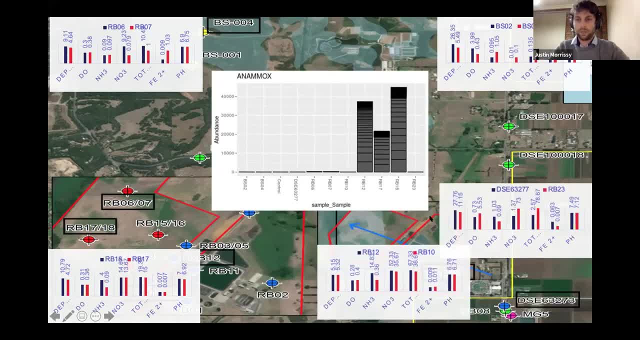 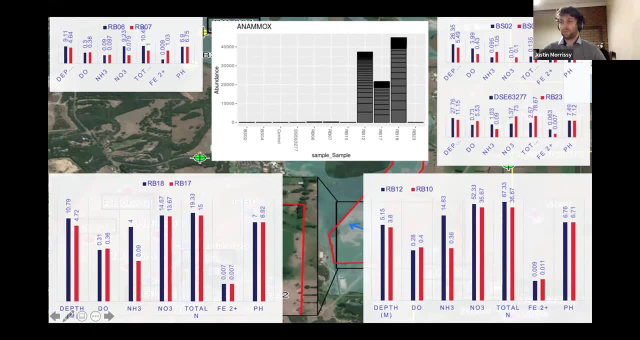 quite a bit from just looking at these kind of surface interactions. So we've got our Anammox here And we can see that the Anammox bacteria are most highly represented in RB12 and RB12,, 17, and 18.. And within those, 12 and 18 are the most highly. 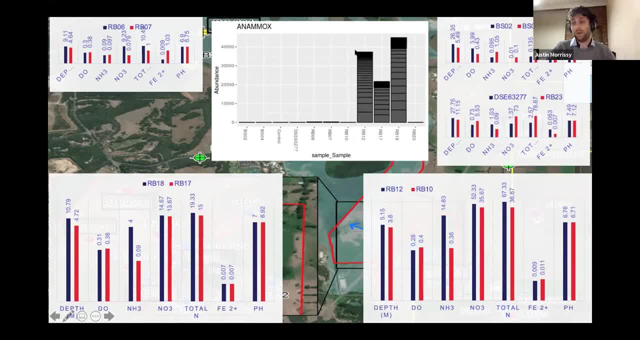 represented. 12 and 18 also have the highest concentrations of ammonia If we look at the at these guys here, And they also have quite high concentrations of nitrate. Both of these are required for the Anammox reaction. RB17 has a lower concentration of NH3, but still. 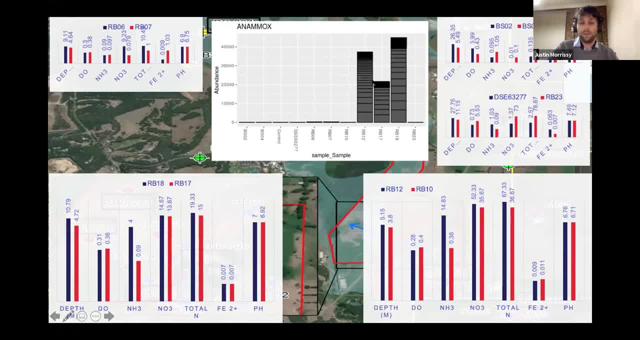 an elevated abundance of Anammox. This is most likely due to the high abundance that we see in RB18.. RB18 and RB17 are paired wells so they're right beside each other, So they're not necessarily the most highly represented, So we can see that there's a strong likelihood. 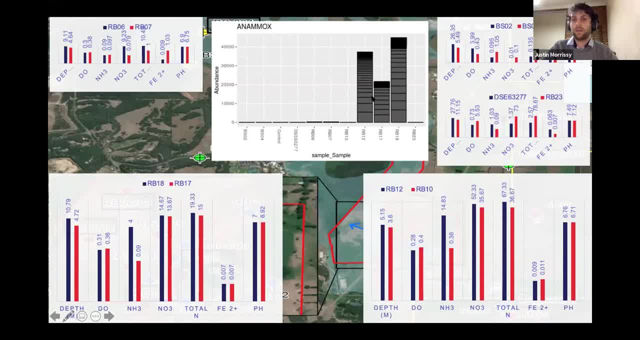 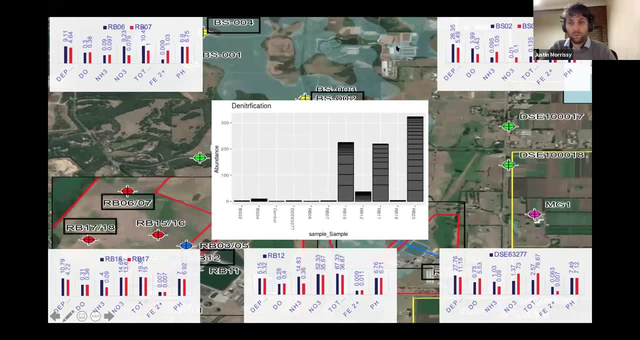 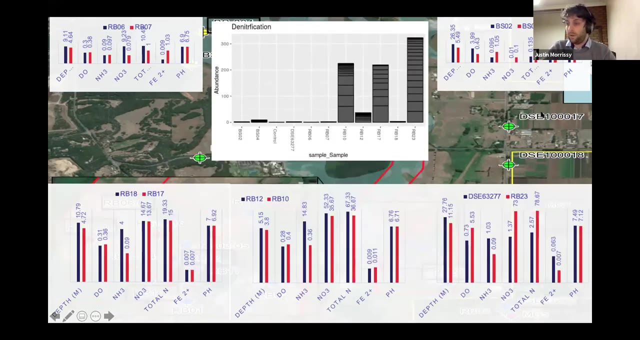 that anything that's in RB18 will also have some effect on RB17 as well, So we'll probably see that again. So move on to denitrification. For the denitrification bacteria, we can see that RB10,, 17, and 23 are all the most highly affected wells. Interestingly, these three. 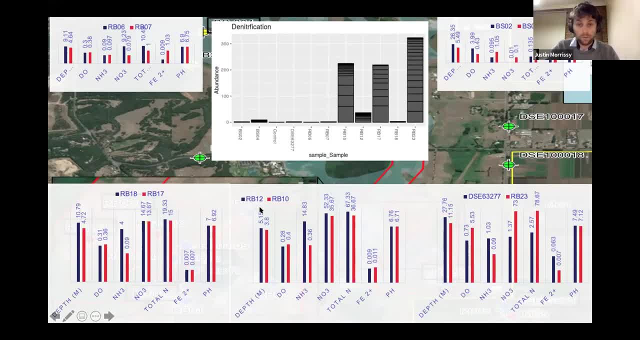 wells are all the shallower of the grouped wells, which is actually a little bit contrary to what we would expect from denitrification. Typically, denitrification likes a deeper well Because of the lower dissolved oxygen levels, although all of these have quite low dissolved 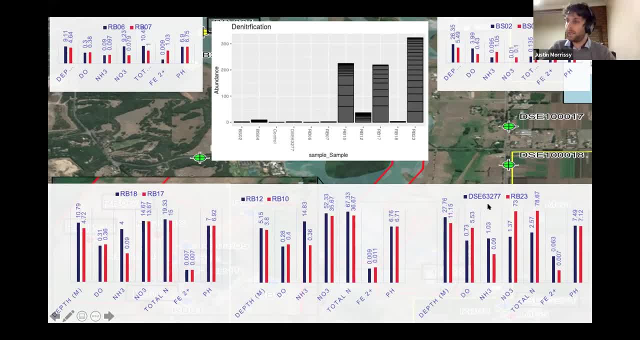 oxygen levels in the first place. So that doesn't seem to come in play here. RB12 also has a blip on the radar, but there's actually not much difference in depth between RB10 and 12. So there's not a huge amount of surprise there either. And then we've got iron rest. 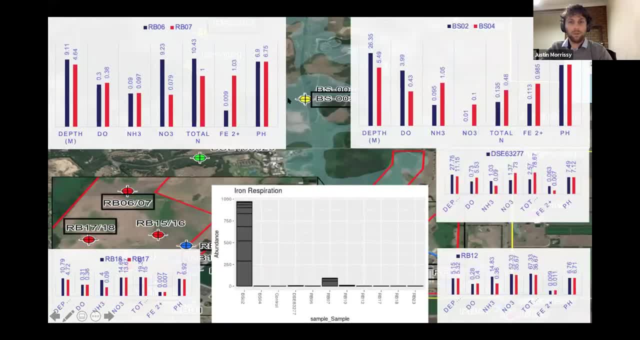 respiration. Iron respiration is one of the more fascinating ones, in my opinion anyway, Because we can see that it's affecting BSO2 and RBO7.. BSO2 has not got all that much iron in it, but RBO7 has the highest levels of iron that we see in the sites that we're talking. 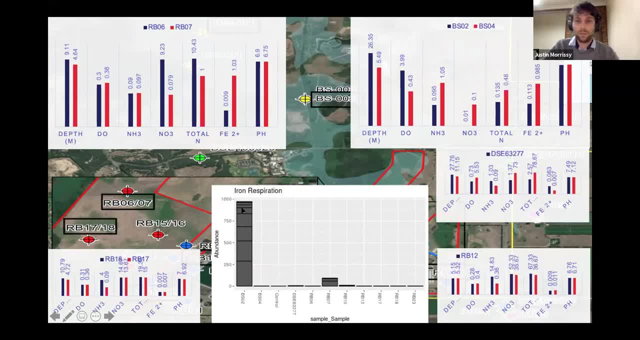 about here. Okay, So BSO2, although it doesn't have- oh, RBO7 is over here- BSO2,. although it doesn't have particularly high iron levels, it does have pretty much zero nitrate, And I don't have 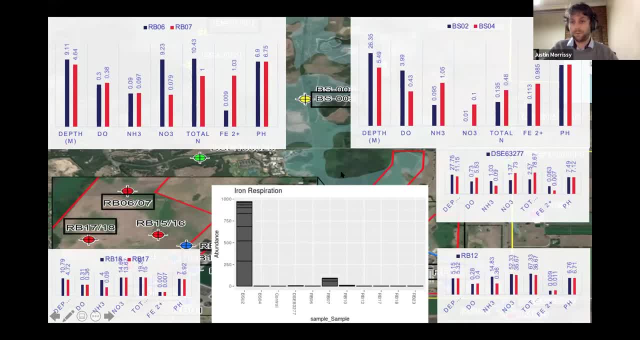 the chemical formula up here. but the chemical formula for iron respiration actually directly involves, obviously, iron and nitrate. So the fact that we are missing nitrate and we don't have that high iron levels may have in my theory, is that it has something to do with. 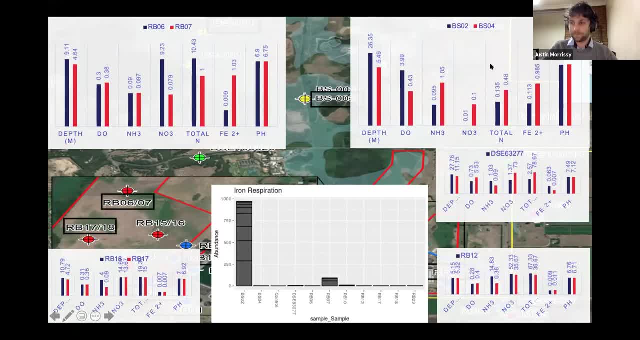 those two factors interacting with each other. So obviously we haven't done any statistical analysis on any of this stuff, so I can't go into how statistically significant all of this, all of these things, are. but I think there's some really interesting relationships going on between all of our different and 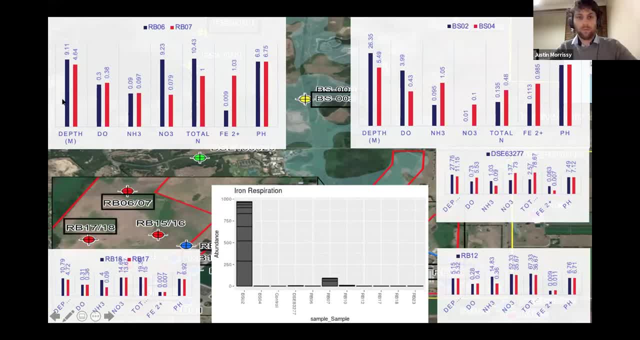 I'm sure there's more that we could look into with pH and dissolved oxygen and stuff like that, but I won't go into it with too much detail here. Okay, But for further analysis, we have a bunch of experiments planned, some of which. 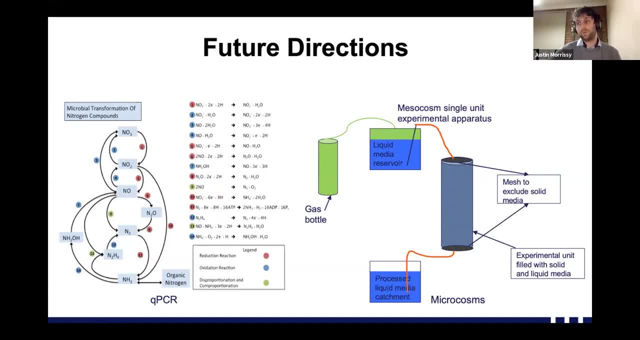 have been somewhat interrupted by the current situation. So we're planning on doing qPCR, which will essentially will be tacked onto our next-gen sequencing and give us some more quantitative analysis of the genes that are functioning in the groundwater, And then we'll 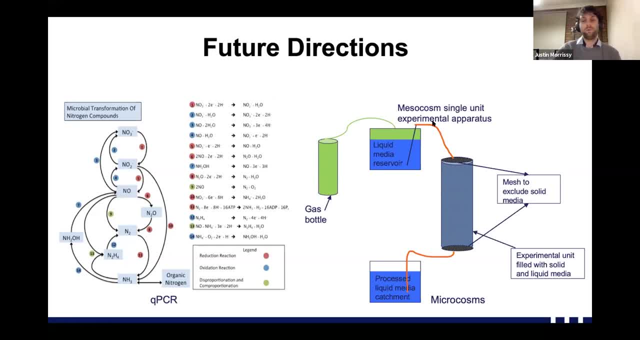 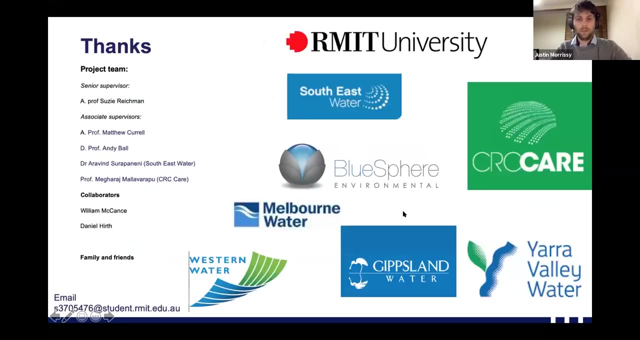 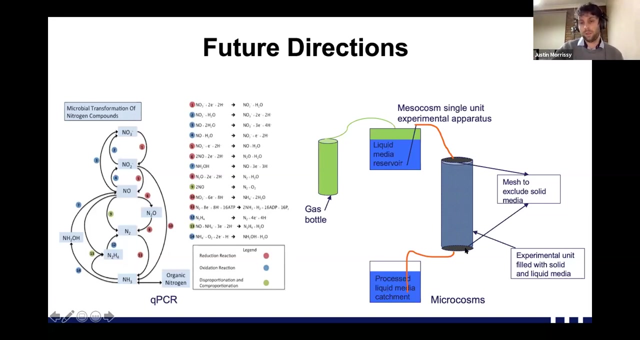 be moving on to microcosm experiments. So we'll be attempting to replicate the groundwater environment in the lab and we'll be isolating variables that we particularly want to look at and looking at those in these projected environments. This has undergone several iterations and we're hoping that we can accurately represent what the groundwater 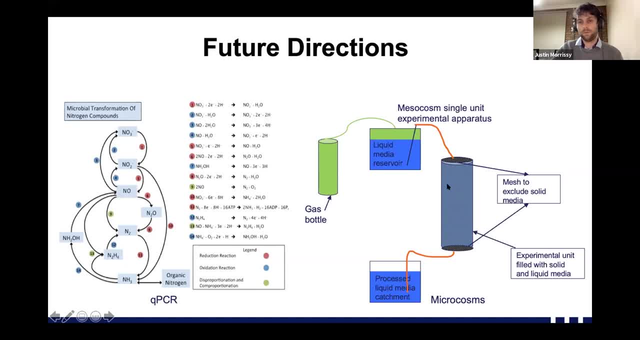 is doing in the lab Using. this is actually one of the one of, I think, three, three apparatuses that I know of in the world that is attempting to do something like this. So it's it's got a few kinks that we need to still work out. 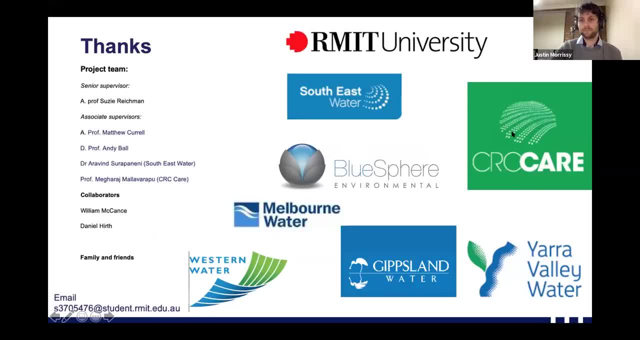 These are our many, many collaborators. CRC-CARE is our biggest collaborator. is is our as our funding body. And then we are collaborating with pretty much all of the all the water groups in the Melbourne area and a couple of Blue Sphere Environmental Loop Blue Sphere. 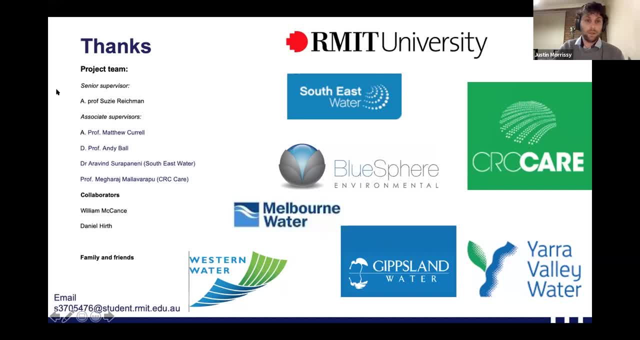 Environmental Loop, who is is also helping out, My huge project team over here, who are very helpful, And William McCance and Daniel Hurth, who are doing a paired project with mine that looks at the movement of these contaminants throughout the groundwater. My email, which 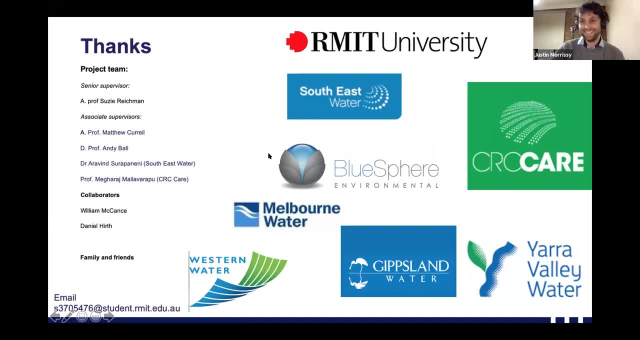 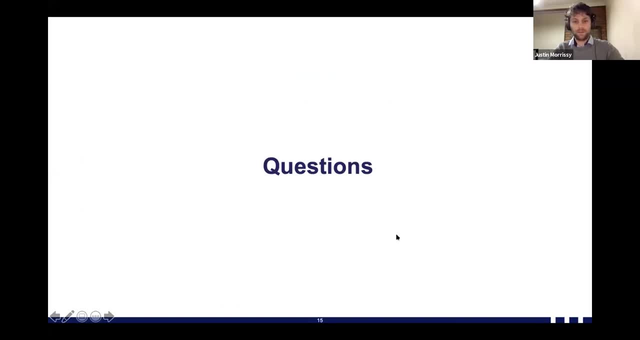 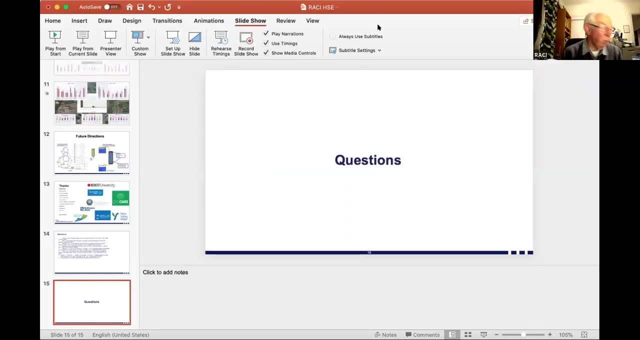 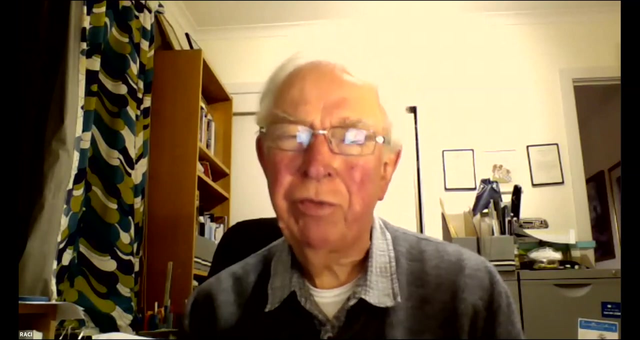 I added just before when Susie added hers, because I thought it would be look good And references Well. thank you very much, Justin, and Susie and Joanne. I think we've all been treated to a really fantastic overview of the work, the research that you're doing at RMIT Now. 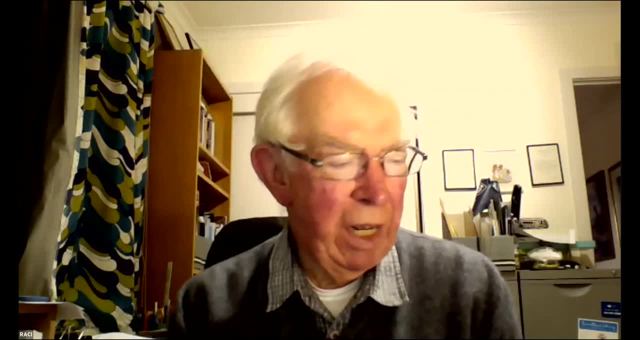 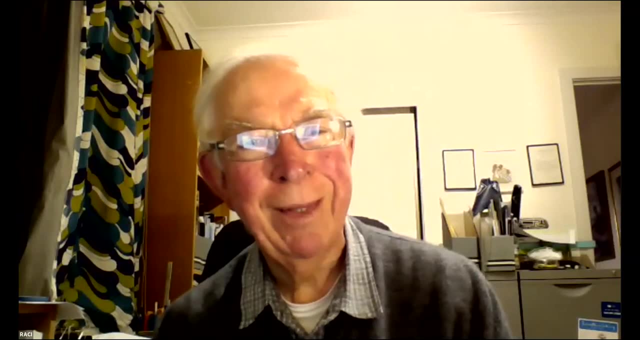 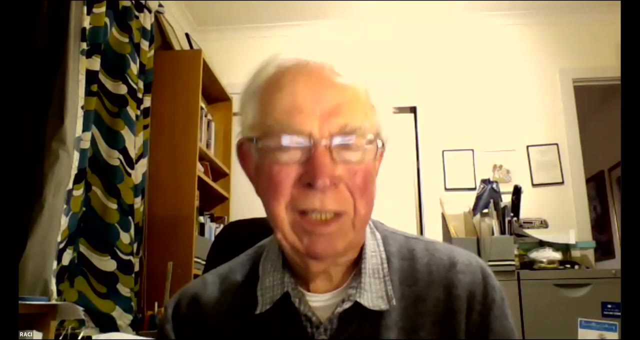 Ian Thomas, at this stage, was going to chair the answer session. Yes, he is. Are you in a position to do that, Ian? Absolutely, Yeah, Well, thank you. I know that there have been a lot of questions and answers during the chat, during the presentation. 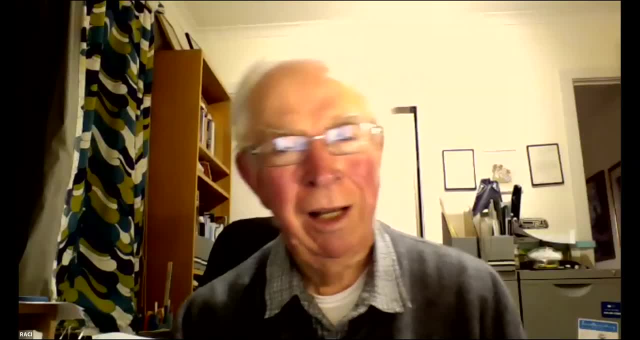 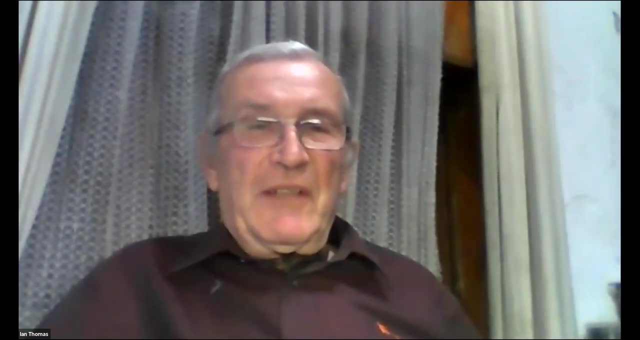 Indeed, If you'd like to facilitate a few more questions for the next five minutes or so, that would be great. Thank you, Richard, And thank you everybody- This is terrific- And all three of you for your presentations. It is delightful for our group to go and have a chat with you. I hope. 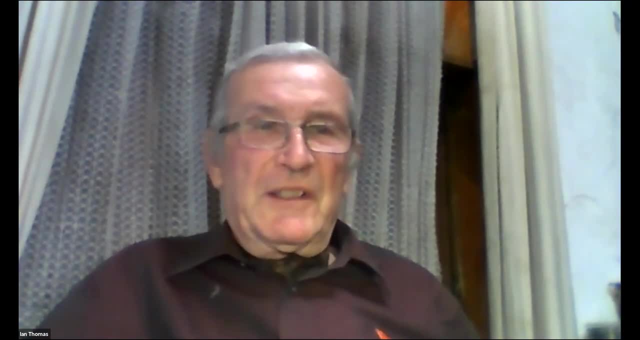 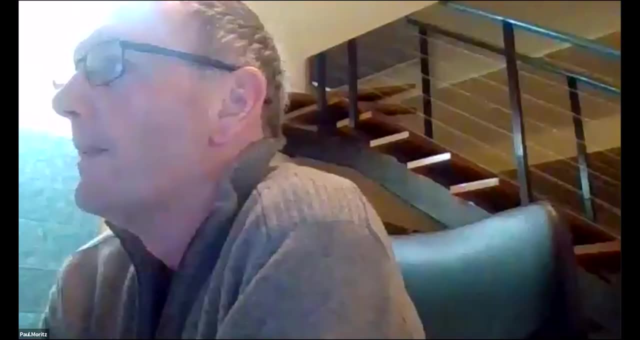 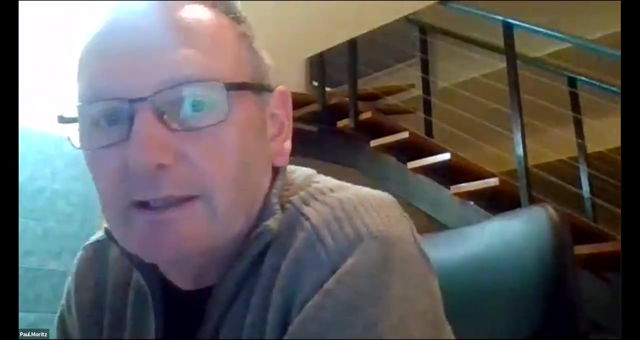 to go into this level of detail in a field that we've not done before. So thank you. Questions, anyone please? Hi, Ian, It's a question from Paul Moritz here. It's actually a two-part question for Susie. Can you hear me? 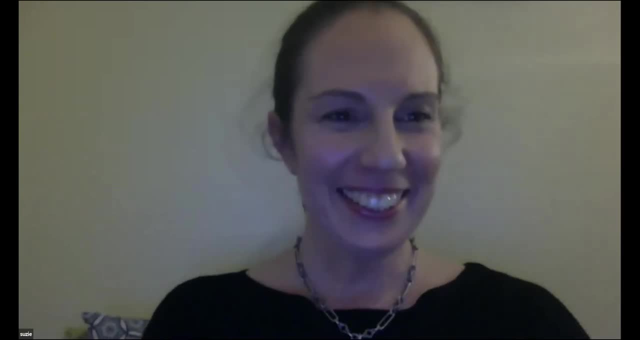 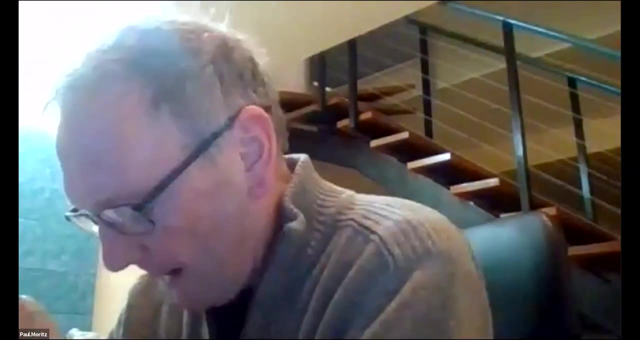 I can hear you, Paul. Yeah, Okay, Susie. first of all, the lead concentrations in soil that you've recorded. that seems to be a bit of a challenge. Yeah, Yeah, Yeah Yeah. That seems to fit a different distribution from what I would typically expect to see. 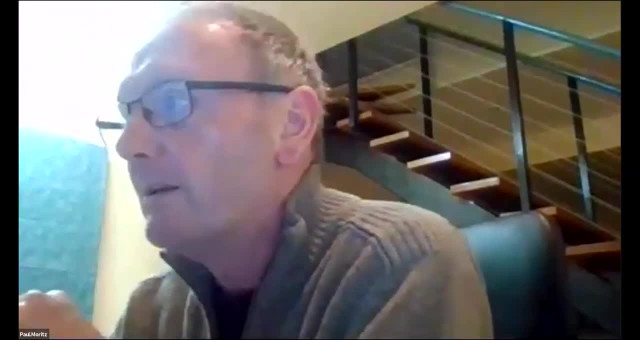 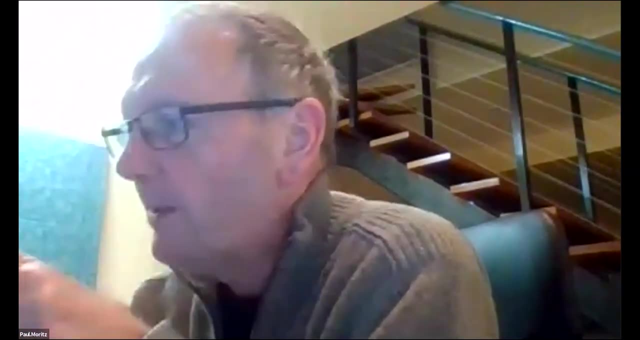 on a contaminated site that's being redeveloped in Melbourne. Admittedly, they tend to be focused in the inner north rather than the north and west, But I wonder whether anything could be correlated there with the fact that you've actually gone and looked at vegetable. 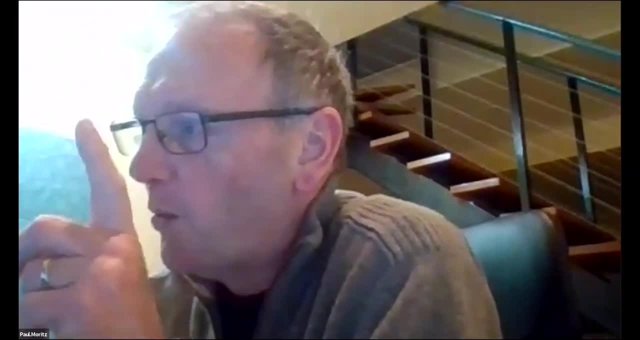 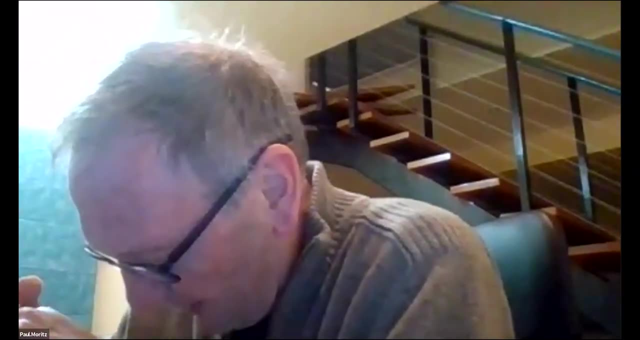 gardens. Could there be something in the fertilizer or the planting mix that people are using that's giving the higher lead concentration? That's my first question. Okay, Well, the second one's a comment. It seems as though the bio-accessibility you were showing. 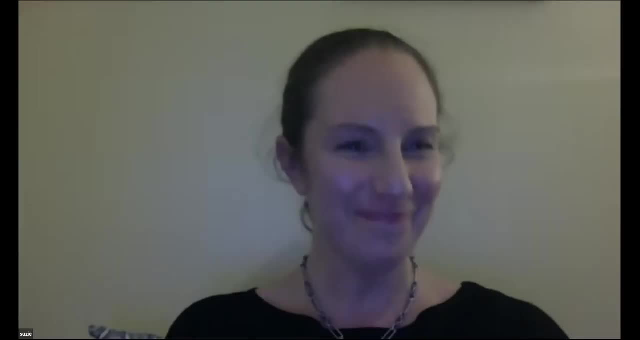 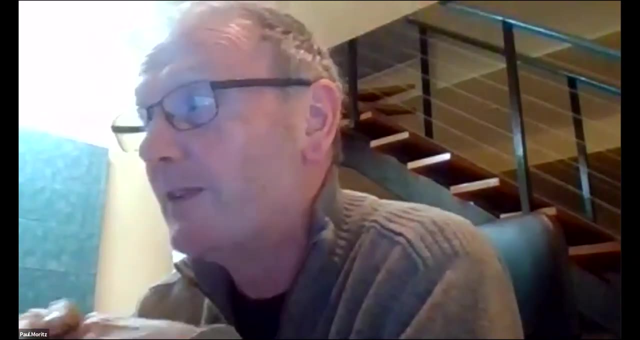 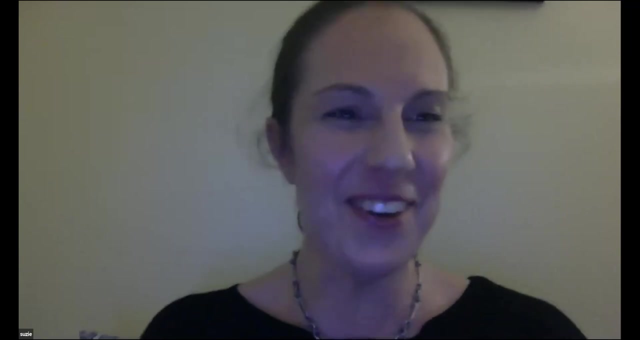 is pretty close to a hundred percent, which is interesting in the context of the health investigation levels you were talking about, which are based on an assumed bio-availability of 50%. Yeah, Okay, So I'm going to answer that one first, while it's still clear in our minds, 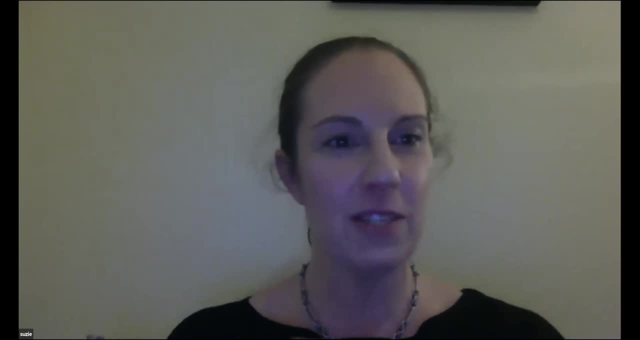 So I didn't talk about it. But part of the reason why I'm going to answer that one is part of the reason why we're doing this and part of the reason why ACLCA funded it was because that's the Australian Contaminated Land Consultants Association. for anyone who's 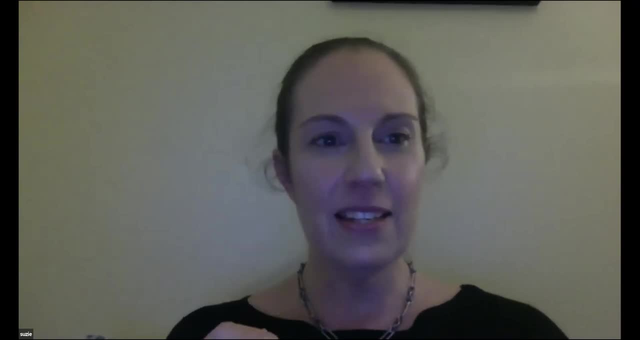 not aware. They were interested in getting some harder data around that. And, yeah, part of what we've shown and I'm a little bit hesitant to get people to go and use it, but it's basically you could probably just use your total soil concentration. 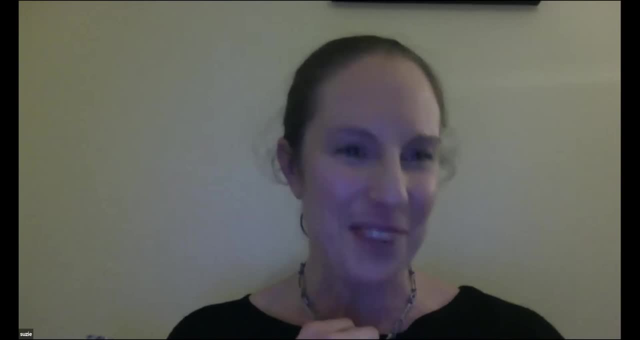 Okay As your bio-accessibility in the North and West of Melbourne. If we've got now again, this is in. yeah, this is not. it's been in vegetable gardens. So it's sites with legacy pollution And, from what we've shown, looking at a whole lot of different factors, it appears 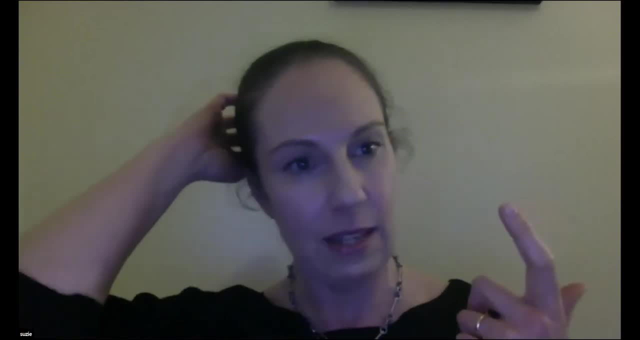 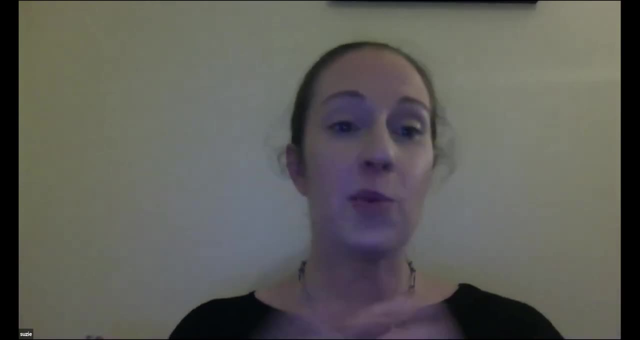 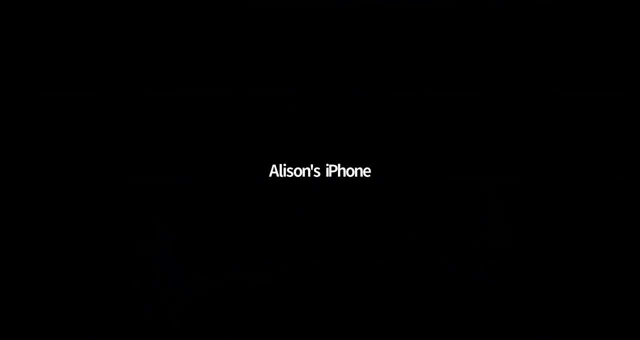 like it's mostly from lead and paint and lead leaded petrol. Not only in a few situations. was that actually industrial pollution? Yeah, So whether or not this holds in real brownfield sites with sort of lower organic matter, lower, yeah lower- levels of fertiliser, we get some really high organic matter in. 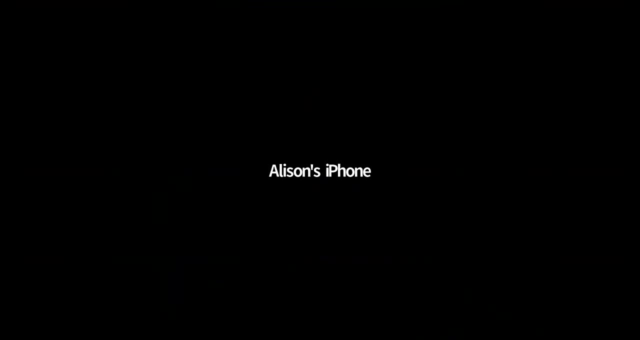 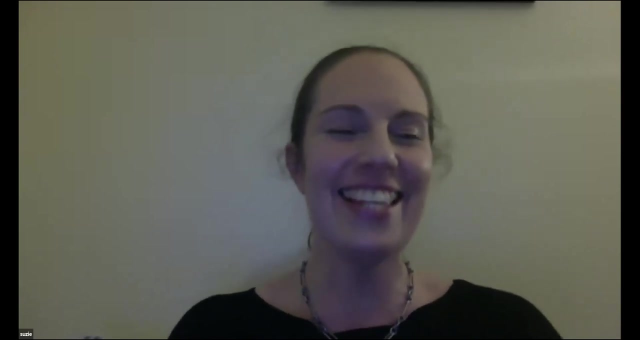 some of those sites. We've actually had trouble. Alison, could I ask you to mute? sorry, that's all right. I think it's happening. It's happened to all of us over the last few weeks, Thank you. Yeah, we get really high organic matter concentrations, which might be quite 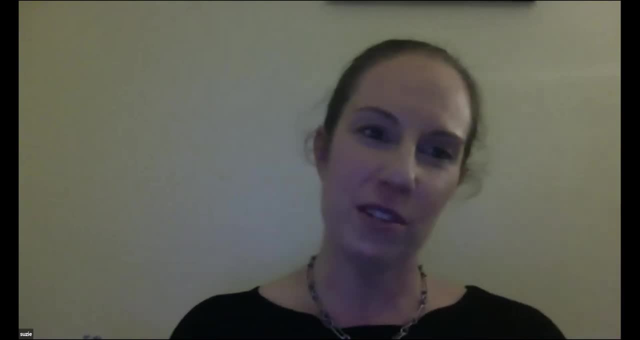 different to in more brownfield sites. So this research, I think, is really interesting from the point of view of assessing more brownfield sites, but we're not exactly sure how transferable it is yet. Now, Paul, could you please repeat your first question again? 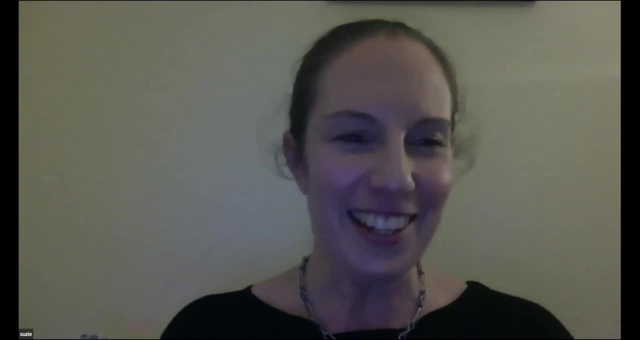 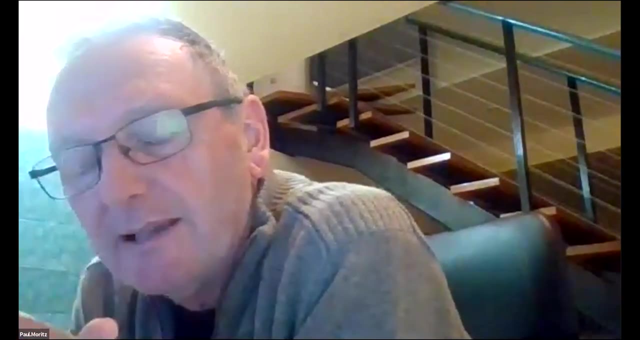 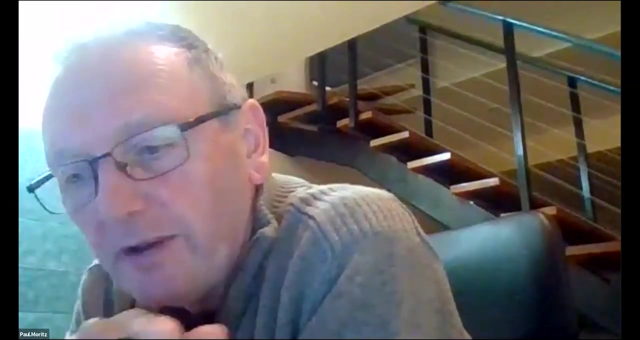 Or just remind me so that I can get back to it. Yes, The distribution of lead concentrations that you were showing there shows more high concentrations, particularly above the health investigation level, than what, in my experience, you typically see on a brownfield site. So I was just wondering whether that and brownfield. 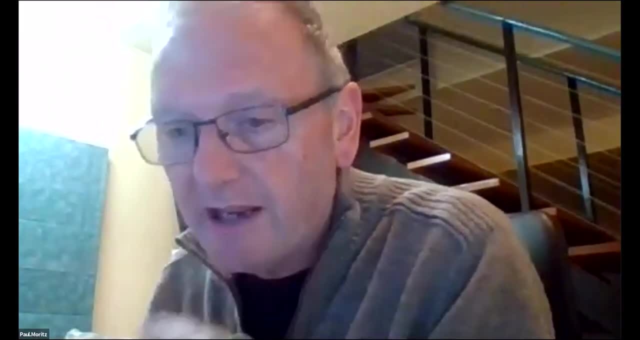 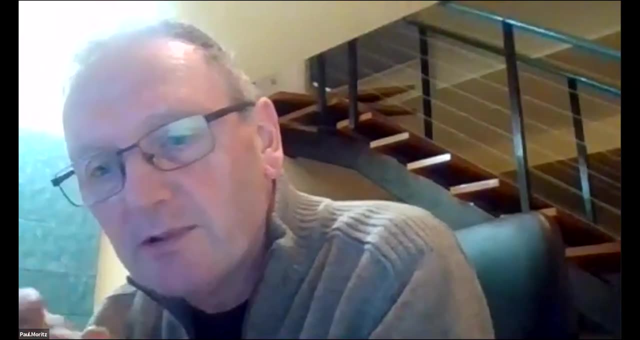 sites can be near major roads and in the suburbs, So I was just wondering whether it might be linked to the fact that where you've taken your samples have actually been used for cultivating vegetables, and something that's been added to the soil there might be contributing. 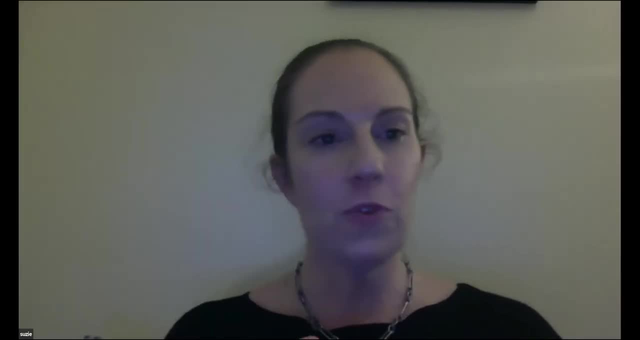 Yeah, So research. so from the Veggie Safe Paul Taylor's data that we also published, then the data from it, from Melbourne it looks like they get, and in the paper in Melbourne too It's a relationship that soil that's collected under the eaves. they call that in the drip. 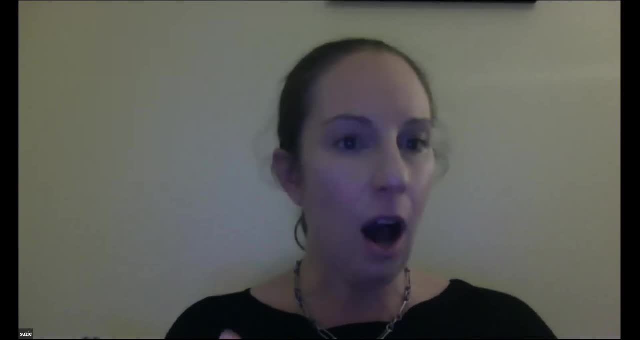 line. It is very high. It's higher than the soil collected in the veggie gardens, So we're fairly confident that it's coming from paint and or or like sort of from the leaded petrol that's collected on roofs and then, over the years, drifted off. Yeah, Did you want to add? 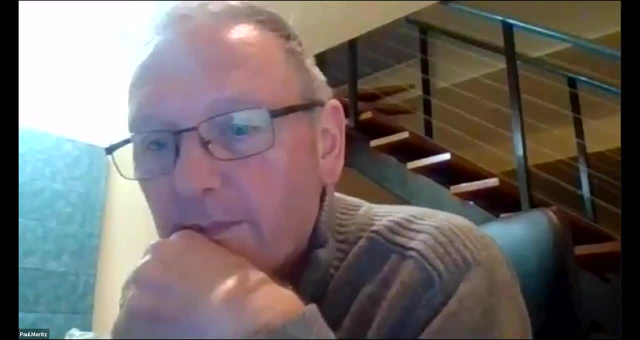 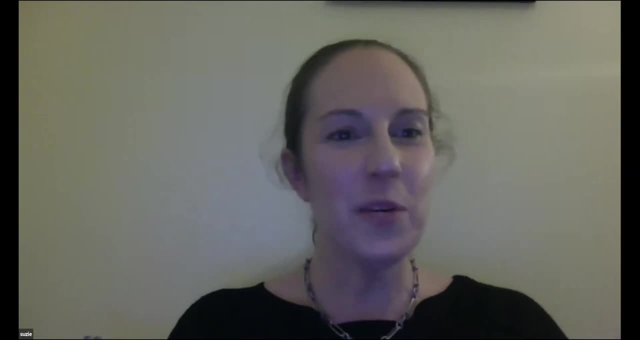 something there, Paul Taylor. Well, the other thing about drip lines that we've done then is that particularly older gathering lead solder would have been: Yeah, Yep, Yep, Lead solder, Yeah. So we and Slavica did some principal components. 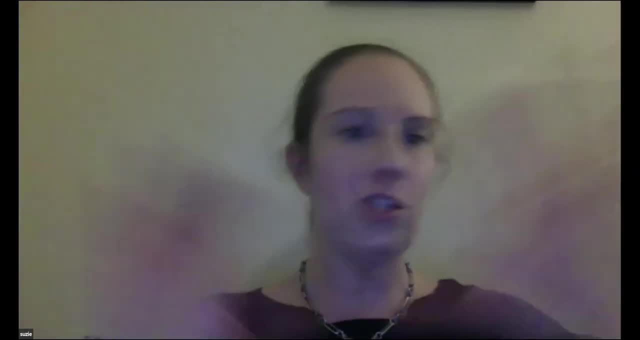 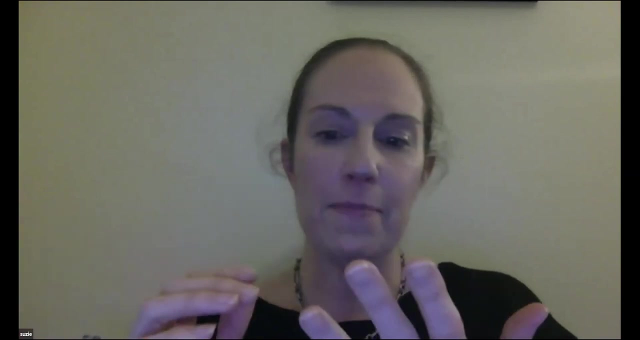 analysis just to get an idea of what was varying with what, because she measured all sorts of different things, you know, iron or soil, organic matter, And I didn't show that data tonight but lead the lead really clearly came out with the age of the house and the distance to the road It didn't connect with. 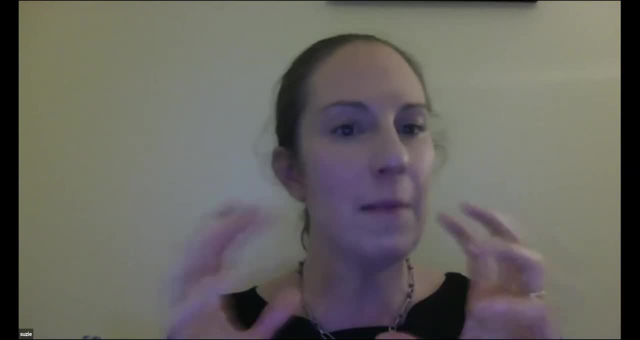 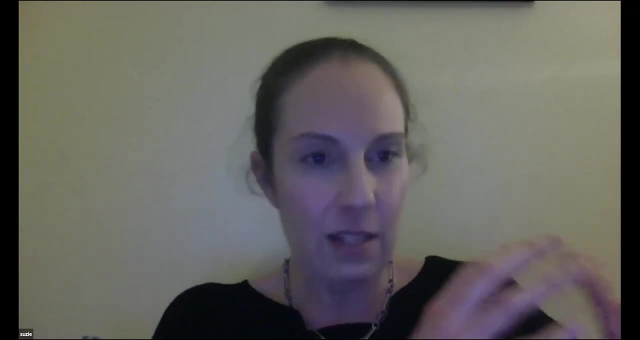 like distance to railways or- and it didn't come out with any of the natural sort of soil things like pH or cation exchange or any of those factors, Whereas chromium and nickel all came out in the PCA connected to those natural soil factors and they weren't related. 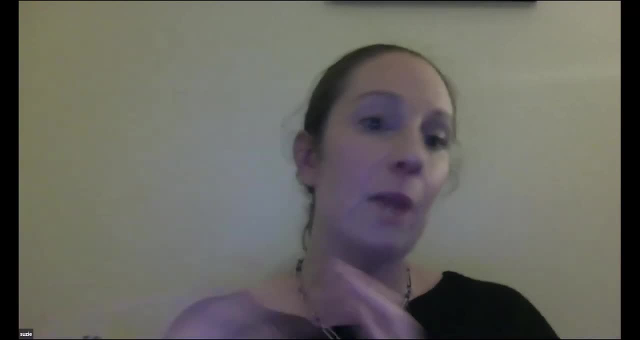 So I mean we didn't look at that. I mean we didn't look at everything We didn't have included in there, like proximity to industry, say. but we're able to explain so much by those correlations with things like house age, And I didn't show like whether the house is painted or not was had a very 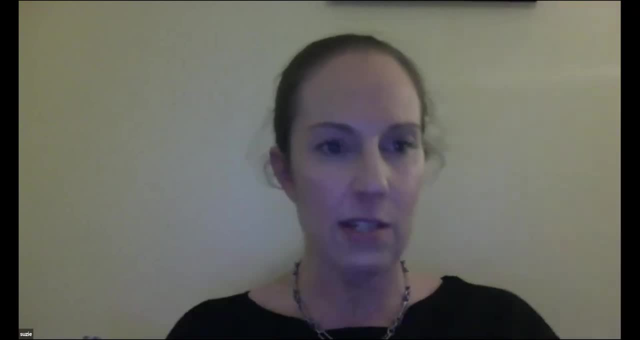 big difference on the concentration, irrespective of the age and things. So we're we're fairly confident you know as much as you can be with correlations, rather than you know directly looking at it. We haven't done any isotopic work or anything like that, Although I am. 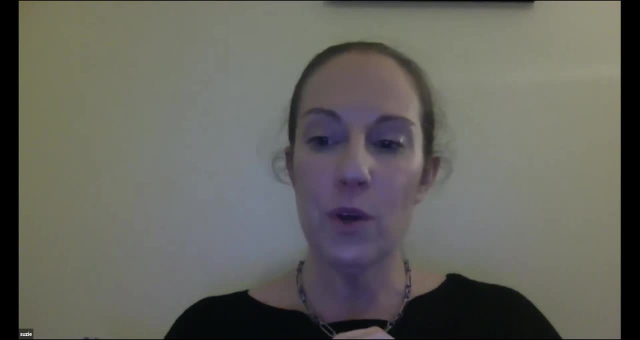 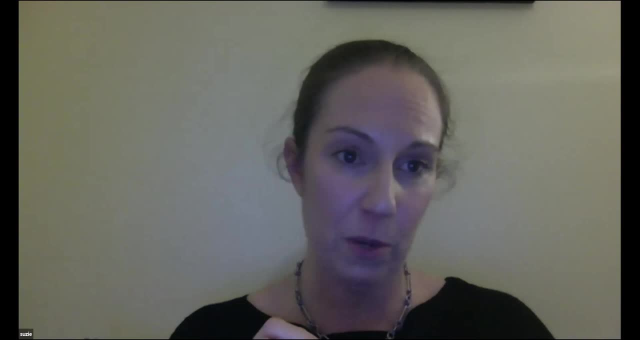 it to Sylvica's project where we are starting to do some of that isotopic work to try and ascertain, you know, bit more confidently than using correlations to look at where it's coming from. So you know, kind of watch this space, I guess. 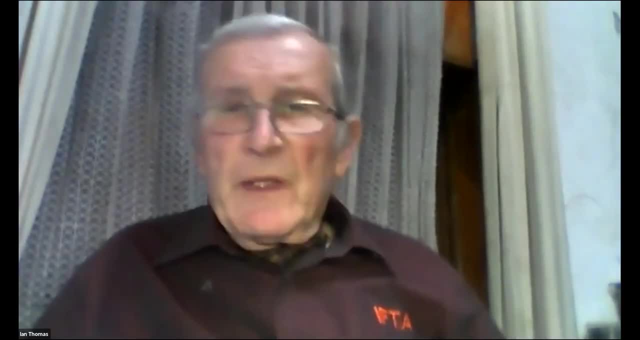 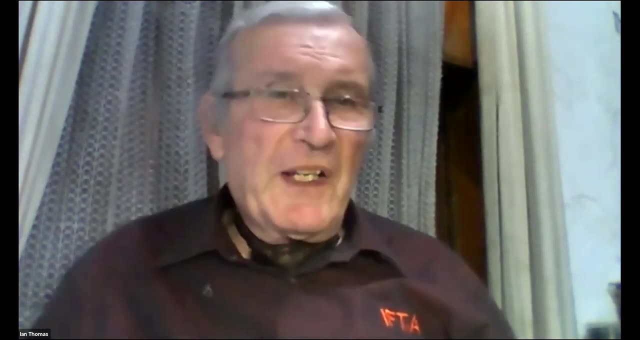 David Sheldon. Could I come in at that point, Susie? I just. obviously other questions would be welcome. as far as I'm concerned, Technically we have one minute left, But provided you're all happy to go a little longer, I certainly am. 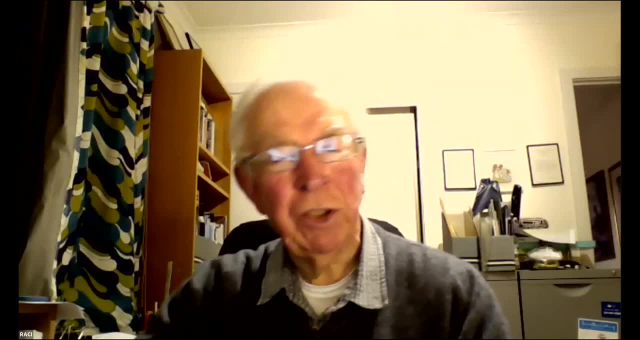 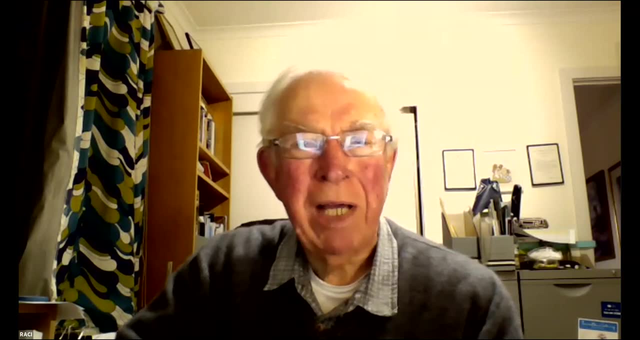 I think that would be a good idea, Ian, But what I should have mentioned is that Phil Sinclair had his hand up during Susie's presentation. I don't know if he wants to make a comment at this juncture. Do you want to say anything? 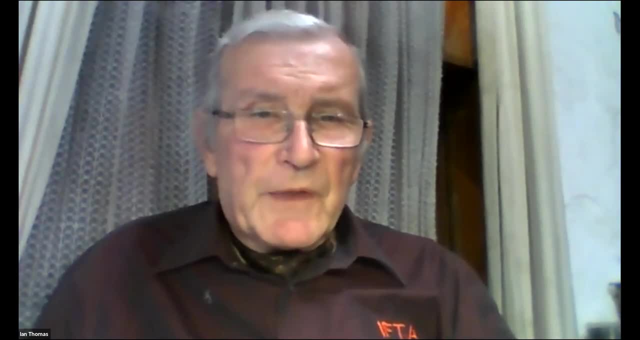 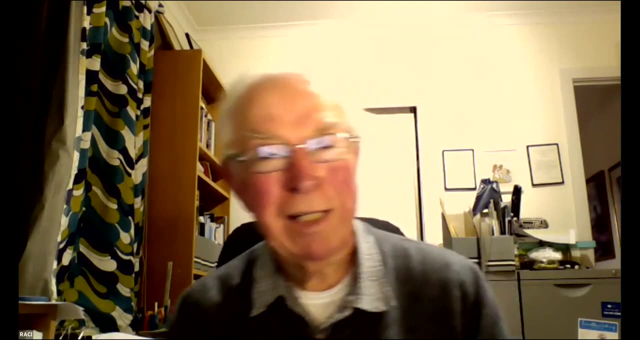 I can't see Phil on the air. He's further on, I think. Well, he might have left by now, so I'm sorry. I apologise to Phil for not sort of recognising that he had his hand up during the meeting and during Susie's presentation and perhaps had something to say. 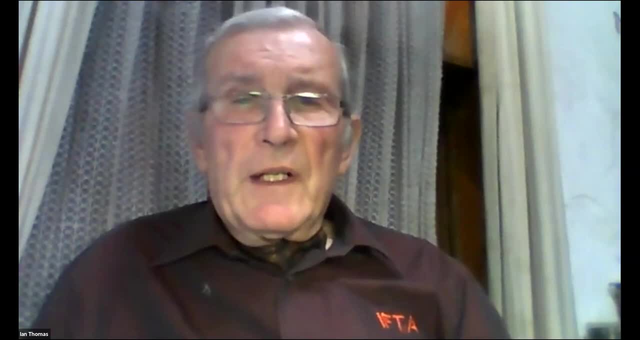 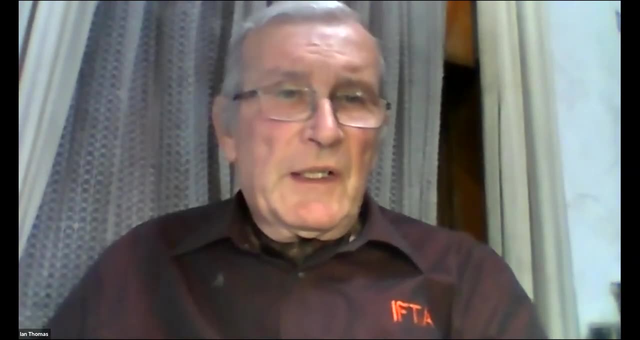 But if he's gone, he's gone, Okay. Okay, Incidentally, before we go, I'm going to mention something about Brad Clark, who's our next presenter, and what he's up to, But first, are there any more questions from anybody? 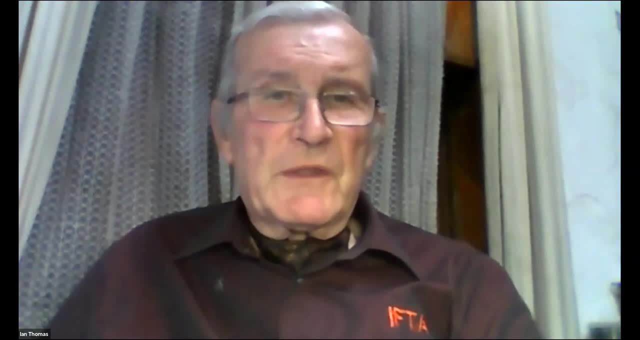 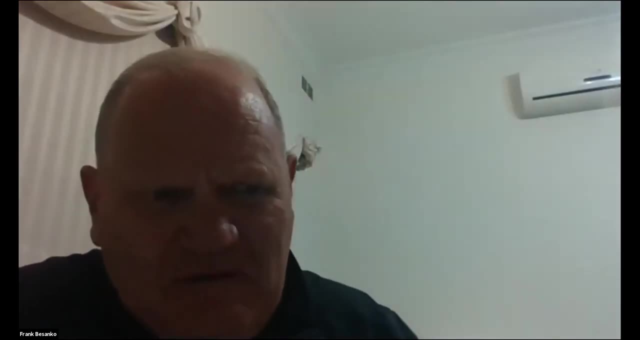 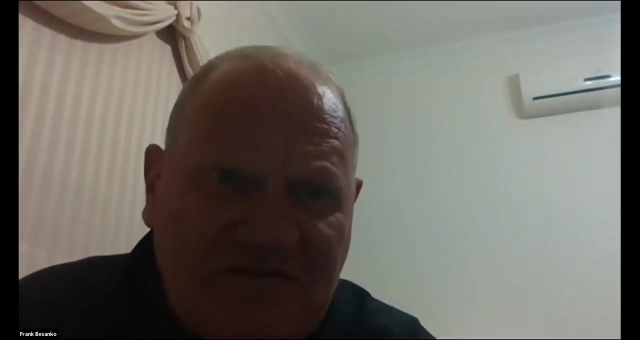 And good for you. Thank you all for chatting as well. That was good. Frank Bissanko, Firebreaker. I've got two questions. Go, Frank Good man. First question to Susie: The electron microscope that you used in your testing of some of your materials. 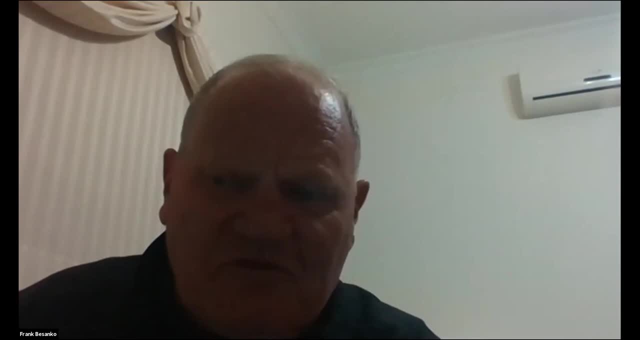 what time frame was there when you dropped off the sample to when the results were delivered? Do you mean the synchrotron, the XAS? Yeah, sorry, Yeah, Oh goodness, I can't remember that off the top of my head. 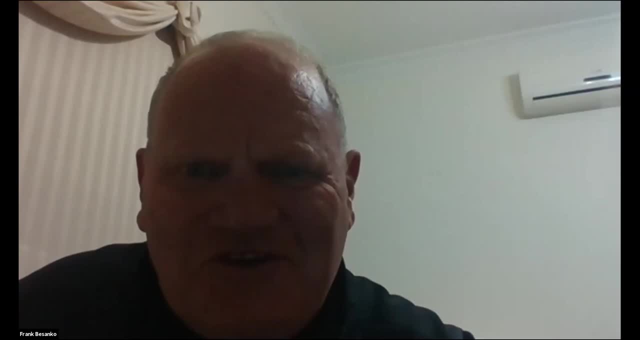 Sorry, The second question. look, I'm not a chemist or an engineer, but just a firefighter. But just for my, it might not be the appropriate place to ask this question, but the soil testing on the Westgate Bridge site- where did that go wrong with the companies? 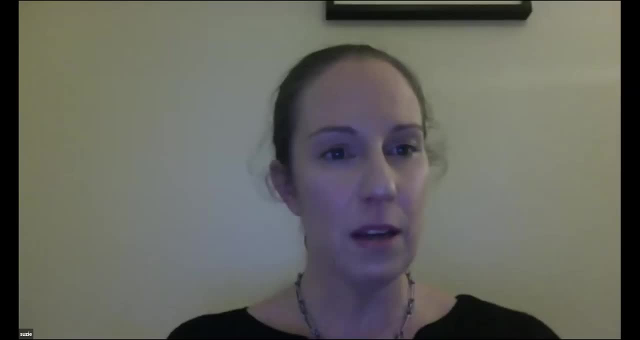 Have you got any insight into that? or rough? Do you mean the PFAS testing and the tunnel? Yeah, the soil testing? yeah, Look, I've sort of been like I only really know what's in the press for it. 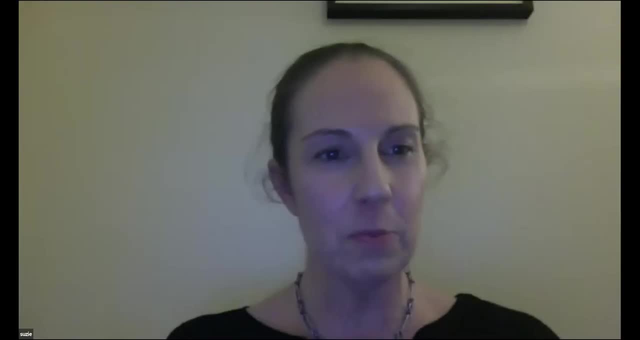 I've sort of been following it a little bit, but I think the thing with PFAS is we're finding it in all sorts of places, We used it in all sorts of things and it's really soluble and mobile And so you know, it moves through the soil. 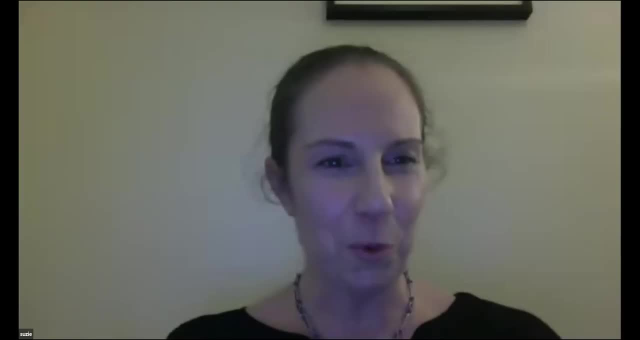 Okay, And yeah, I think I don't know that's a very broad kind of answer. I hope that helps a little bit. Probably a dumb question for this forum actually. Well, no, I don't. I mean it's in the broader area. 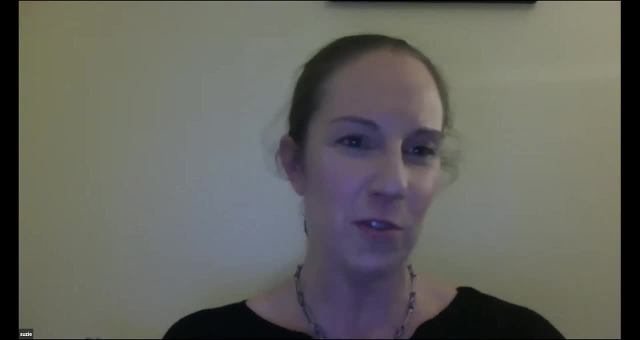 I'm just not. I don't happen to be involved at all, haven't been involved at all in that project. Not a dumb question, just slightly outside our expertise. Well, no, it's just that I haven't been involved in that project, I think. 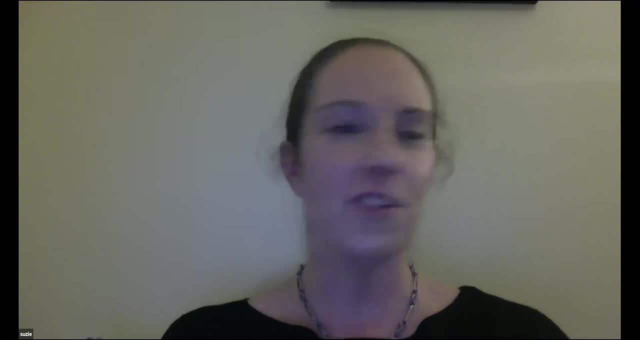 But you know, sometimes, if it's, you know, there's certain contaminated land assessment ones that if you talk to me about, I'd be able to talk more generally about them, but just not that one, unfortunately. Okay, Thank you. 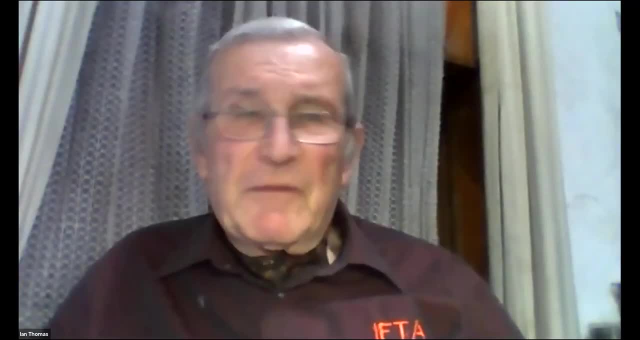 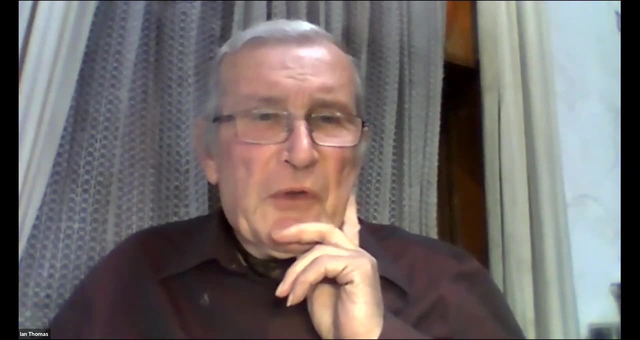 And it's. I've got to say it's a terrific lead-in for Brad Clarke, who's going to be our next presenter on the 18th of July. But before I do that, if I'd been with it at the beginning of this. 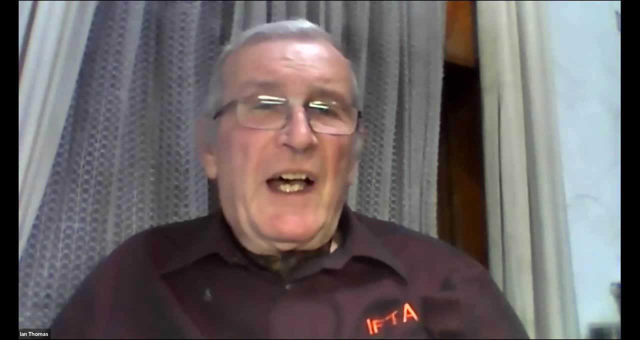 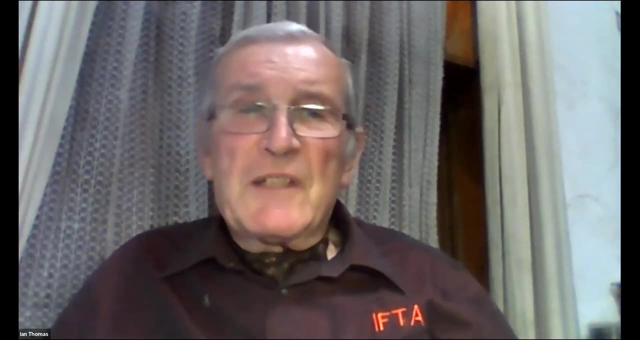 I would have said thank you to Richard for organising this meeting And Brad Clarke's, because it all started back in February at our last face-to-face meeting, when I said: I'm quite happy to continue as chair, but I don't want to also organise the seminar. 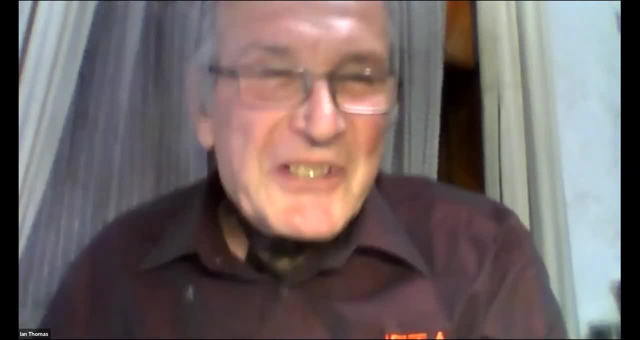 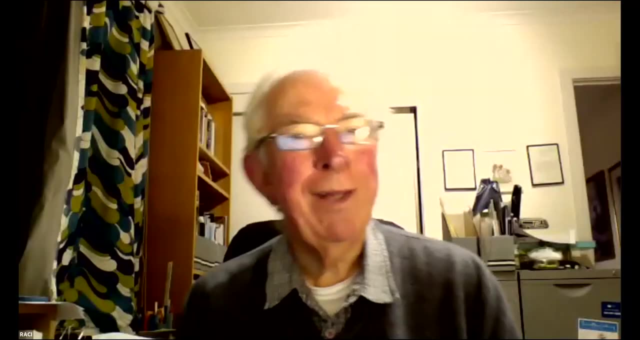 Is there anyone who'd like to do it? And I kept pressuring Richard and he bit the bullet brilliantly. So thank you, Richard. Thank you Ian. can I just say something that Brad Clarke is talking on the 18th of June, not 18th of June. 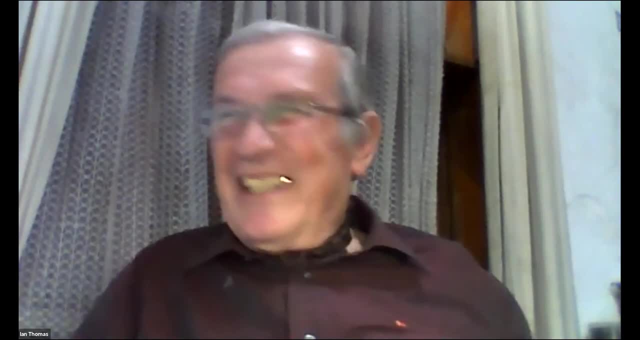 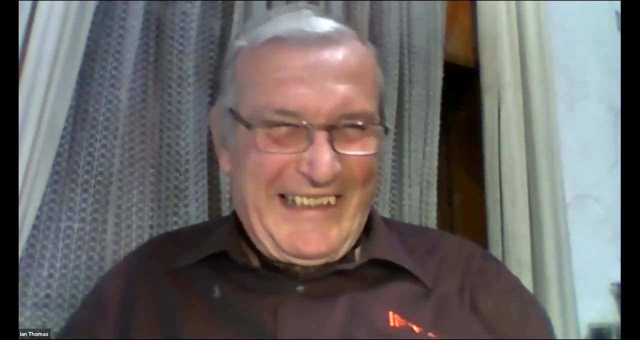 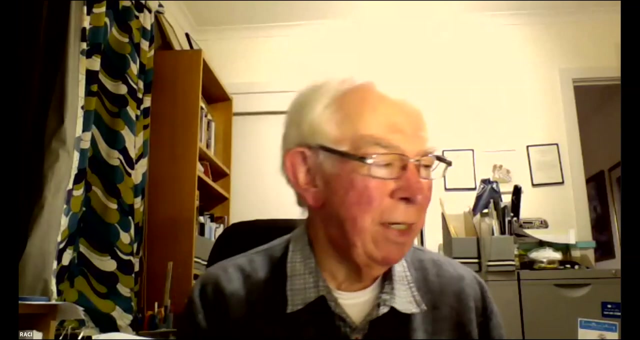 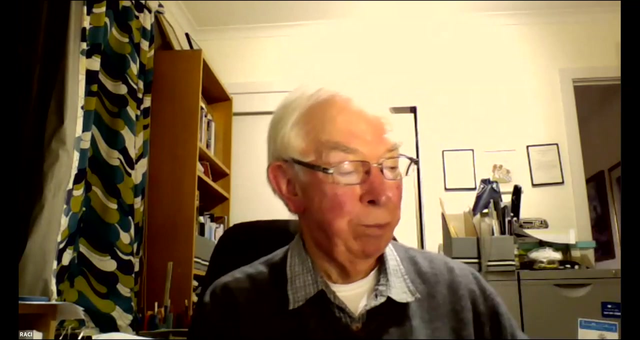 I beg your pardon. Indeed, I've got it written here. I've got two mice open. you see, Is it two mouses? I'd like to also mention, if I can, that Brad is organising a series, a weekly series of seminars, starting next week, on environmental pollutants and so on. 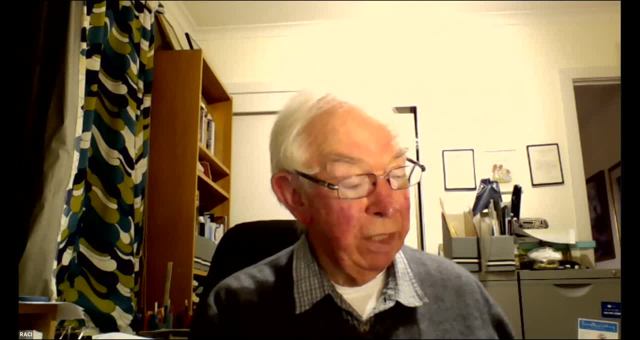 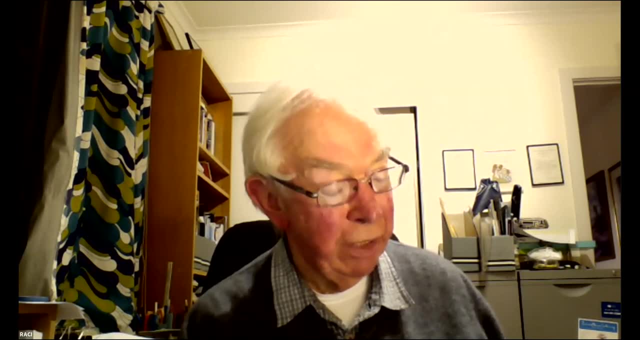 I think the first, the first presenter, if I've got it here- and I think I've got it here and I've lost it- It's the environmental science meeting for Australian research teams, Envi-SMART or Envi-SMART. 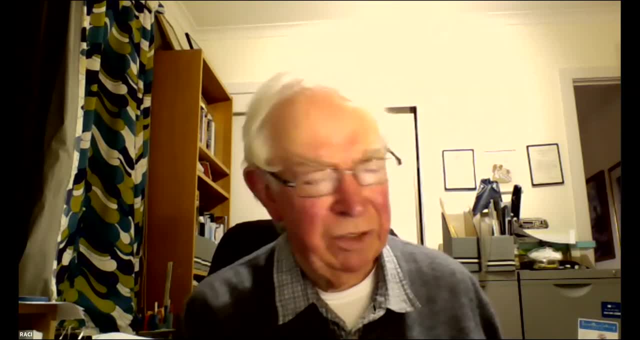 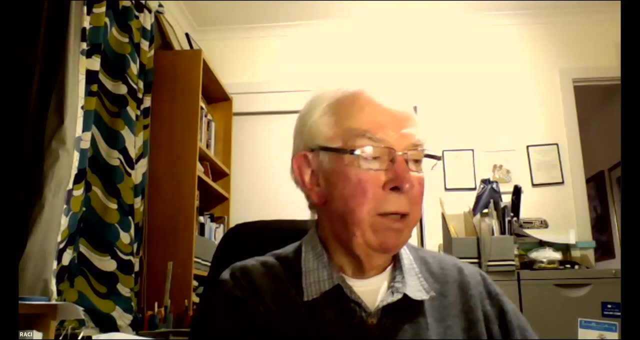 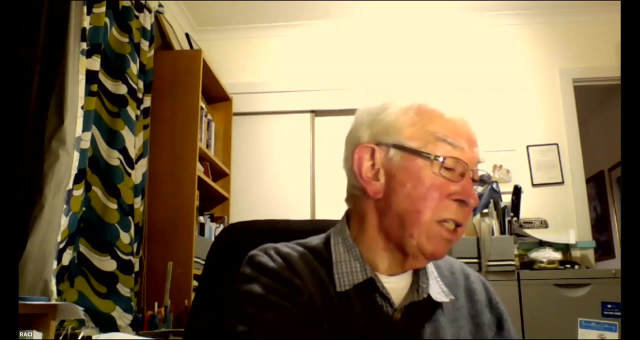 The first presenter is going to be Bob Wong next Thursday from Monash University. You can find out more details on Brad's website at the University of Melbourne. And I have got it somewhere and I've lost it So, So that's not very efficient of me. 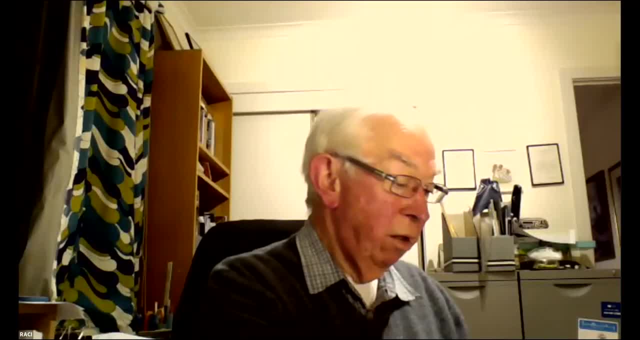 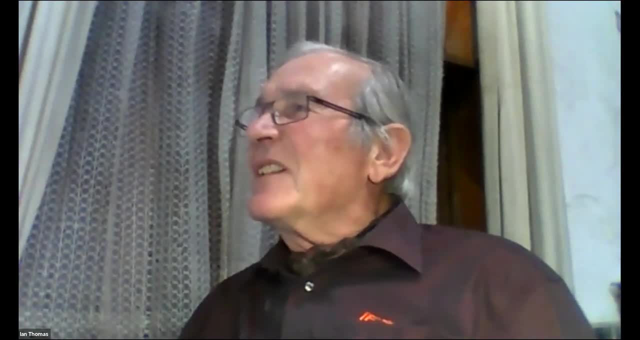 I've got it here, Richard. You've got it there, have you, OK? Yeah? Yeah, I call it Enviro-SMART, even though it's Envi-SMART as written, because the S-M-A-R-T stands for things. 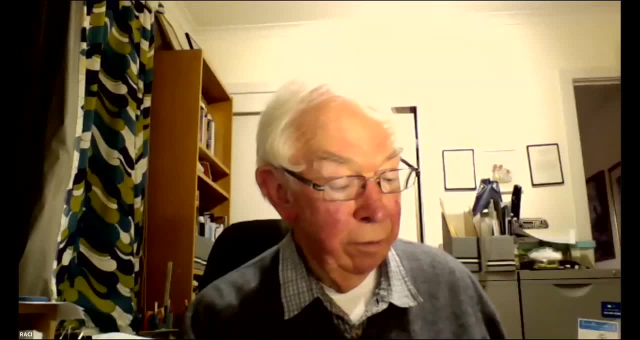 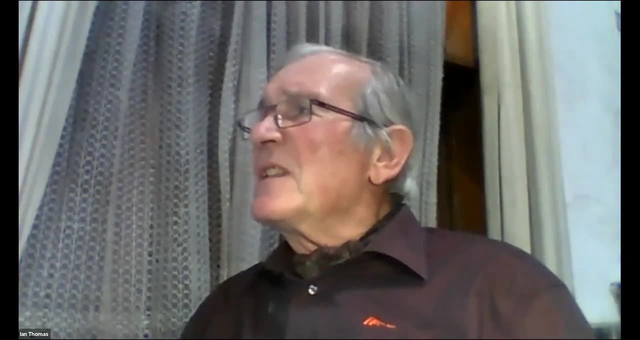 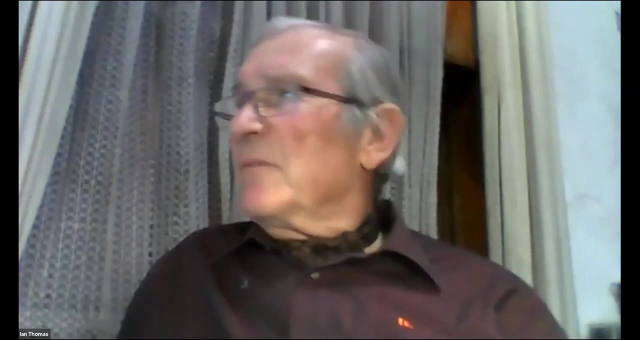 So it's Envi-SMART as written. Yeah, So the site that I've got is Envi-SMART. underscore: abstract hyphen, submission hyphen- April 2020 dot PDF, Something like that. But look up, look up Melbourne University and ask for Brad Clark and that'll do it, I'm sure. 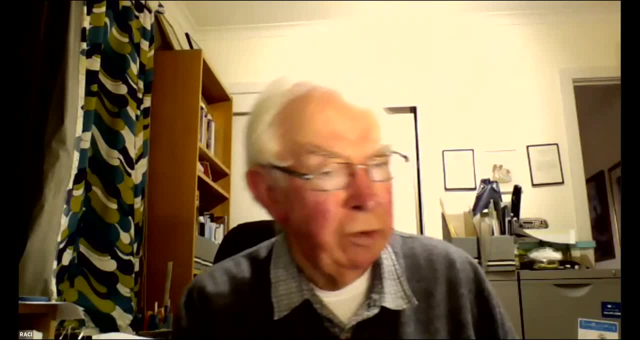 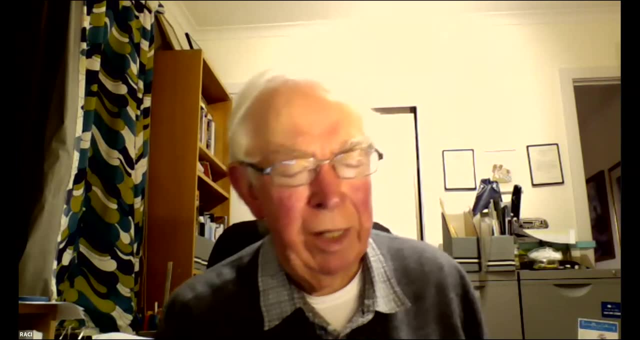 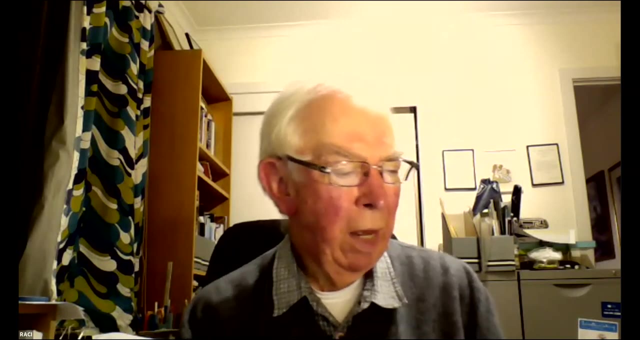 I'm sure it will. Brad is looking for student abstracts to be able to be involved in the participation in the seminars And I believe there's going to be quite a generous prize for winning students. So it will be interesting. starting next Thursday on a weekly basis, I think five o'clock. 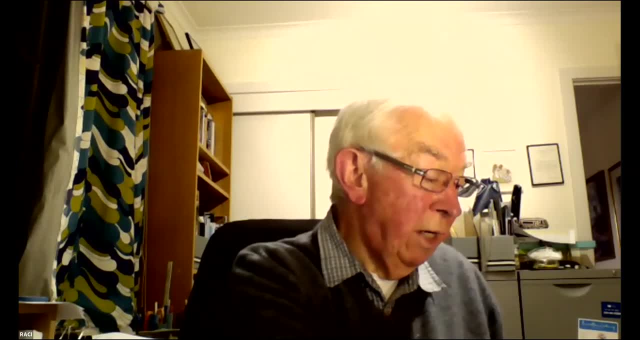 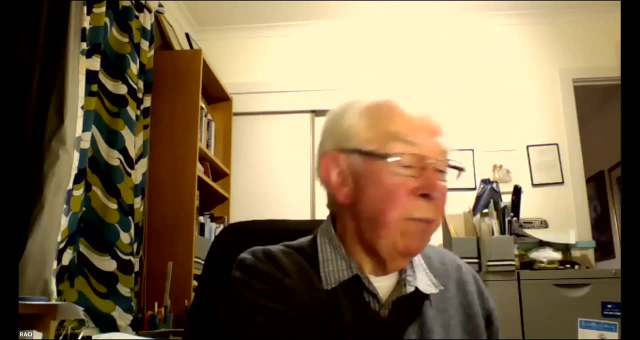 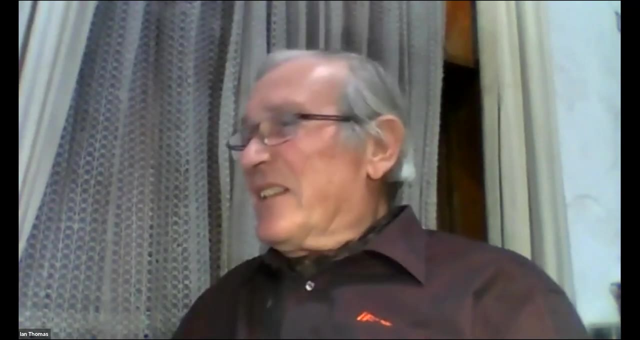 And He will be, as you said, Ian, speaking at our next HS&E seminar on the 18th of June, June, June, Right? The other thing I wanted to mention about that, which is it fascinates me. 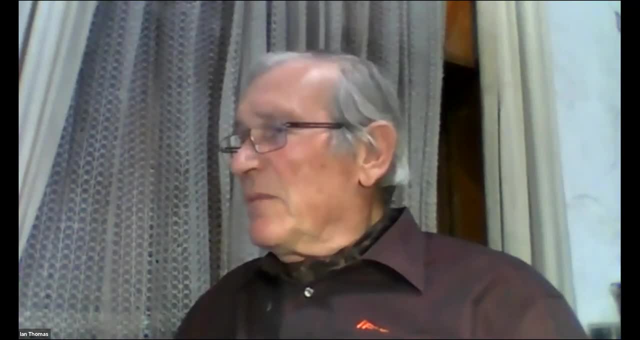 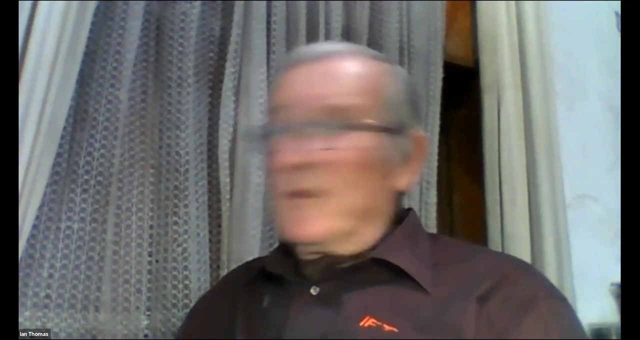 We know Brad Clark. Dr Brad Clark is Melbourne University, but he's also has Agilent and Eurofins involved in this as major sponsors- Yeah, Which is delightful. And at the bottom of his website it lists RACI, of course, which is us lot, and Accolcut and various other organisations that are partners. 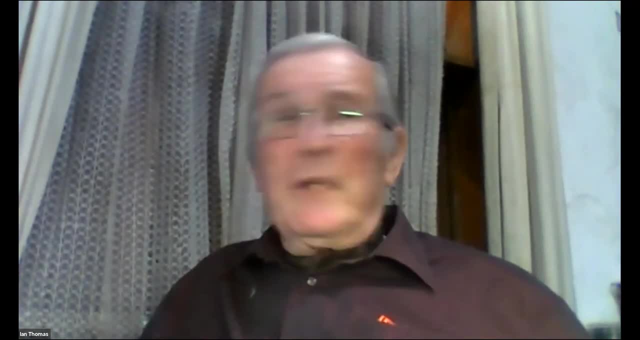 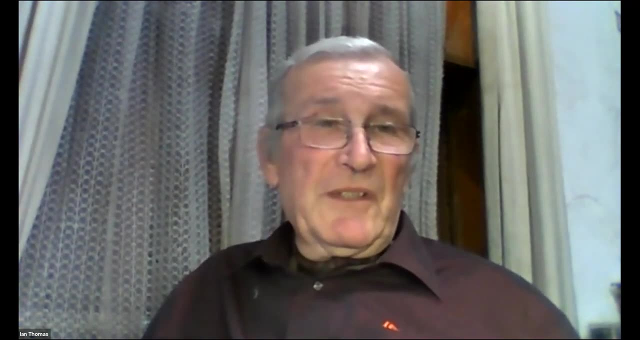 So it's quite delightful We're learning more now that the COVID-19 is on than we otherwise would. My goodness, Right now is there a last question from anyone for us? No, No, No, No, No, No. 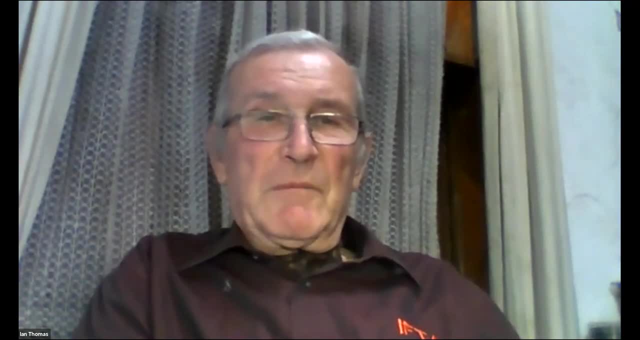 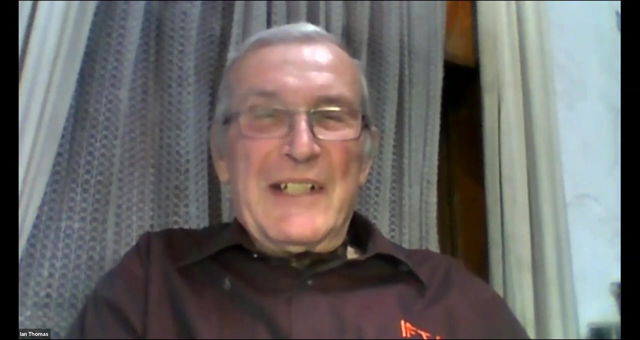 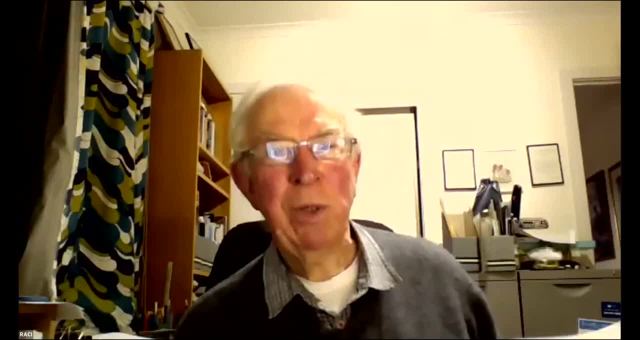 Thank you again, then, Susie, June June, June, June, June, June June は. Jeyueyn. Jeyueyn For Thomas. Jeyuey examples: Jeyueyn Justyne. 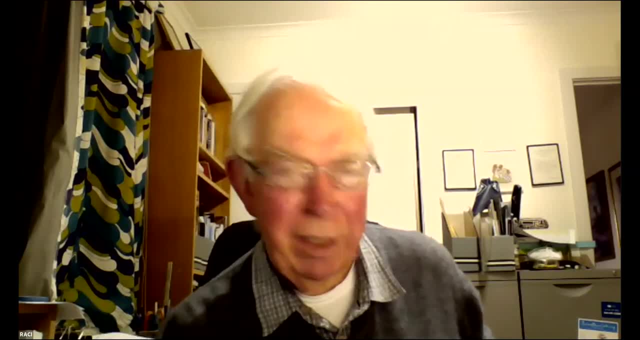 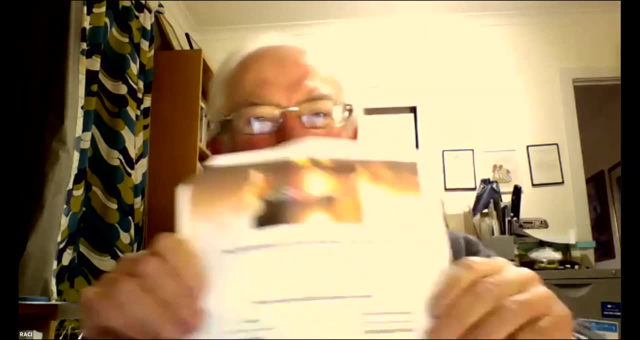 Thank you very much And let's all clap. Thank you, Thanks. Well, we can do that virtually. That sounds good. At this stage in the proceedings, we would normally have produced the video showing, just a corner, a bottle of wine each for our speakers, but clearly we can't do that, so you will get a gift card like: 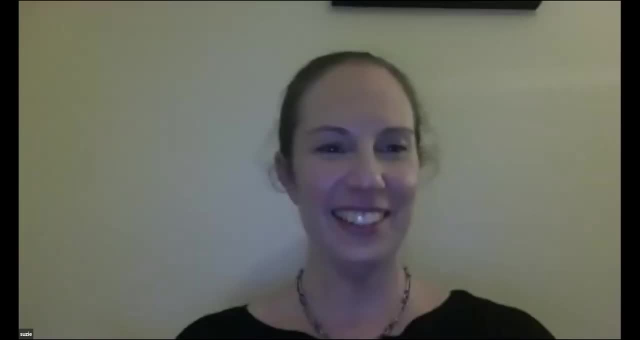 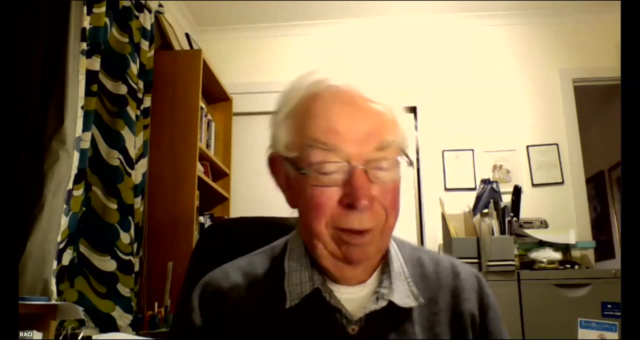 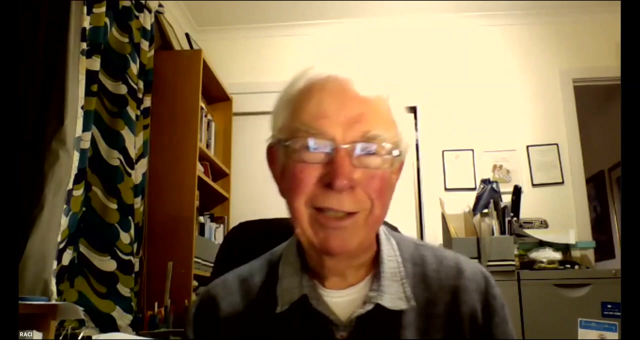 that sent to you by email, and so it's the best we can do in the circumstances. the advantage is that you can spend the gift card on grog, if you want to, but also on other things at walrus or big w or caltex or wherever. so a bit more flexibility. but thank you again, uh suzy and uh jewin. 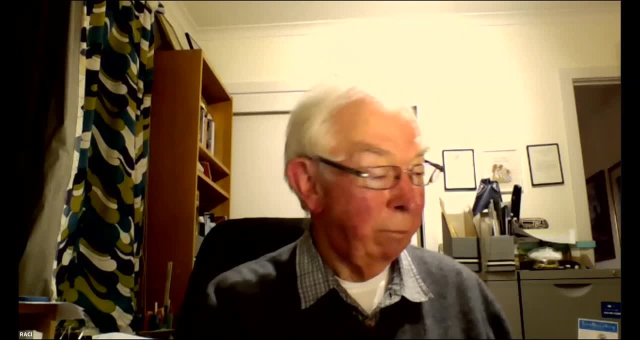 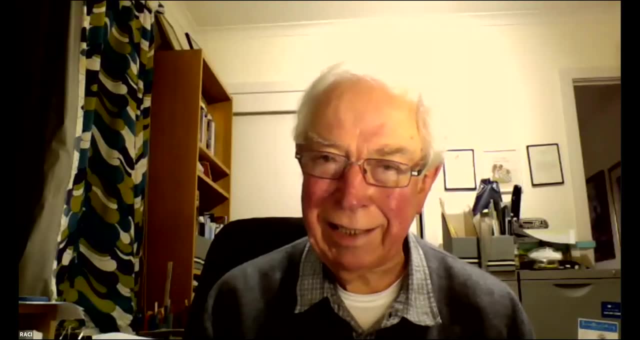 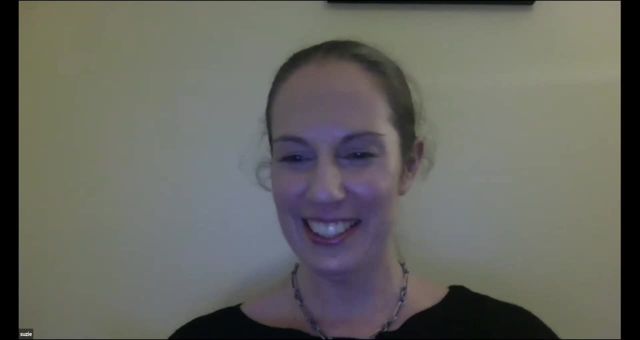 jewin and- um, i forgot your name, um, justin, justin. yes, absolutely uh, jewin and justin for an absolutely fantastic uh evening, thank you, thanks for having us. yeah, thank you very much, and you now wish to close, richard, because we can. sometimes we kick on a little bit informally afterwards, but